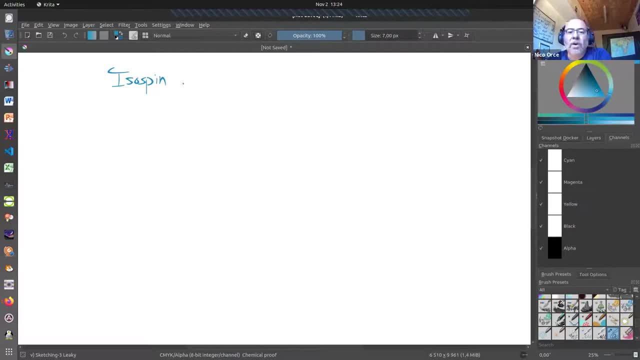 in our lecture notes, Or what is the same thing, is the charge independence. it's also called independence of nature And the nuclear. So basically, this implies that we're going to be treating protons and neutrons as the same particle, independent of the charge that the proton has. We're going to be calling 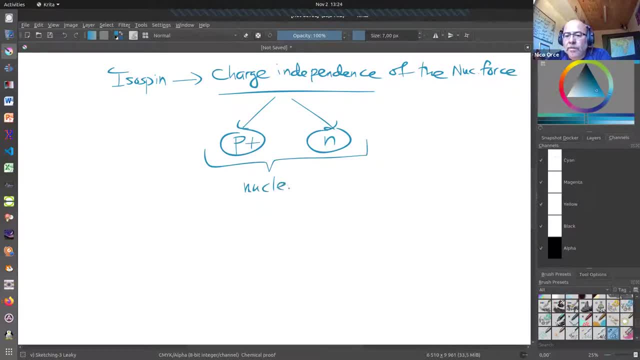 these two guys Nucleons Right, And this was an idea, An idea introducing in 1932 by Heisenberg, the guy of the Uncertainty Principle right. And it was introduced by Heisenberg because it turns out that during 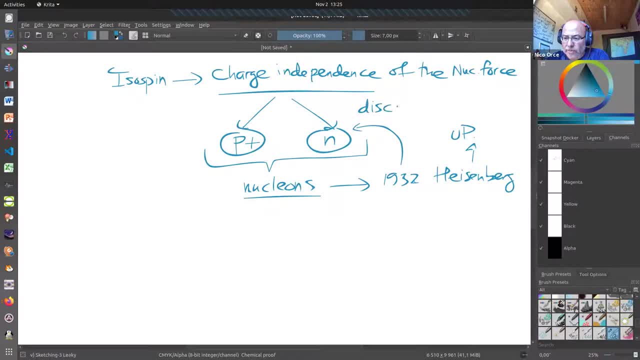 that same year there was a discovery of the neutron. Discovery of the neutron happened in 1932. I'm sorry, the neutron. And to treat things to be simple, to apply simple mathematics, to treat the problem always in a simpler way. it was an interesting notion to assume that. 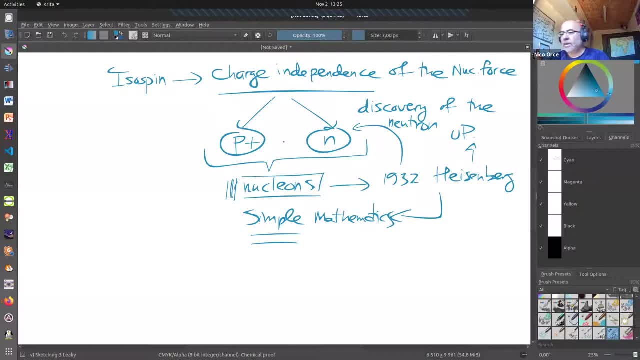 proton and neutrons were exactly the same particle, always assuming that there's a charge independence of the nuclear force. But we know this is not a pure symmetry. Sometimes isospenes is called isospenes symmetry But it's not a pure symmetry because, as we know, it's broken by the Coulomb force, right. 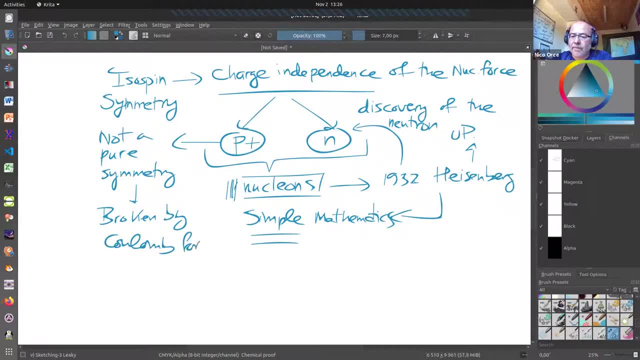 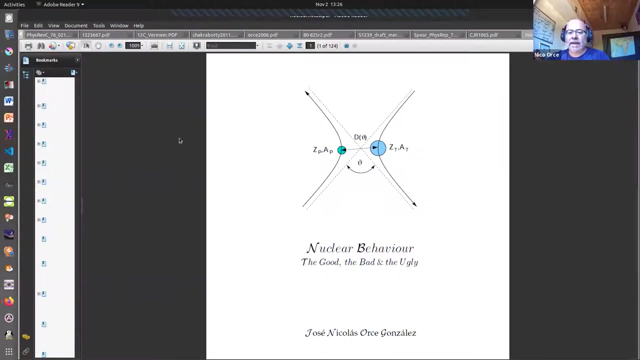 Broken by the Coulomb force. So it's not a pure symmetry. What we call it is approximate symmetry, Approximate symmetry. But it's going to simplify mathematics. It's going to make a very interesting insight into nuclear physics. Here we are going to get into it. 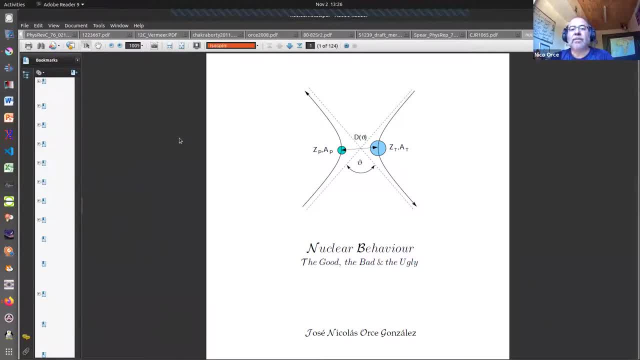 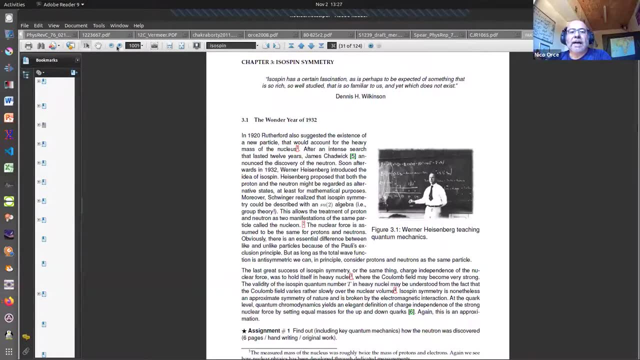 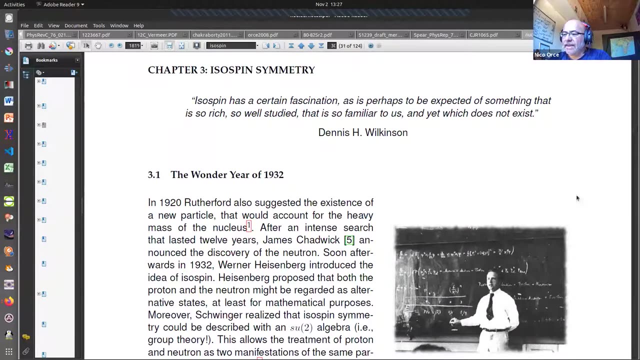 By going to the chapter, the isospenes chapter, which is chapter three. isospenes, symmetry, Right. So, as I was saying, the idea of isospenes is not a real thing, It's something, something fictitious. you know, is a mathematical approximation to treat proton and 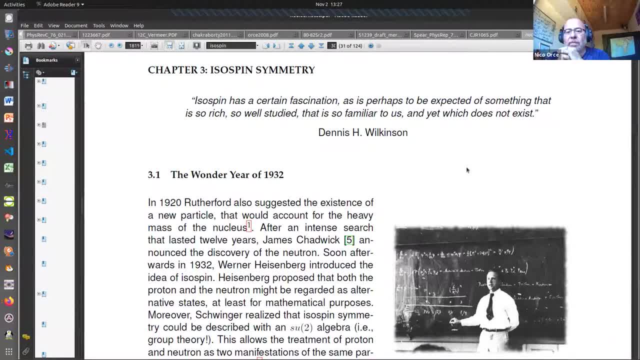 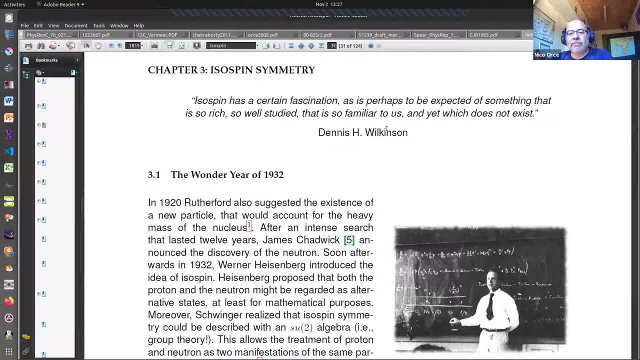 Bye-bye. as Sir Dennis Wilkinson wrote in his book which I have here- This book is probably also in the library- It would be nice to get a thick book. You see, here we go. The editor is this guy, Wilkinson. 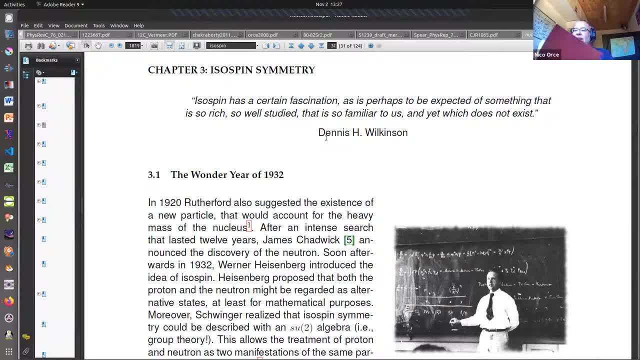 He says he's been in nuclear physics. As you can see, this is signed by the same person, by the same Sir Dennis Wilkinson. with regards to every encouragement, Dennis Wilkinson. So this guy wrote down that. I suspect he has a certain fascination, as is perhaps to be expected. 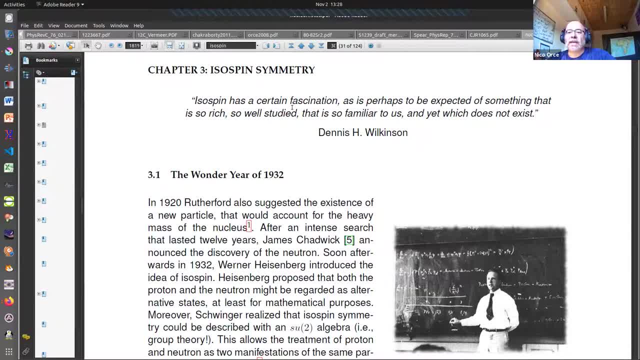 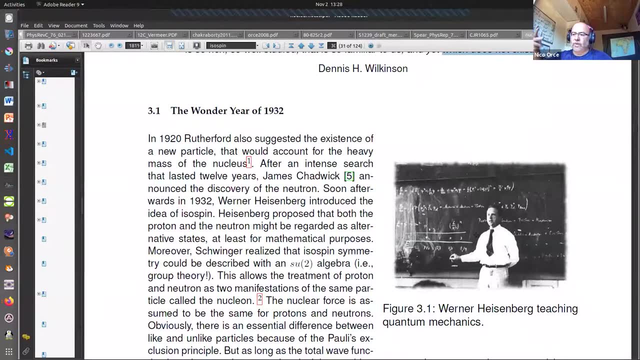 of something that is so rich, so well studied, that is so familiar to us and yet which does not exist right. This mathematical approximation, as I say, was introduced by Heisenberg using the opportunity that the neutron was just discovered in 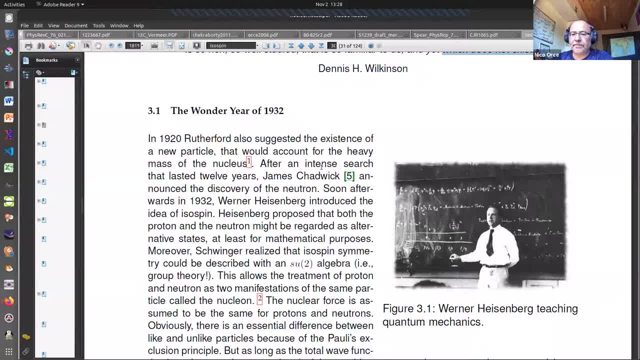 1932 by James Chadwick, And in the lecture notes you have different references where you can go and check. So Werner Heisenberg introduced the idea of isospin, proposed that both the proton and the neutron might be regarded as arthritic. So Werner Heisenberg introduced the idea of isospin, proposed that both the proton and the neutron might be regarded as arthritic. So Werner Heisenberg introduced the idea of isospin, proposed that both the proton and the neutron might be regarded as Cowden. 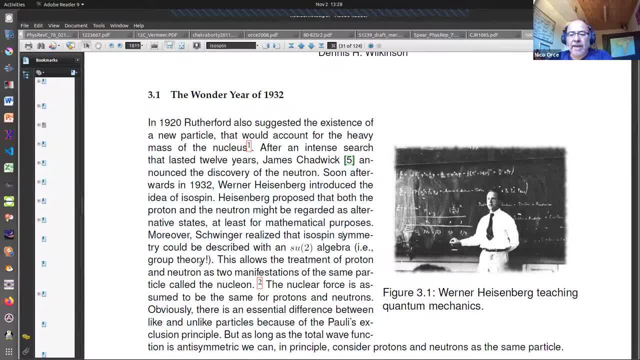 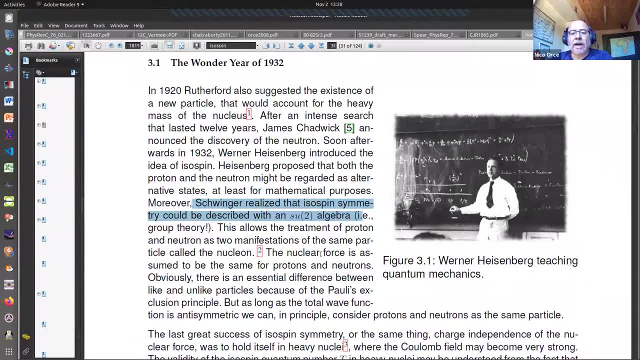 or at least for mathematical purposes. And then Schwinghere realized that isospin symmetry could be described by a particular algebra in group theory, And this allowed the temptation that protons and neutrons has two manifestations of the same particle called the neutron. 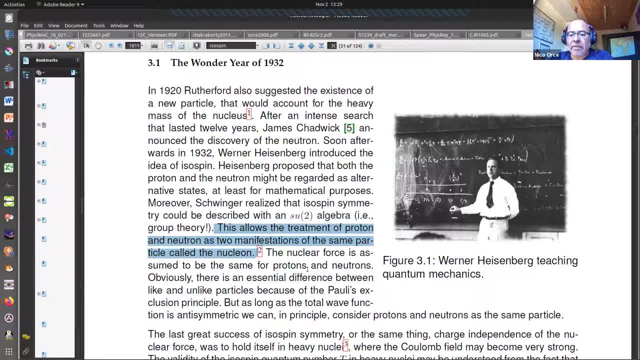 Okay, And then they were. obviously, when you introduce this, you always have to keep in mind that proton and neutrons and nuclei have the same performance. Isn't this all just a goodness of your species? Thank you for recording this. So with that. 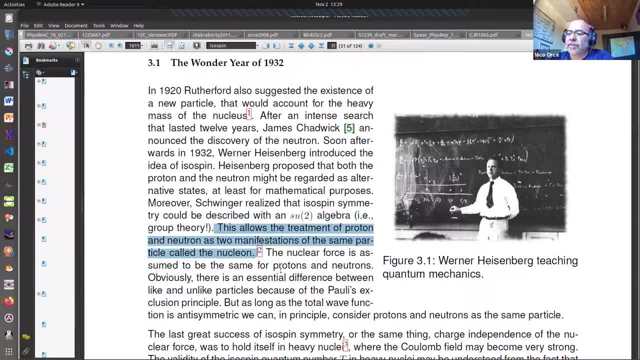 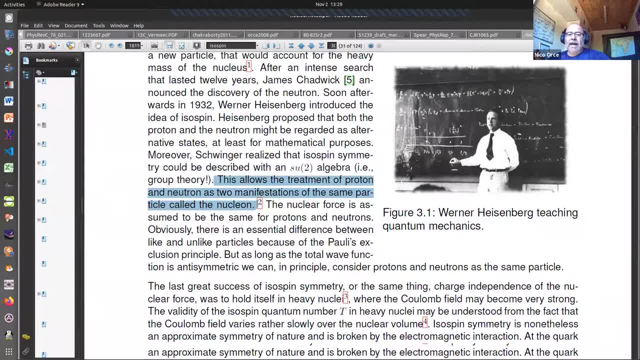 they are fermions and the total wave function which represents a fermion must be antisymmetric, and we'll go through this a little bit later. and it was assumed that the nuclear force is assumed to be the same for proton and neutrons. but this was not entirely true because, as 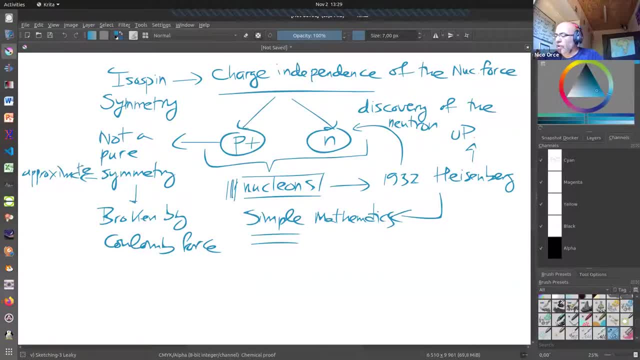 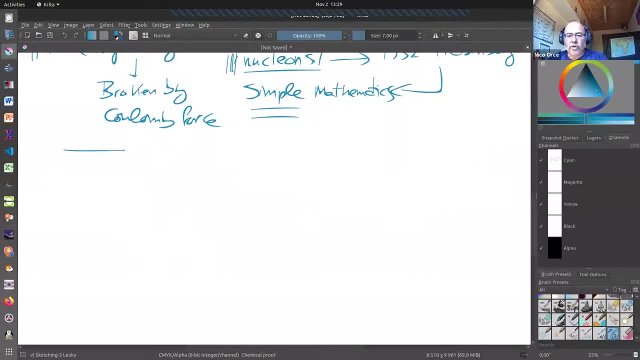 you have more protons and more neutrons. you know the the there's something called the shell model and we go to the shell model later on, but this is one to to relate the shell model to isospin. and we learn, we learn in our next lecture, on two lectures time, that 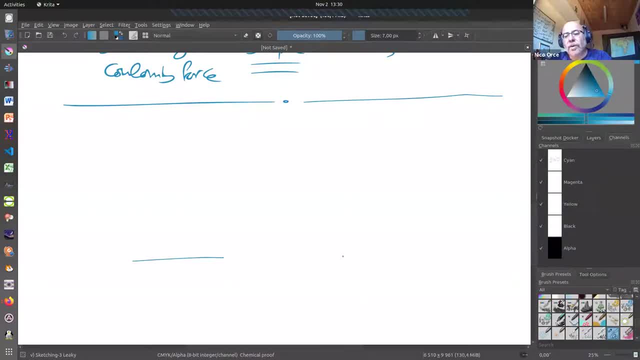 we have a building for protons and a building for neutrons, and the building looks exactly the same. these are the floors and uh, okay, let's make it just. uh, sorry, here we go, one and two, and then one, two and three, right, and we'll learn that this is the. 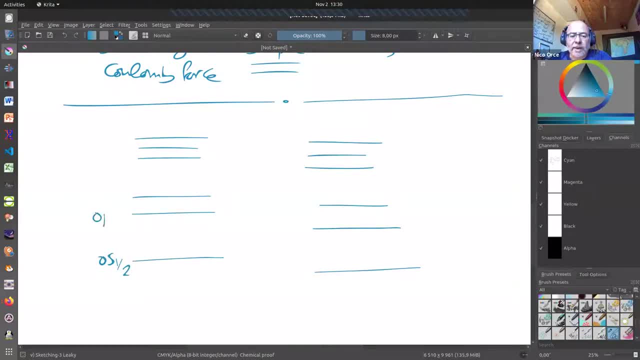 zero s one half. this is a zero p three half, is the zero p one half and this is the zero d five half. this will be the the one s one half and this will be the zero 3 half. and the same thing here. the same thing here: zero d three half. 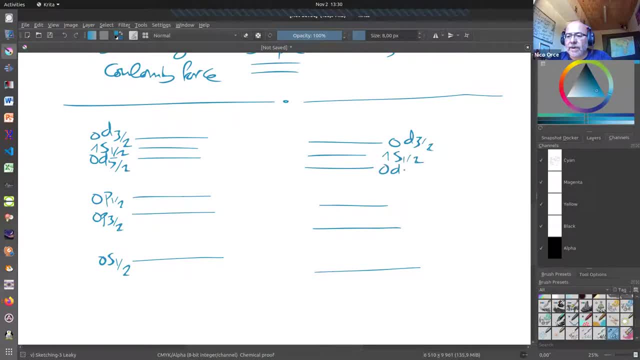 one s one half, zero d, four half. so these are for for protons here and neutrons and this will be the zero as one half and this will be the zero b. three half will be the 0P1 house. This is the floor where we are going to have the protons and neutrons living. 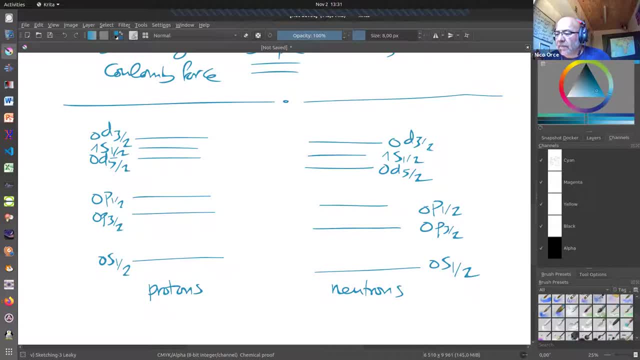 right. There will be a particular building which we call the shell model. There are more floors up there. We keep adding neighbors and protons and neutrons in a way which follows the Pauli exclusion principle. So this is a little bit of the introduction. 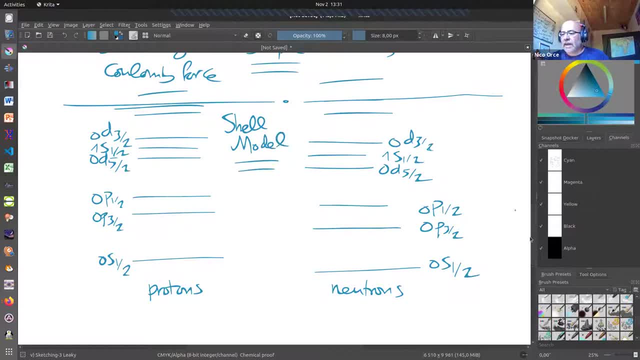 a little bit of a preliminary introduction to the shell model And in this particular case we have that. in this case the occupancy will be two protons, Here we have four. And again this will come because of the Pauli principle only allows- uh, only allows- particles to have different quantum numbers. You have the same quantum number. 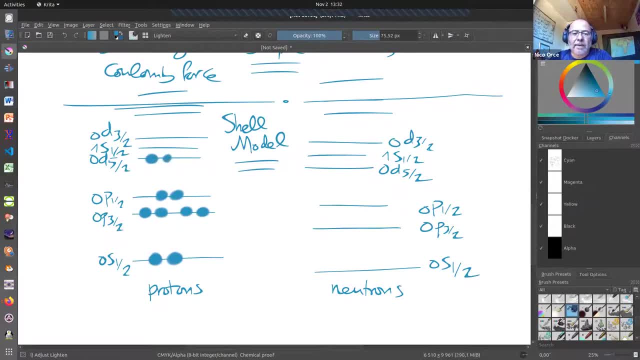 then you cannot live in the same flow. Here we have one, two, three, four, five and six, One and two And here one, two, three, four. And for neutrons will be something similar: One here, two here. one, two, three, four. 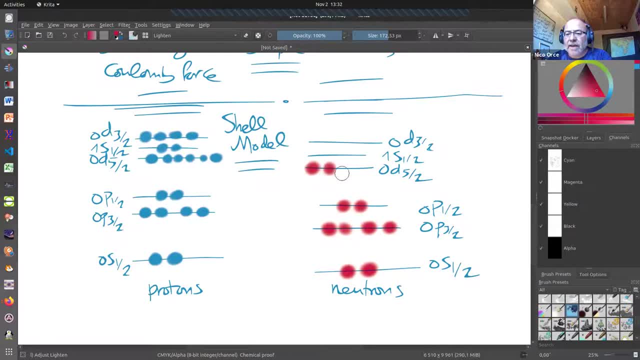 One, two. So you see, we see that there's some kind of isospin symmetry which is manifested in a way. Another one here: Put it here: One and two. And one, two, three, four, Right, And we'll see that these magic numbers, this shell model has special magic numbers. 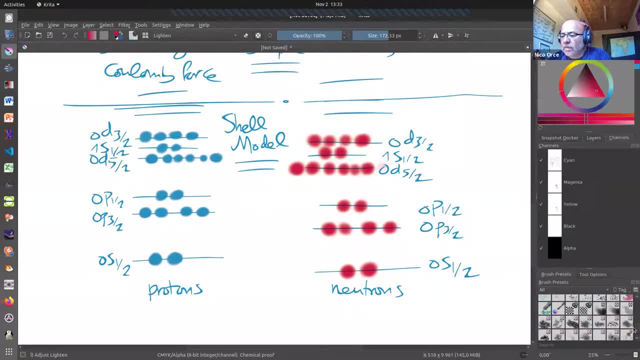 for nuclei to be extra stable. And these magic numbers will be here, two, Here we have eight. Here will be twenty, Twenty, eight, two. And somehow we last week we learned from The Harmonic Oscillator that, uh, we are, we're going to link that next, next week, But these are special magic numbers. 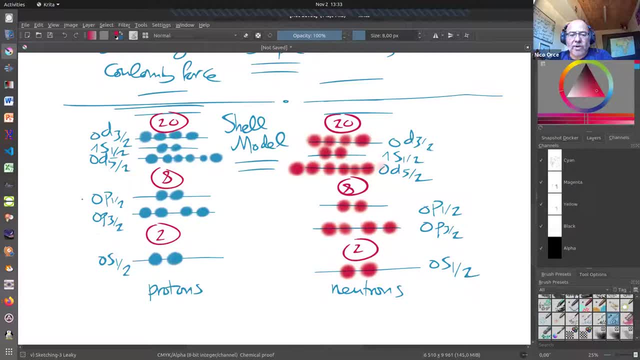 because, uh, a nucleus you know like, for instance, Oxygen 16.. Oxygen 16.. Let me put some green here. I like this pistachio green. Oxygen 16 will be a building like this, where you have 8 protons and 8 neutrons, right? 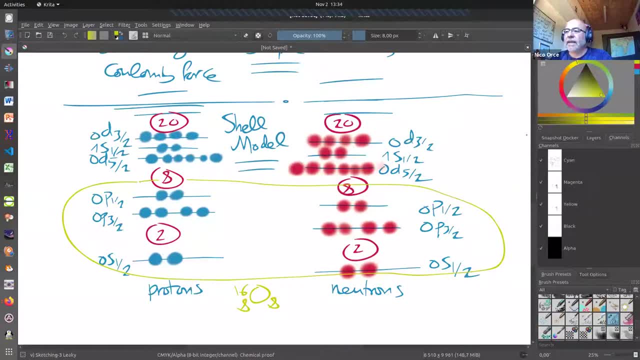 So Oxygen 16 will be particularly stable because these guys to be excited, they need to move up there and they need to cross this shell, this energy here, Right, So these guys will be particularly stable. So someone is raising their hand. Let me just stop sharing here. 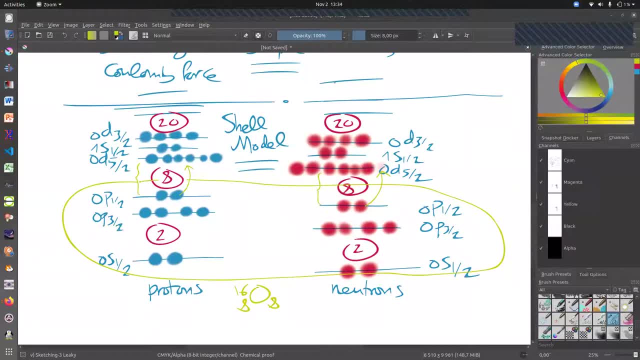 Sayola, what do you need? No, prof, don't stop sharing. I think I'm lost somewhere here. Okay, you're lost somewhere here, So let me Blue and red. Okay, the thing is, I just want to briefly introduce the shell model. 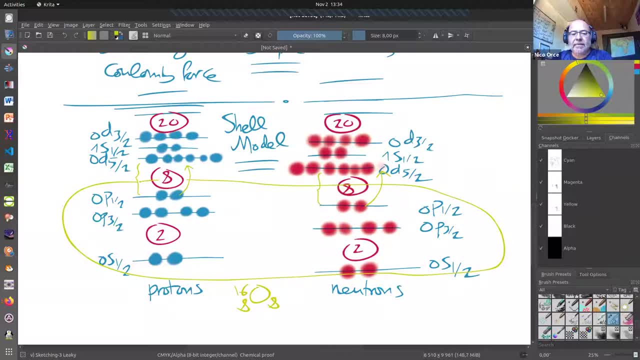 And what I'm saying here is that these guys, these guys, they are protons and there are two protons here. there are two neutrons here. So each ball here is a proton And each ball here is a neutron, right? 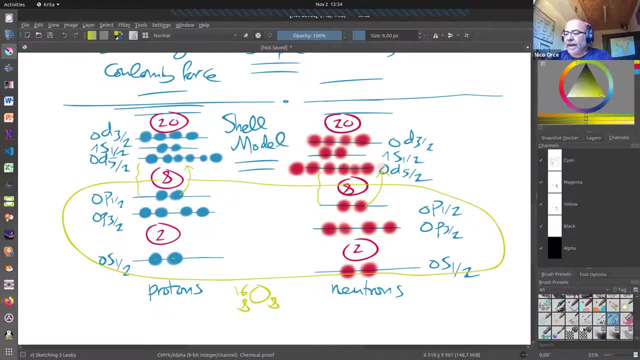 And they have particular occupancies Which depend on the Pauli exclusion principle. It's good that you stopped me, because I just wanted to introduce this- And the occupancy goes like this: 2J plus 1, where J is this number here. 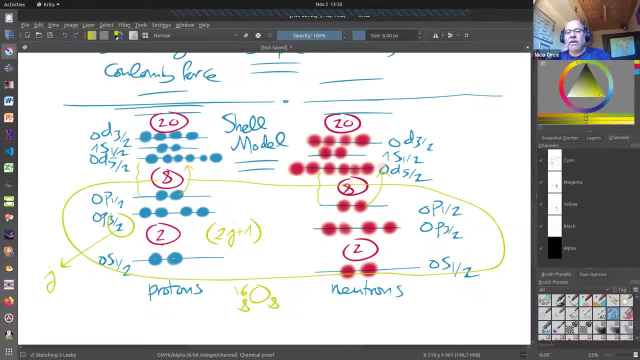 But I don't want to go through this too much right now. I want to focus on the isospin. They will see this long enough next time. I just want to show for the first time. So next time we see this it's not so surprising. 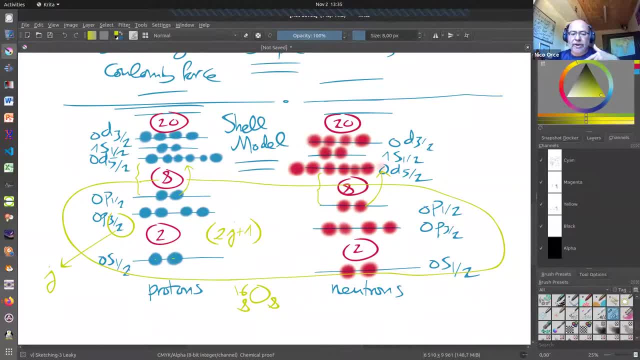 Basically, Here we have: if J here is one half, right One half, So we put J one half here. Times 2 will be 1 plus 1, 2.. So we have two particles. Okay, So this will be the occupancy. 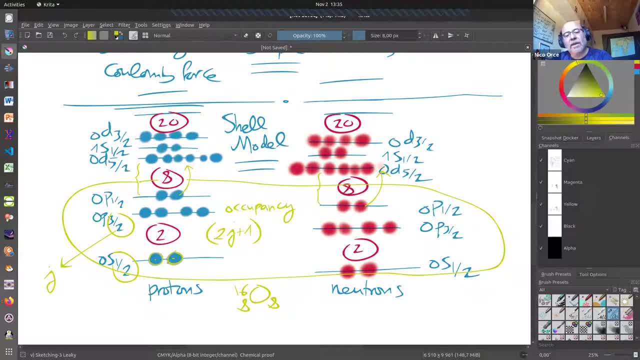 And we learn why: Because these guys, they have different spins pointing up and down, So they may have the same L. This is L. Remember, L is equal to S, P, D, F, G. This is N. 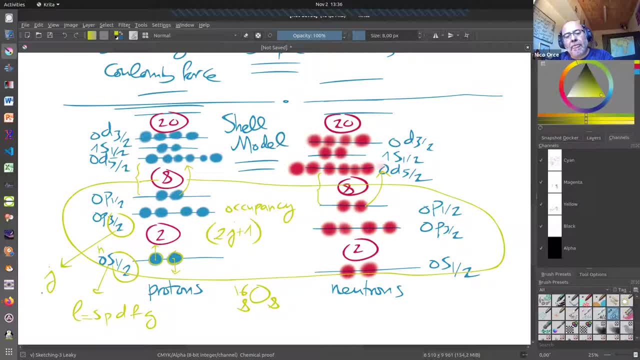 And we'll see here. You know, I don't want to say anymore. This is basically obeying the Pauli exclusion principle, Pauli exclusion principle. And I want to say here only the following: That this level I draw them in a particular way. 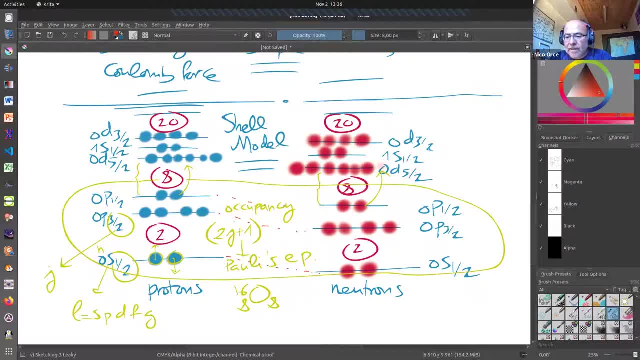 They are not the same. They look the same, But you see, these neutron guys are deeper in the potential than the proton guys. You see, I drew them in a way that these guys always they look like the same building, But this building, this building here, is deeper right than this building here. 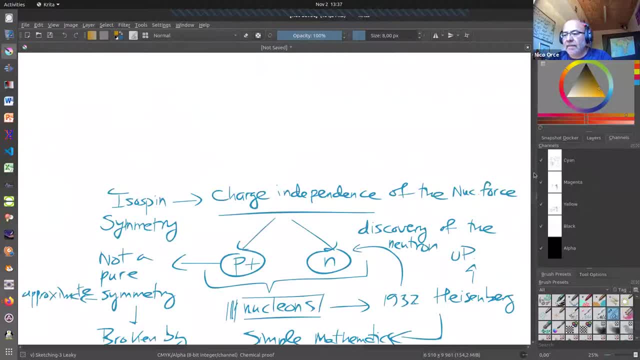 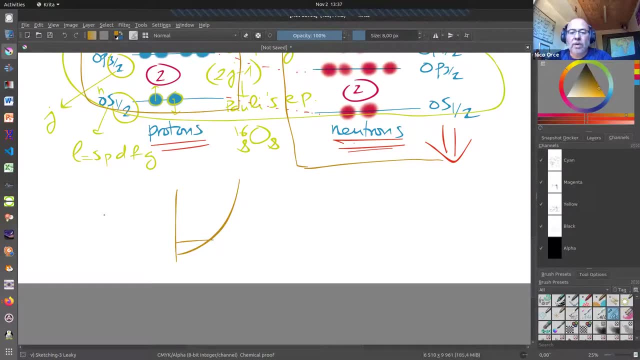 So by meaning that the neutrons in our potential, the neutrons, the neutrons, will be deeper in the potential, in the harmonic oscillator potential, say, than the proton, The proton will be slightly for the same level, for the same flow. 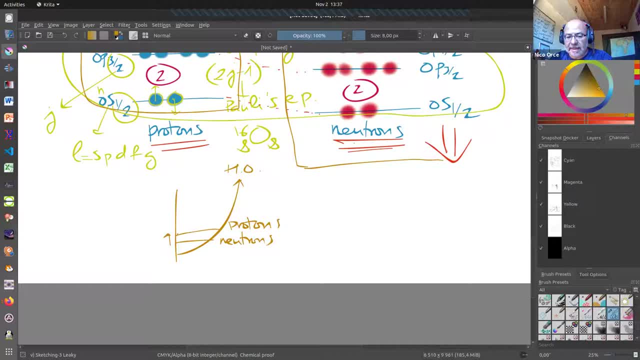 the protons will be a little bit higher than the neutrons. I mean less bound right, Less bound. The deeper you are, the deeper you are, the more bound you are right. But because of the protons having a positive charge. 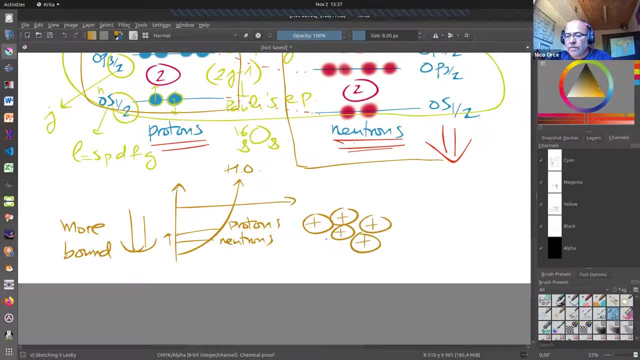 the more positive, The more positive charges you are you have here. as you increase the protons, there will be a repulsion right, And this repulsion is manifested right here, And the purpose of this exercise was to briefly introduce the shell model for later. 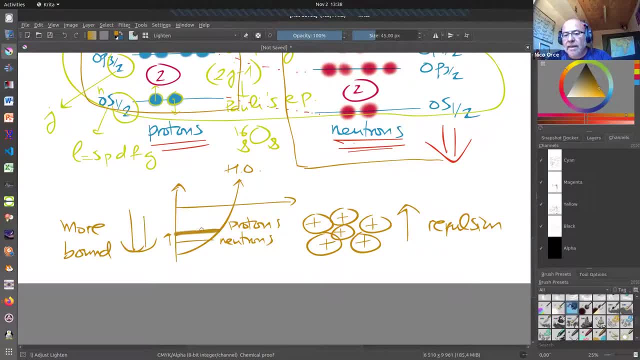 But the main thing was to tell you: look, look guys, this guy is less bound than this guy, And the only reason is the number of protons, right? So obviously, the more protons, the less bound it will be. 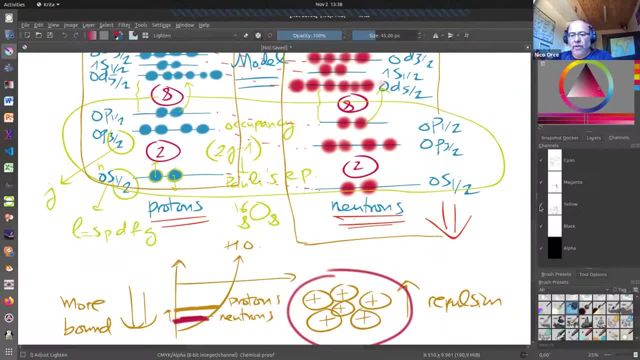 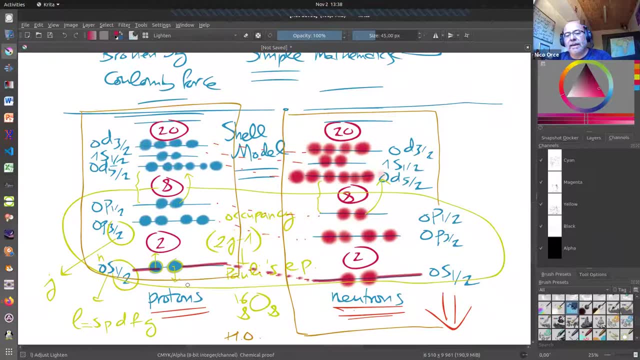 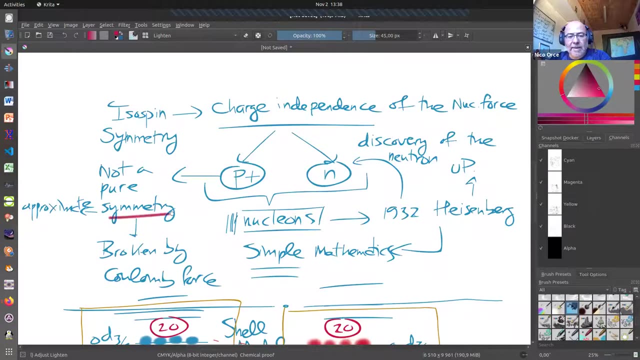 So the neutrons for the same particular flow, right for the same particular flow, they will be lower, a little bit lower than the protons. So by this I want to say that the isospin symmetry is an approximate symmetry. 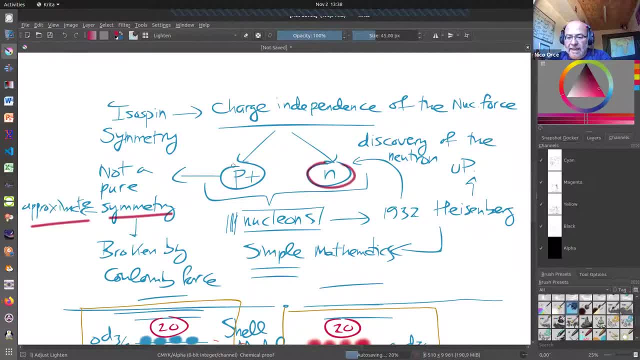 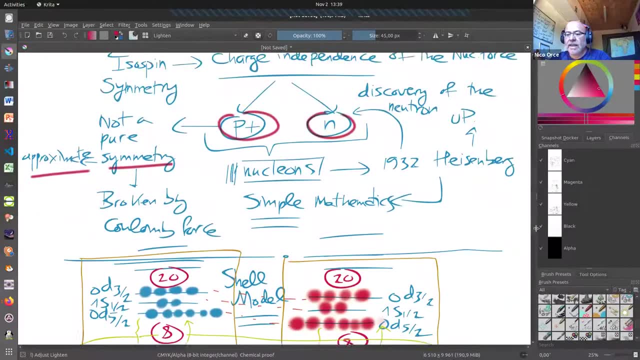 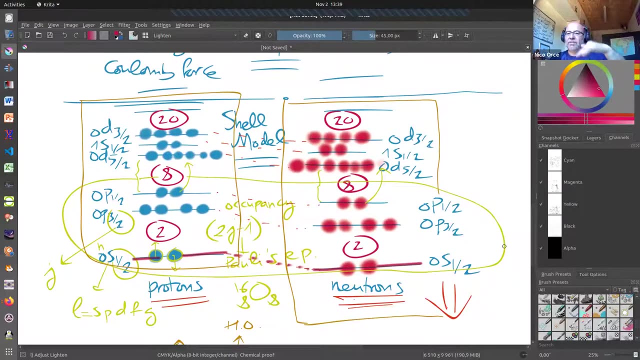 because the neutrons are not exactly the same as the protons, right? This was the whole exercise of drawing this shell model, But I want to explain this in more detail. I just want to have a first flash, okay, of this building that we're going to be learning a lot in the next lectures. 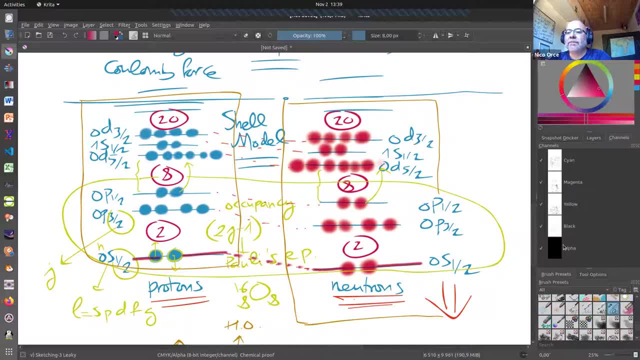 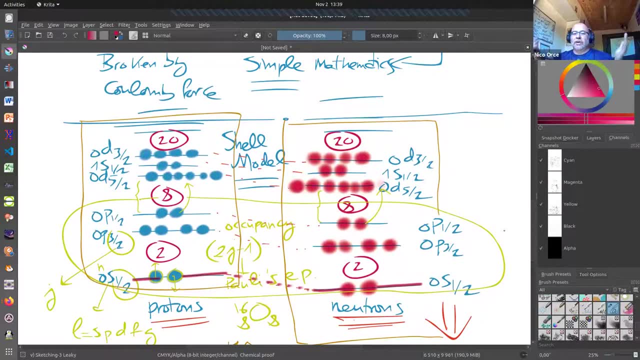 Okay, guys. Just I just want you to have a first view of this building. This is how how we- how protons and neutrons live together- say, We can only put two protons on the first floor. We can only have four protons and four neutrons in the second floor. 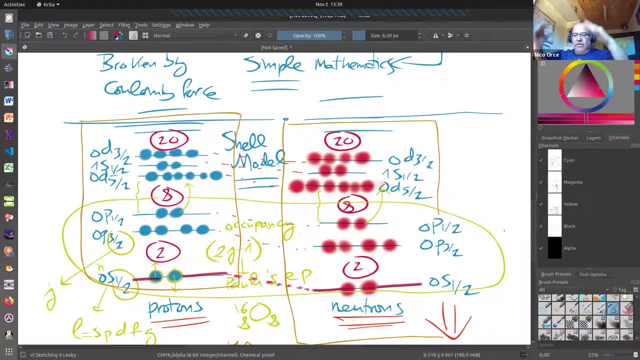 Two neutrons and two protons on the third floor, and so on and so forth. There's a gap here. So this is a particular building which is that doesn't have. you know, like we see buildings around us, you know the same distance between floors, right? 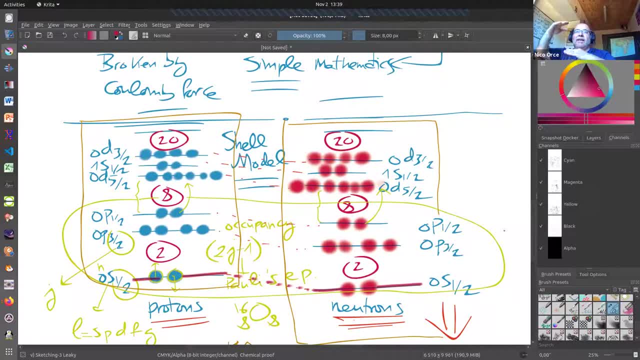 So this is a kind of crazy building: One here, then there's a big gap and you have two, two narrow floors there and there's another gap. So basically this is the building of nuclei, the shell model. 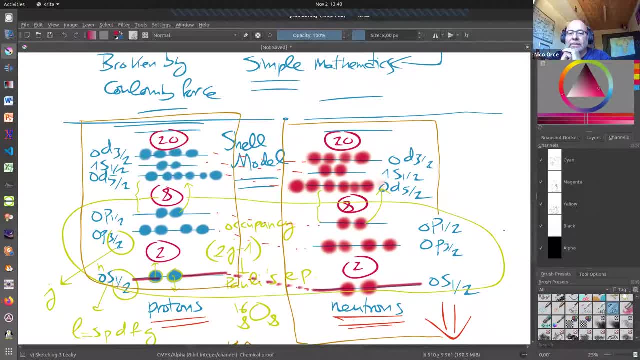 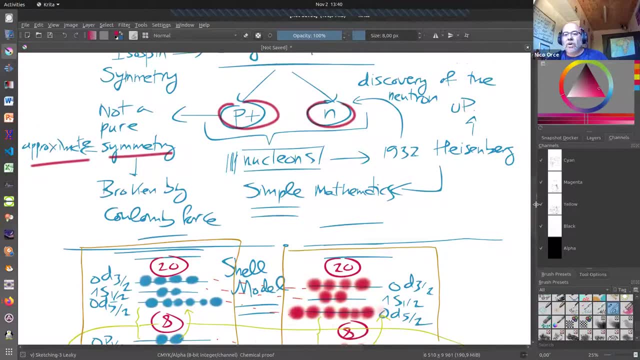 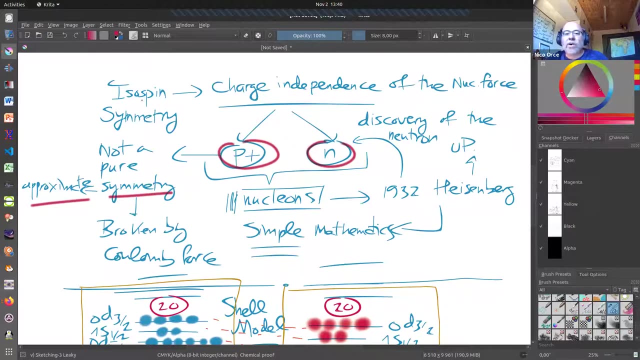 How you, how they are, how they are placed within the nucleus. All right So, but today, as we are discussing, we're going to focus. Our main focus is on isosceles spin symmetry, And for that we go here. 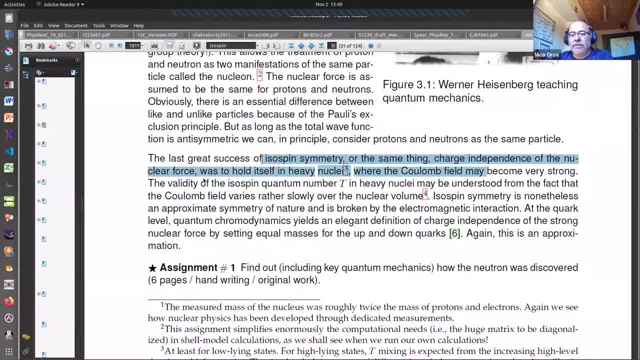 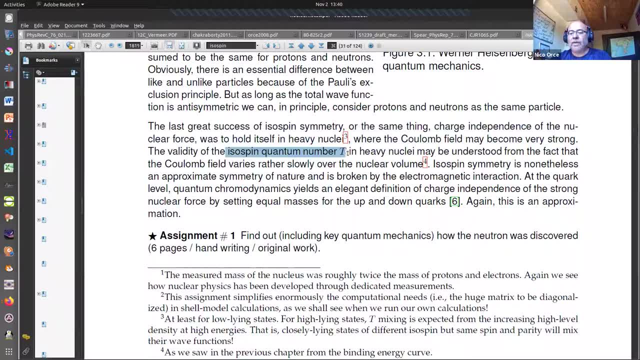 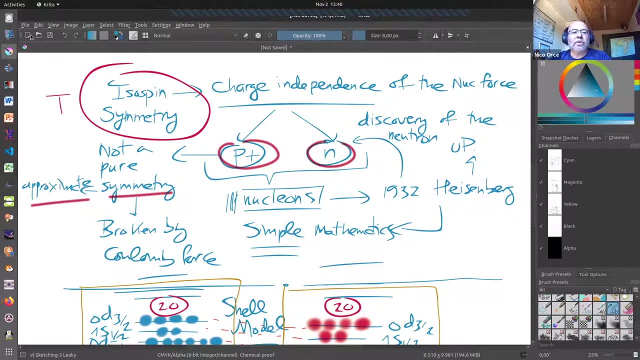 The spin symmetry, or the same thing, charge, independence of the nuclear force. You know, you can read these things: The spin quantum number is is called T, right? So the spin symmetry, the spin quantum number is T And we're going to open a new. 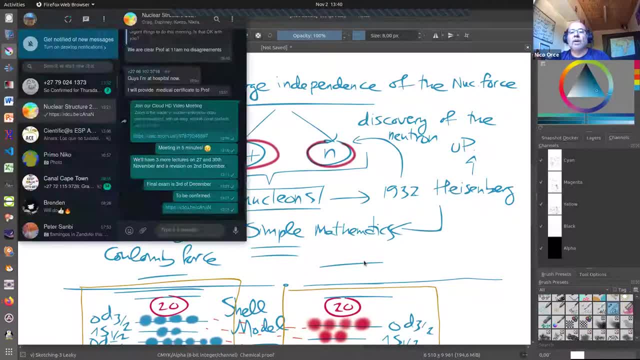 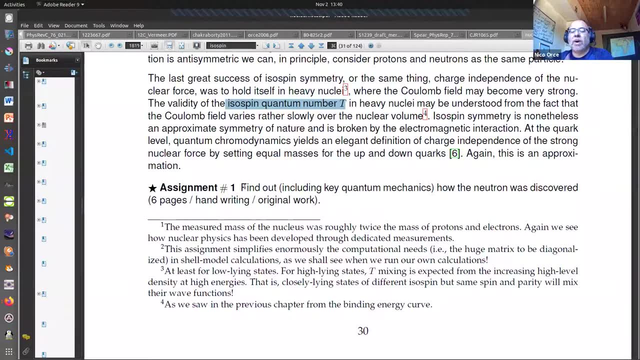 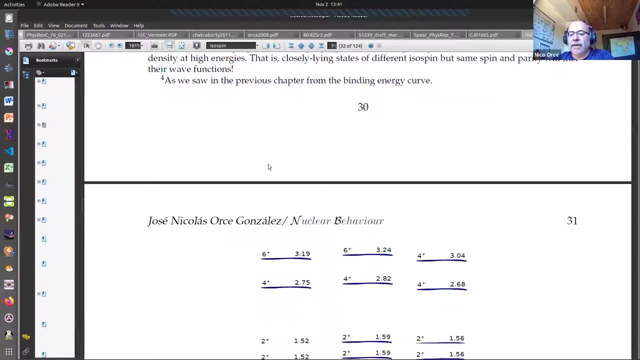 a new page And while we open a new page, we're going to see. you know what? the assignment number one? I want you to read through this: how the neutron was discovered. I want you to learn how these these things happen. 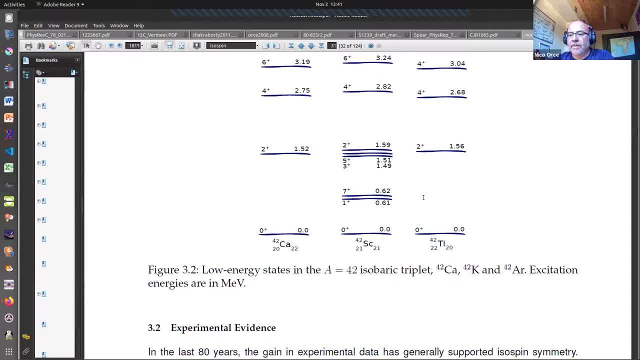 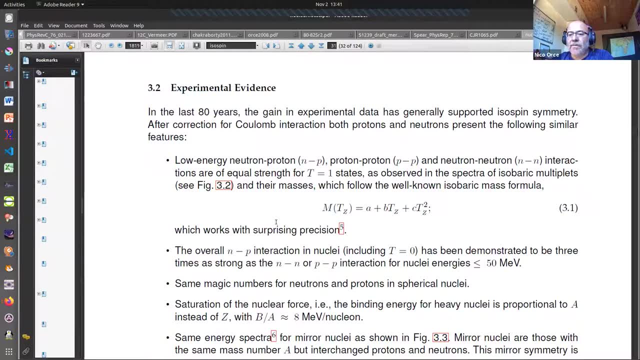 And then we're going to learn a little bit more on this isosceles spin picture. Then you have the experimental evidence for isosceles spin. So you will have that The low energy neutron proton, proton proton and neutron neutron interactions are of equal strength for these T equal one states. 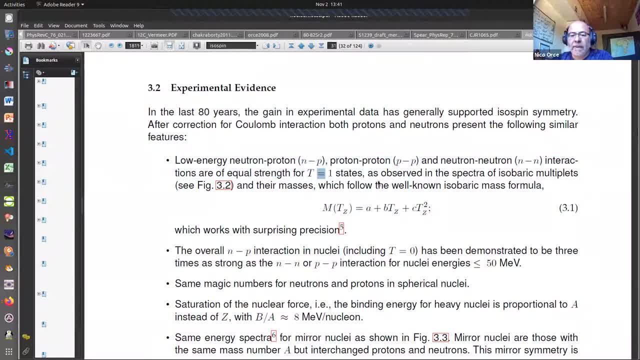 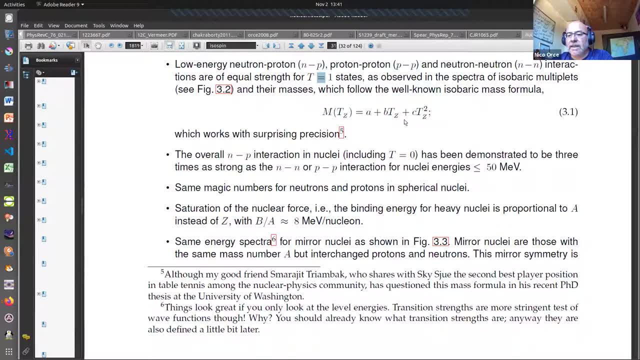 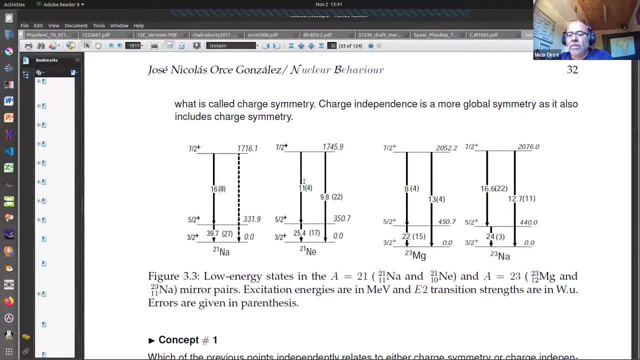 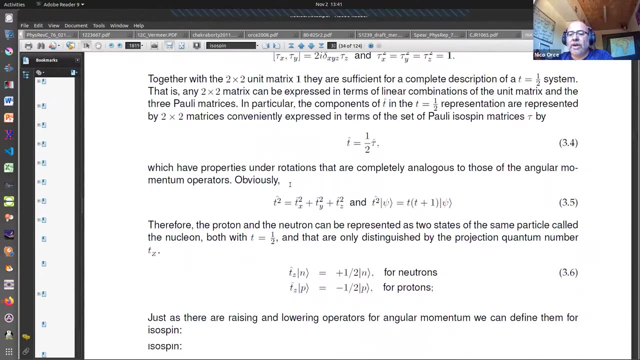 And we're going to learn what is a T equal one state. right now, Before we learn about this experimental evidence, we are actually going to learn what is T equal one and T equal zero, And for that we are going to to go directly to the concept. 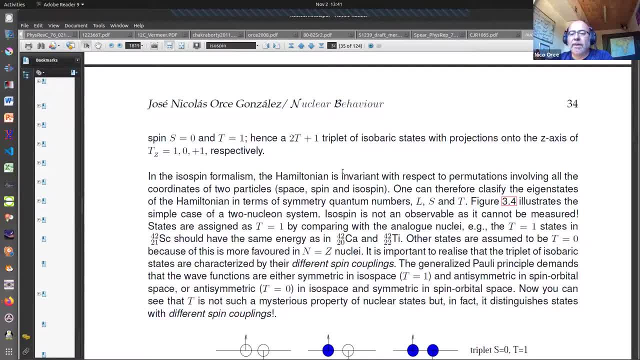 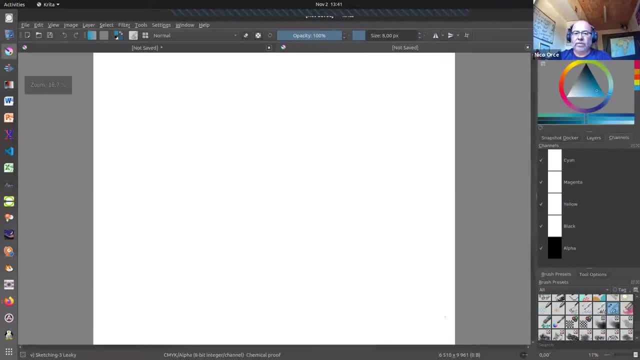 So, when this is just formalism, I want you to go through that. But let's go to the concept here, And we're going to remember the idea of the deuteron. We have a deuteron-like structure which, which is just two protons, two neutrons. 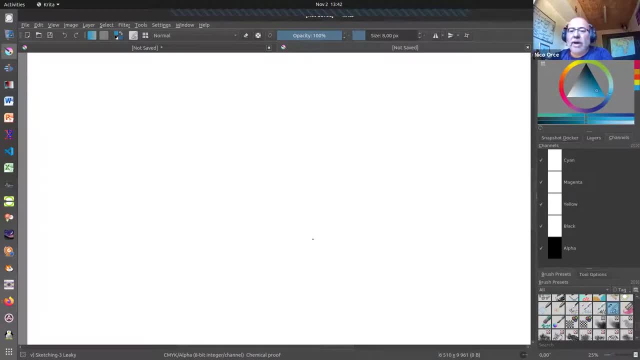 or one proton and one neutron. We're going to have the possibility to have deuteron-like. So we're going to have either two protons And, as you can see, two protons- Let's say two protons here- Obviously the spin. 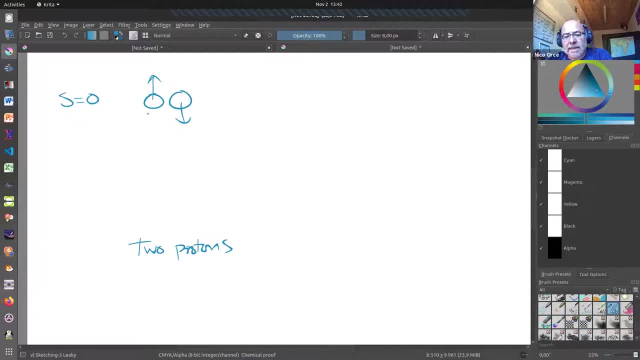 the spin must be equal to zero, right? Because this has S one half, all of them has S one half, but they are in opposite directions, they are antiparallel, right? So then the total spin number, the total spin total, will be S equal to zero. 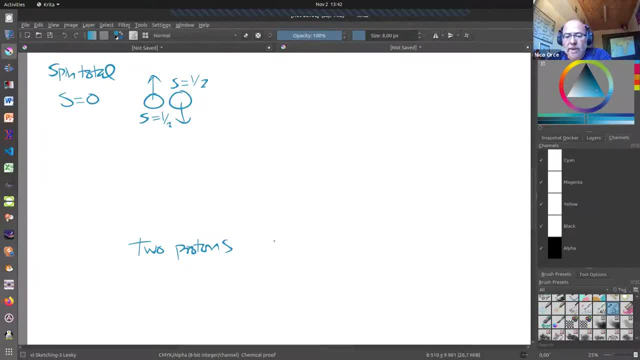 And then we have one proton here and one neutron where you can have the same kind of structure. Let's put this guy here And let's write the proton on red, Let's distinguish them. And here we have two neutrons And again the same situation. 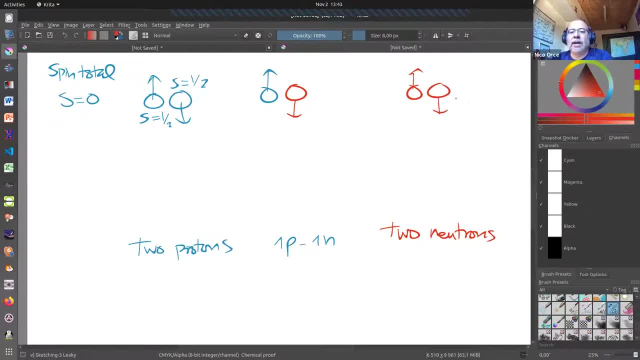 where you have the spins pointing up and down. So for each of these guys, S is equal to zero, right? S is equal to zero here. S is equal to zero here, Correct, That's clear, right, Because the spins are antiparallel, right. 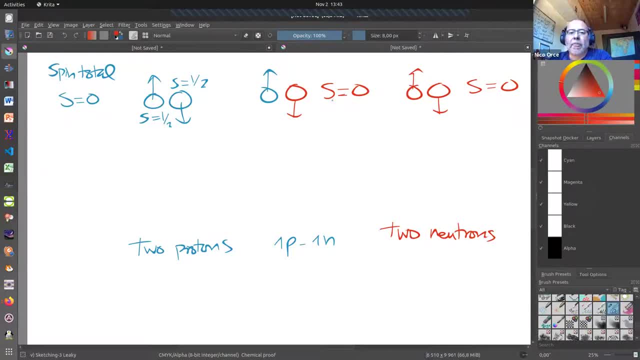 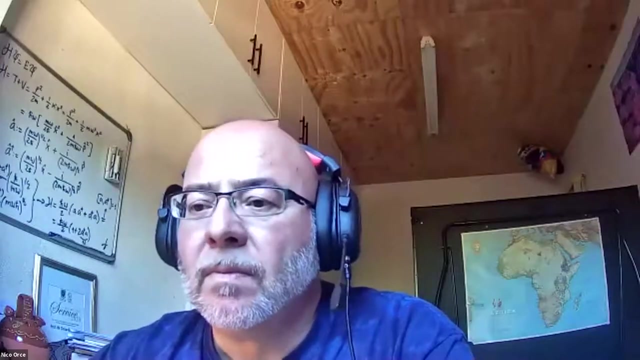 Luasi, is this clear? Basically, we're just having a two-nucleon system, Guys, before we move forward. is this clear? Yeah, I think it is. We're going to shoot it. Let's go. Ciayola, you have a hand raised there. 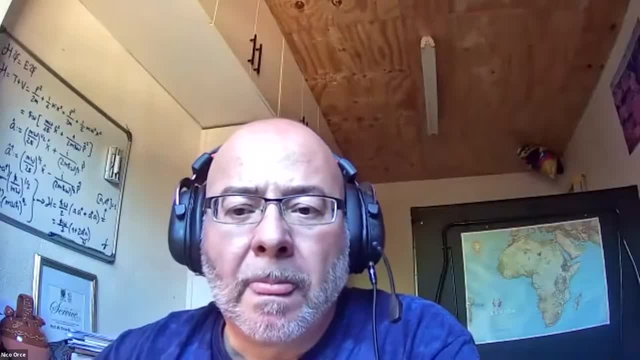 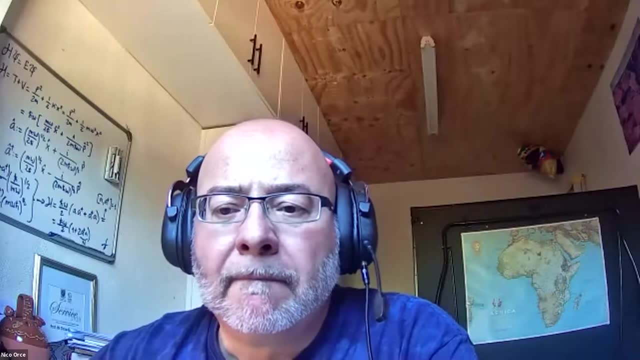 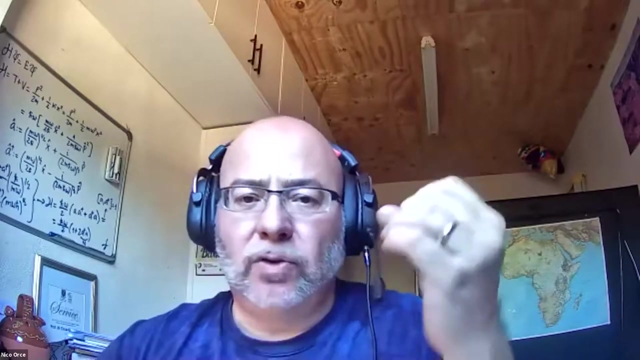 Do you want to know anything You want to ask? Oh, Your hand is from before. no, Yeah, So Yes, Prof, Okay. So, basically, we are having two particles and they are coupled up and down, right? 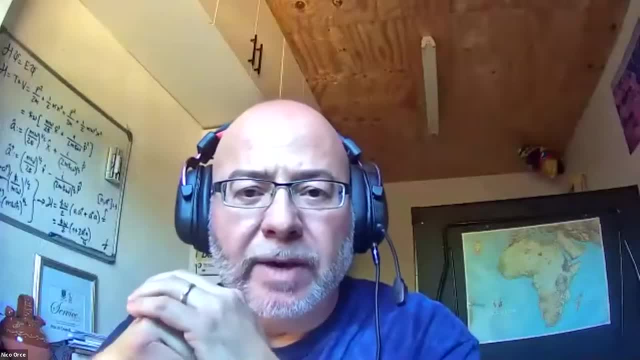 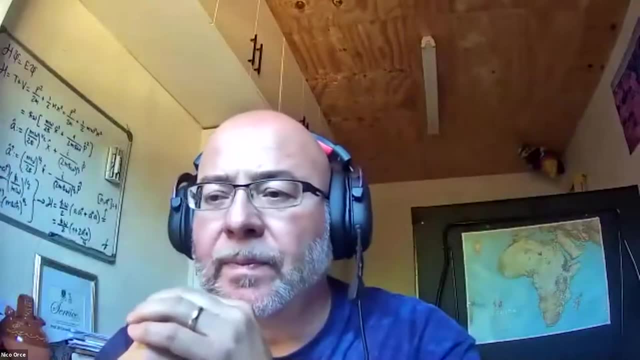 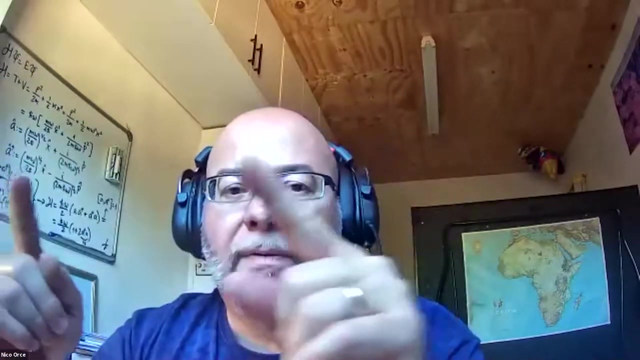 So the total spin, which each spin for each fermion, is one-half. So one-half minus one-half will be zero, right? So we have three possibilities. Three possibilities, But we need to have an anti-symmetric wave function. 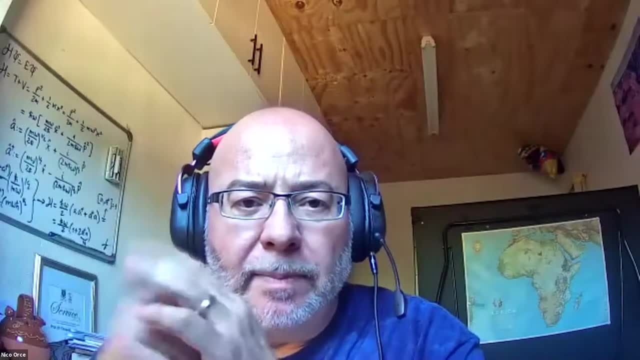 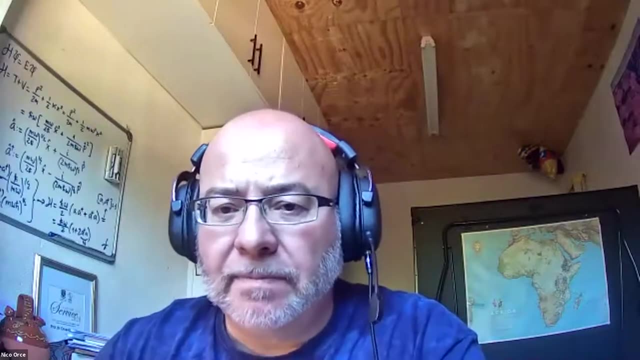 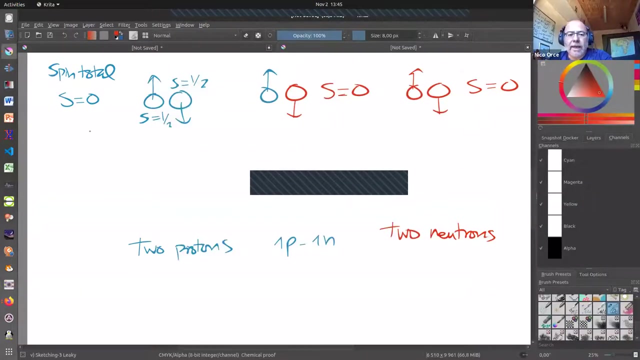 And to have an anti-symmetric wave function, the total, the product of the wave functions, must be odd. So in this particular case, let's share the screen. Well, we are going to introduce the isospin quantum number T. 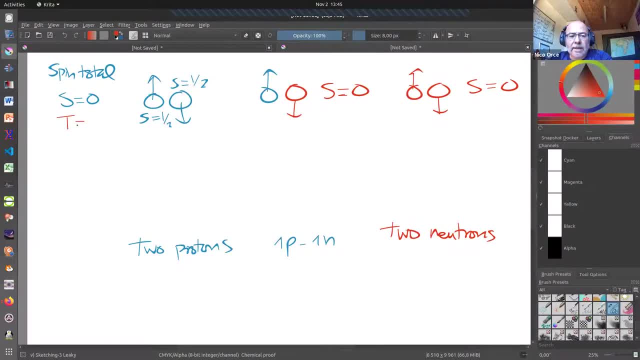 and this T is going to be one or zero. This particular case will be one, because we have zero and we have one. So we make sure that the total wave function is. Sorry, Prof, Tell me So that you know that the function of the wave function. 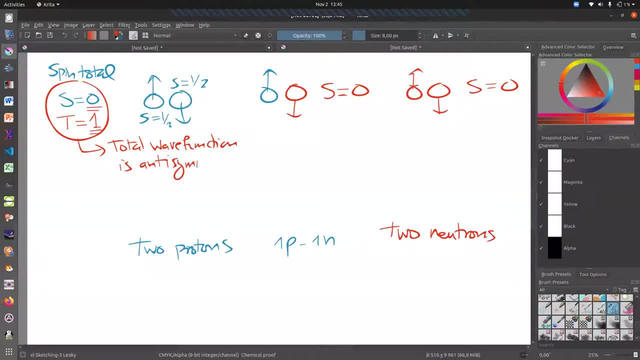 is one, Okay. Okay, So that you know that sometimes S becomes one or zero, Right, But we do determine that when we know the parity. Now that you don't know the parity, how do you know that S is zero? 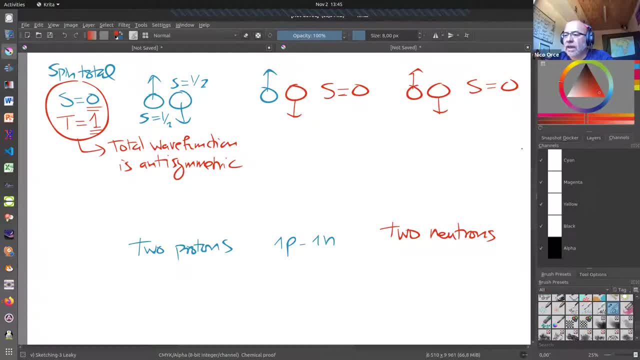 Okay, We know that S is zero, because That's a good question, But let's go back down here and show it to you. So we have This: guy is S one-half right, Actually, plus is S one-half. 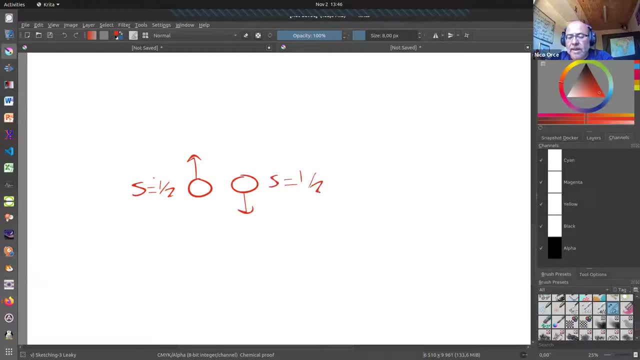 and this guy is also S one-half right, But this guy is pointing up and this guy is pointing down. So the total S, which is S one, let's call this S one and this guy S two, you know. 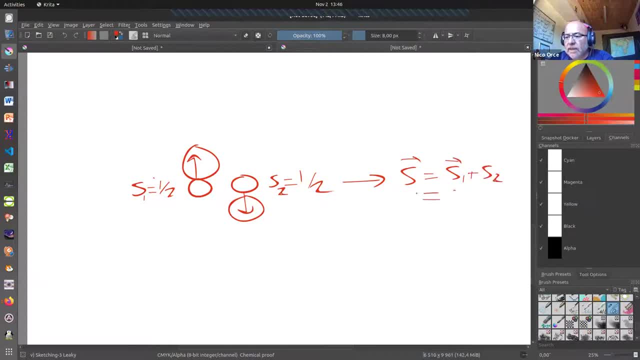 plus S two is equal to total. you know, S will be zero here. If this guy is pointing up, the spin is pointing up, then the total S one plus S two will be equal to one right, So S will be equal to one. 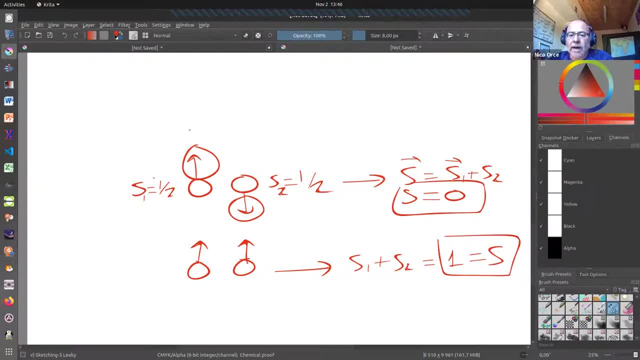 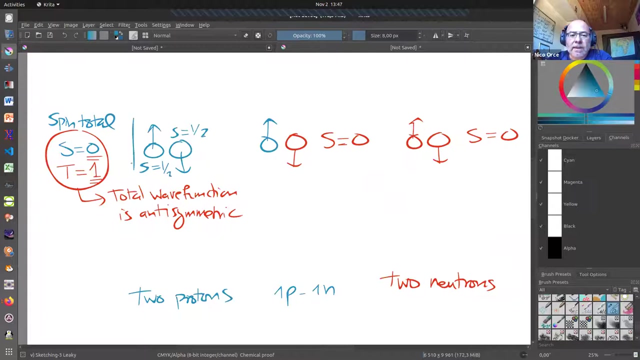 S will be zero for anti-parallel spins, right, And for parallel spins, then we have S equal to one. Correct, Is that clear? Good, So that's why, here, all these three states, all these three states, they have S equal to zero. 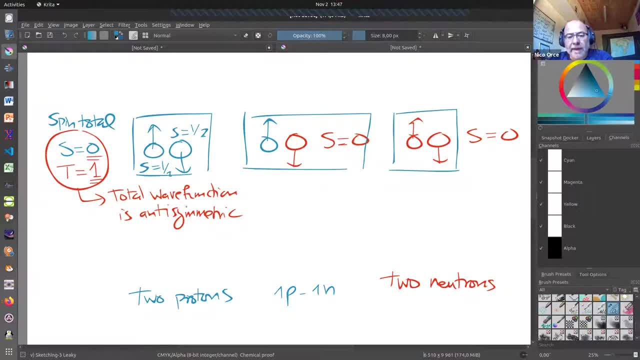 And to make it anti-symmetric, when we introduce the isospin, T must be equal to one, because zero and zero, even and even give you a symmetric, an even function. So the total wave function must be anti-symmetric. 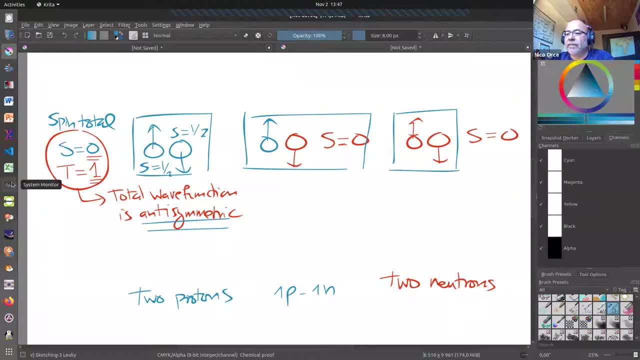 which you need to have an odd number here. Okay, So we are talking about having again proton and neutrons, protons and neutrons pointing up and down, And this is just the picture. However, there's yet another picture. 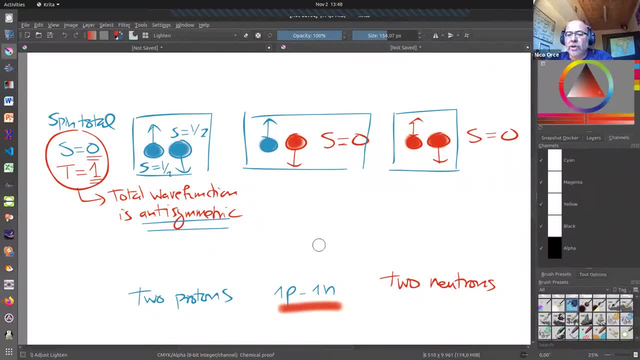 for this particular case, When you have one proton, one neutron, we can have this guy. actually also. There's another possibility And we can have this guy. And for this particular case, we can also have the spins pointing up here. 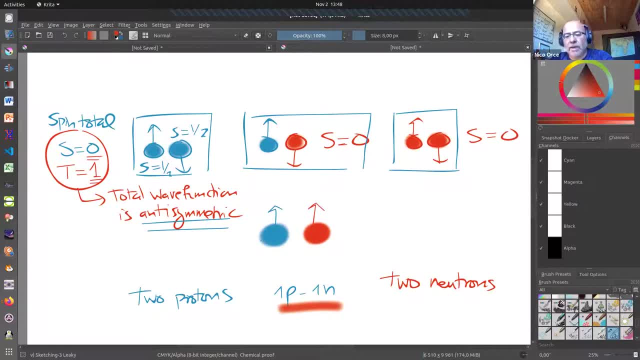 and the spins pointing up there Right, Because these are different particles So they're not the same particle. One is a proton right And the other one is a neutron, So the spins can be these two quantum numbers can be the same. 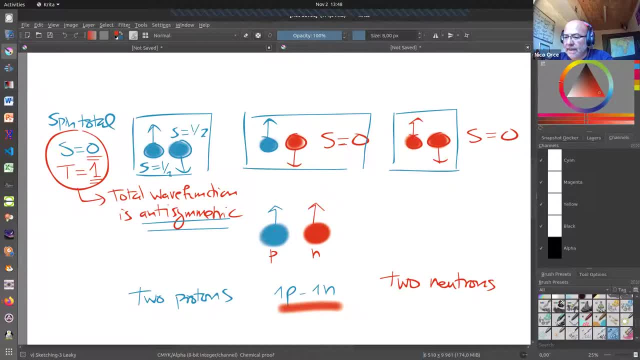 because they're not the same particle. So for this particular case, we have the situation where the spins are up to one and which imply that T must be equal to zero, Right? So these guys, here is called the, it's called the triplet. 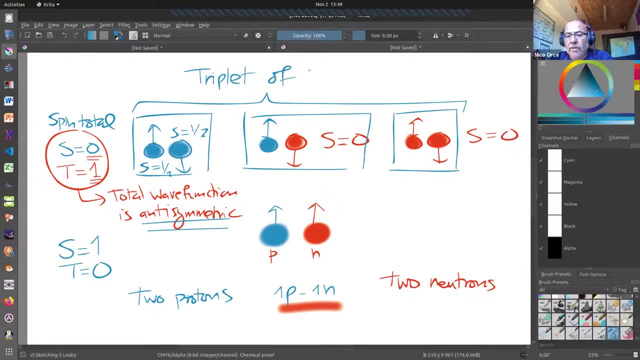 triplet of isobaric analogs And this guy is simply called a singlet. right, Because a singlet? because there's only one way. Obviously we cannot have two protons pointing up, because then you have the same quantum numbers, right. 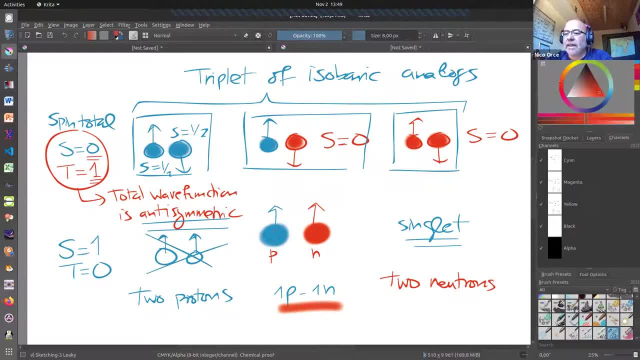 So this is not allowed. And the same thing here: you cannot have two neutrons pointing up because they are the same particle. That's not allowed according to the to the Pauli Pauli's exclusion principle right. 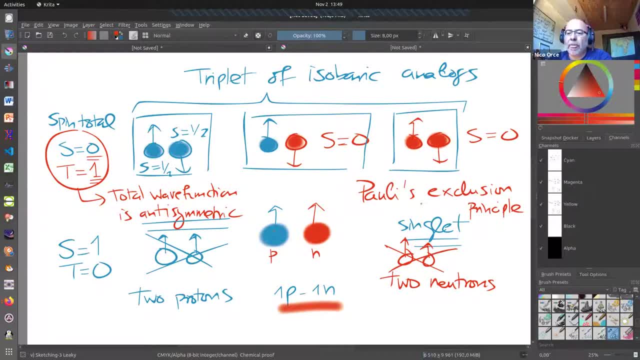 Is that correct? Are we following now? So now we are going to see this in real life. Now we are going to see this in real life and we are going to investigate. The best thing is that we do it ourselves. 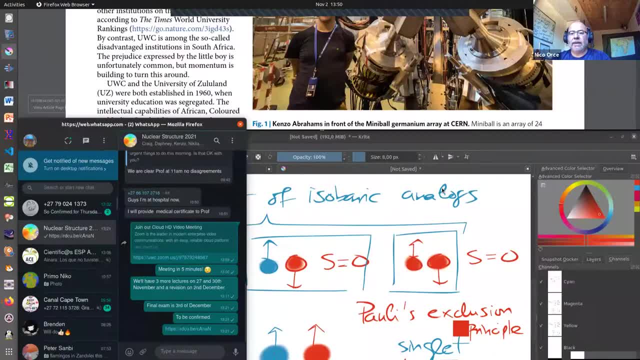 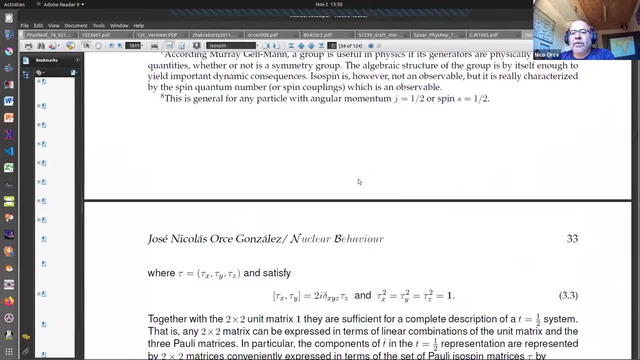 And we go to the NNDC, for instance. Let's go to the NNDC. here You have the example of this, example of these guys, these guys- but I want to see these guys. here You can see calcium-42,. 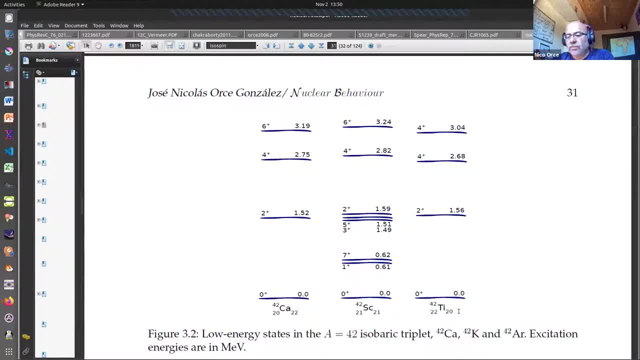 scandium-42,, titanium-42.. Okay, So these guys will have. as you can see very clearly, these are. this is the two-neutron system, All of them. they have 20-20,, 20-20,. 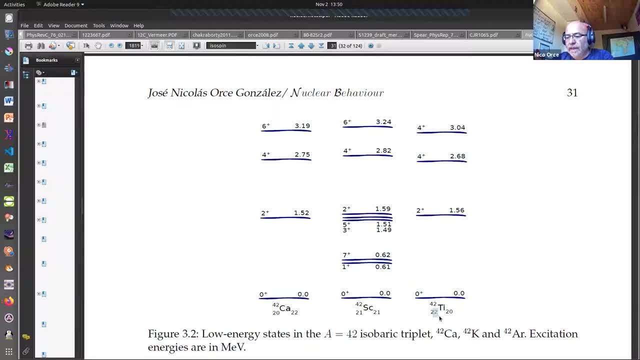 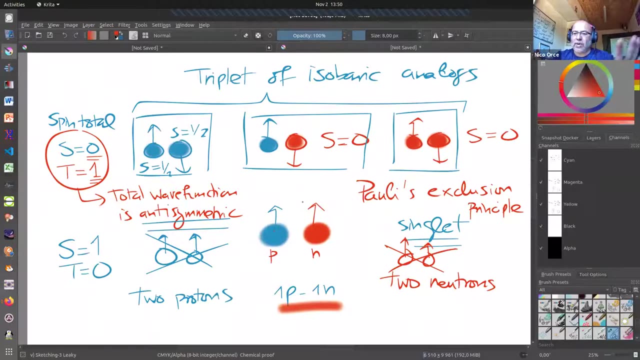 20-20,, but there's a two extra protons here, extra two neutrons here, and there's an extra proton, an extra neutron here. So basically, this is the same situation as we have here. So now, 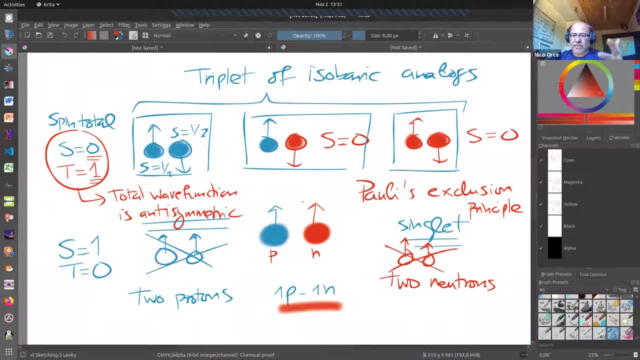 we are going to look at the, at the two. So we have introduced isostein, you know, by means of having an anti-symmetric wave function. So the t-quantum number is equal to one. We have a knot. 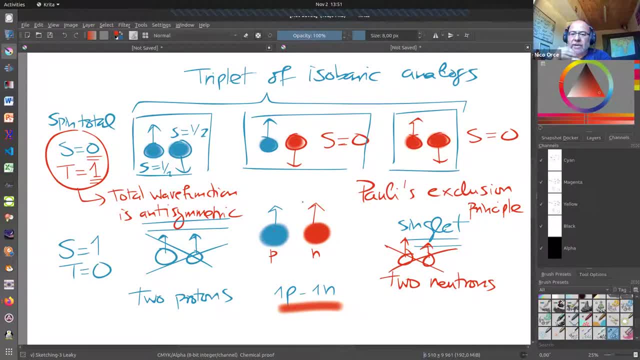 isostein when s is equal to zero, and isostein is equal to zero when s is equal to one, when the spins are pointing up. But that particular case only happens for the, when you have protons and neutrons, right. 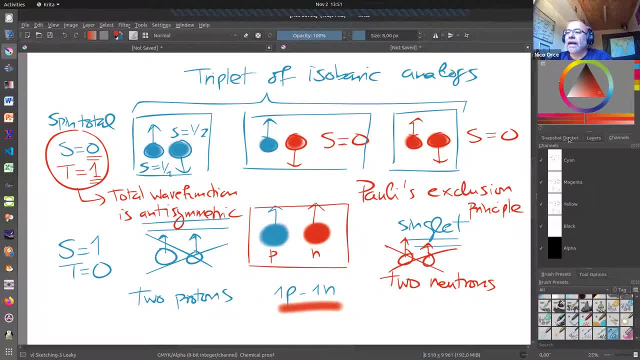 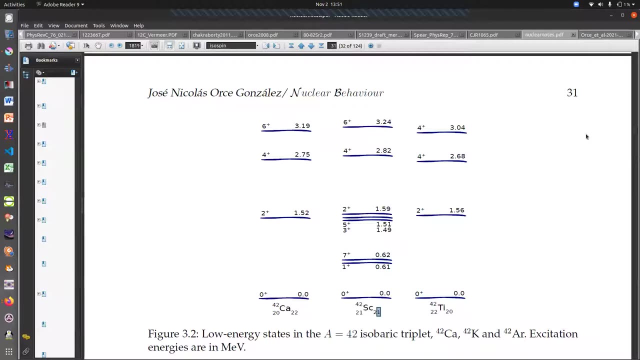 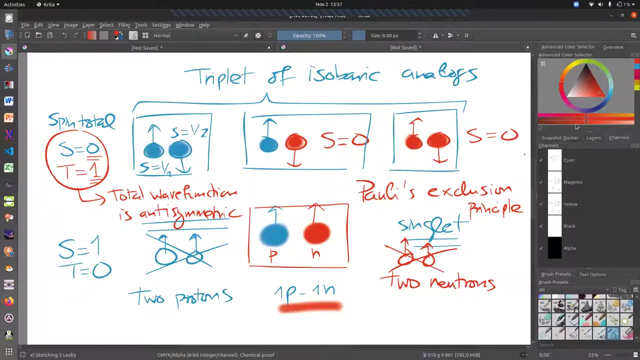 When you have different particles. Guys, questions. Okay, let's follow up. So now we have a situation here, So tell me. It means that if we have t is equal to zero, we have two wave function, which is symmetry. 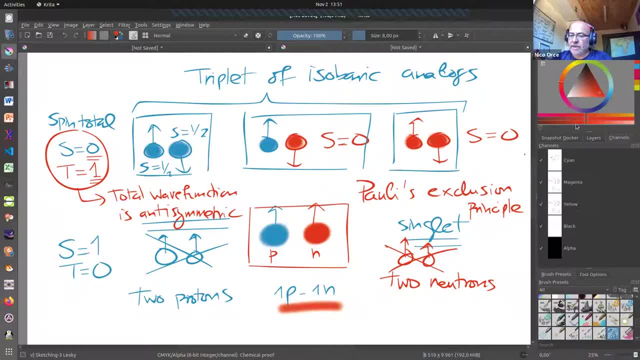 Well, when t is equal to zero, s must be equal to one. Always there must be a knot or a number right. The product, the product, the product of the two must be odd, Always, always. we must satisfy. 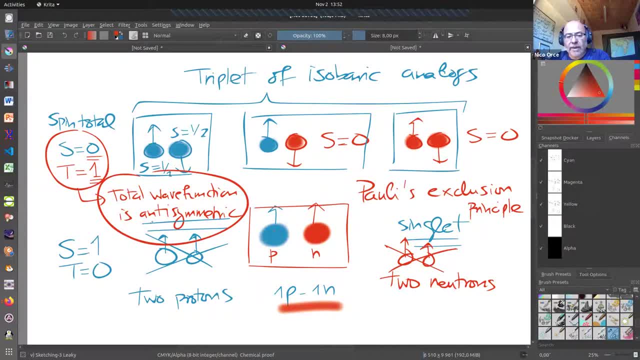 that the total wave function when fermions are involved. it must be anti-symmetric, And for that to happen, the product of these two must be always equal to a knot number, right? Okay, Anichuti? Yes, sir. 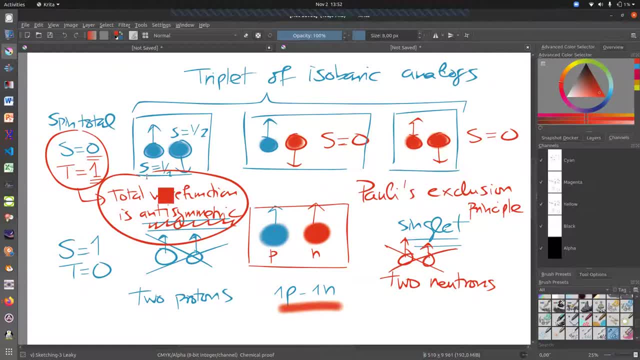 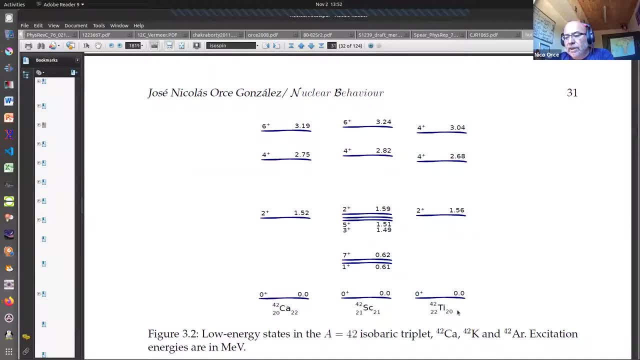 Yeah, Okay. So now we go here and say, okay, look, let's look at this, at these guys. So let's say that 2020,, 2020,, 2020, doesn't affect nothing. 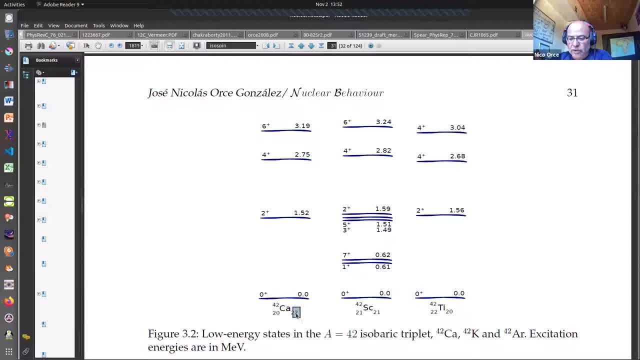 But here there's an extra two. This is two neutrons. Here we have one proton and one neutron, And here there's an extra. two is here in the two protons. So we have the same situation here. 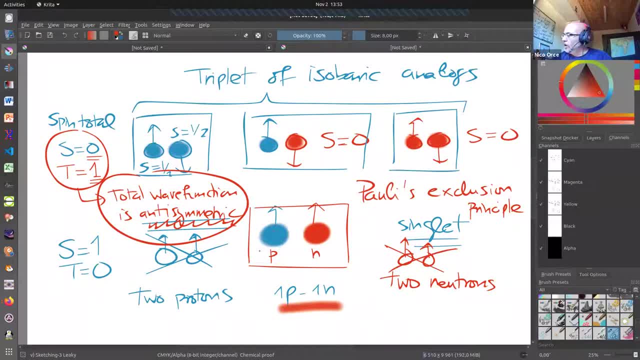 Now let's compare one with the other. So in this particular case- and I'm going to write this in a special- let's see what this guy does here. Okay, this guy is doing something strange, but I like it. 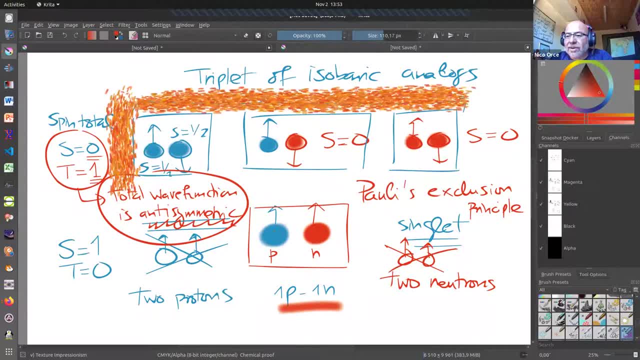 So let's look at this guy, What this does. all these fellows, all these fellows- oh, I did it too strong here. Okay, Here, This triplet means that the nucleus having two protons, and now we are relating. 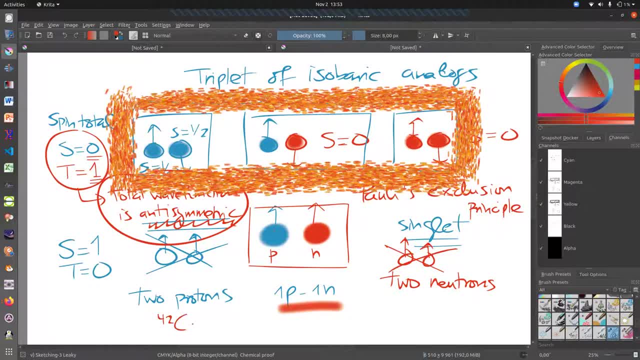 we say this is 42 calcium with. oh sorry, sorry, that's not the two protons. Let me see, That's 42 titanium. 42 titanium here. Bring this a little bit down. Well, not so much. 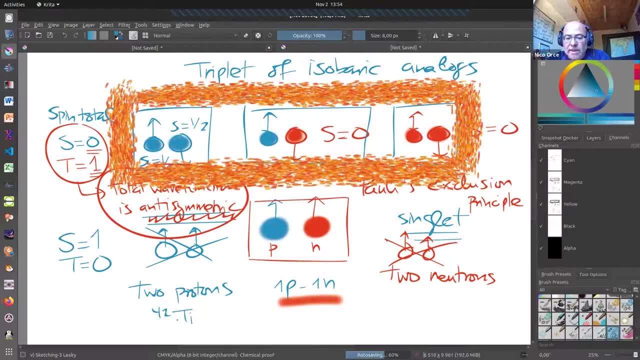 We don't lose the not so much, but 42 titanium is 22 protons and 20 neutrons. This guy is called 42 scandium, with 21 protons and 21 neutrons, And this guy is 42 calcium. 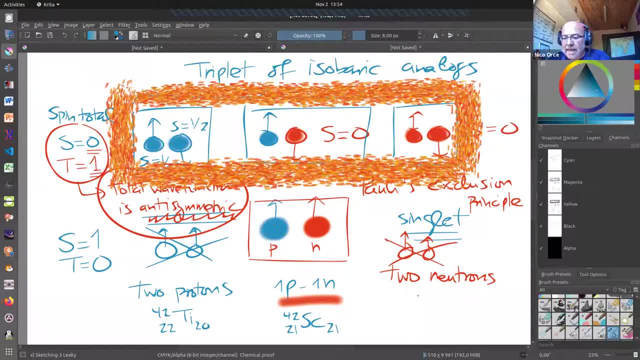 with 20 protons and 22 neutrons. So they take these twos, these twos and these twos and we are going to compare with this picture. So let's see what this guy is doing. So let's see. 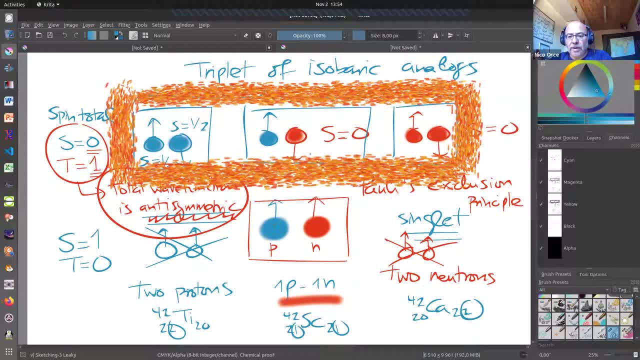 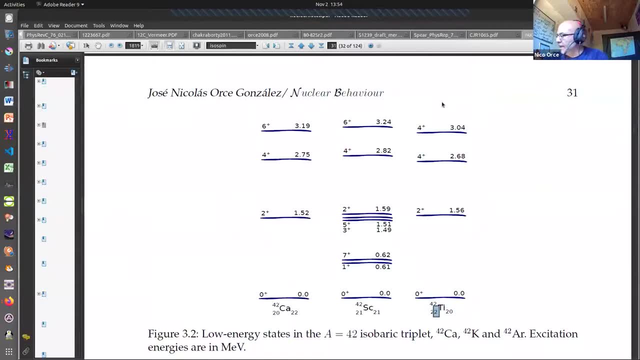 what this guy is doing. So let's see what this guy is doing. So let's look at the triplet. So what we see is the following guys And this is very, very interesting. So look at this. 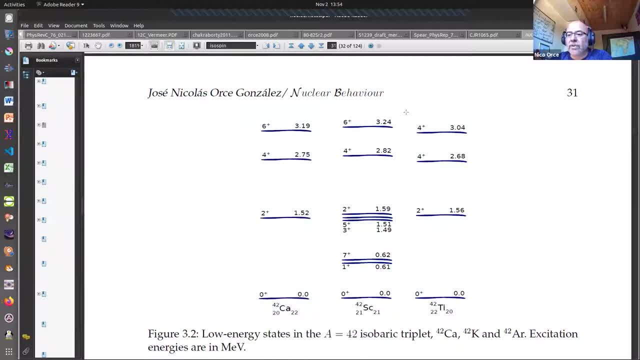 This is the scan, the calcium 42. And look the comparison between calcium 42 and actually titanium 42.. Actually, if I always forget to change this four, but this four should be a six, This four is a six, So 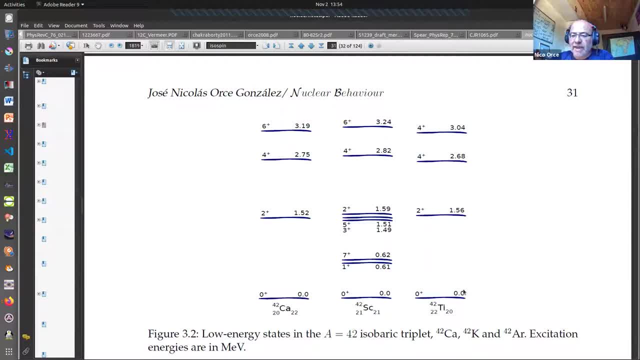 basically we have zero. there's no zero energy. This is the binding energy as a reference zero. So 1.56 MeV above the binding energy, above the zero, the ground state. four, four, six, six. 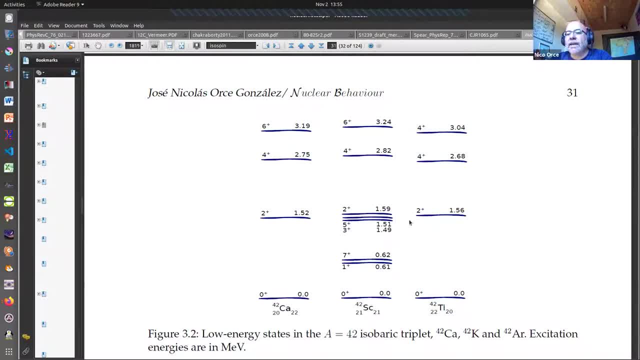 This should be a six as well, So you can see the energies. the levels are quite similar. So you see here and here, Or two different nuclei, we see that they are very similar. So you can see what we are doing. 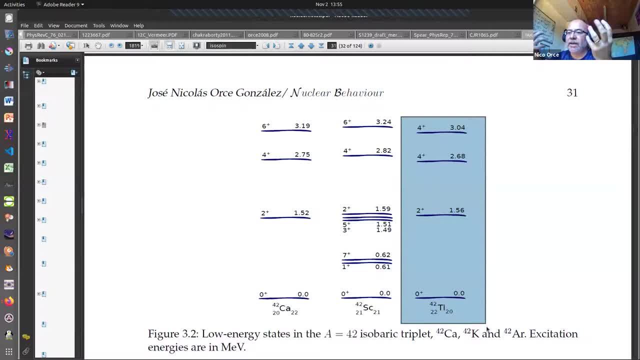 here how the protons are and the two neutrons are aligned with each other. So we see that the two protons here are pointing up and down. In these particular states the two neutrons are pointing up and down, And you can see. 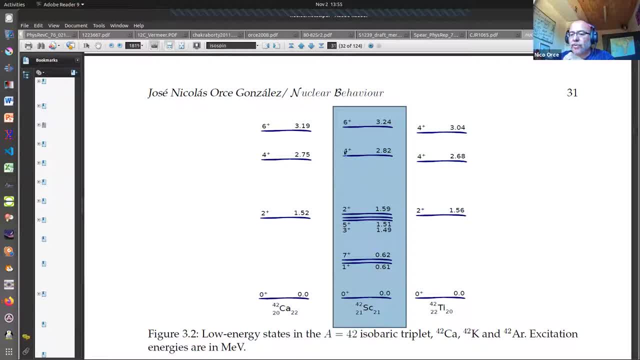 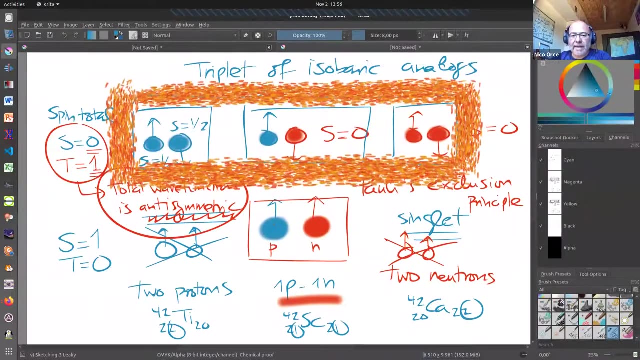 here in the third one, in the titanium 42, that we also have one proton and one neutron aligned up and down. So you see, and we know here that we have proton and neutrons, two proton, one proton and one neutron. 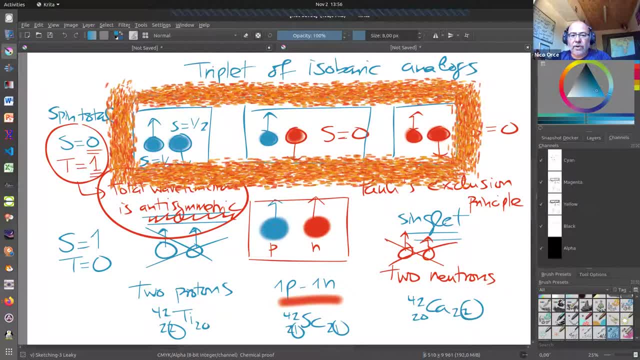 aligned up and down. So I want you to see the similar picture here. These three guys, these three guys. this guy is the titanium 42 with the two protons pointing up and down. This guy is the titanium 42 with the two. 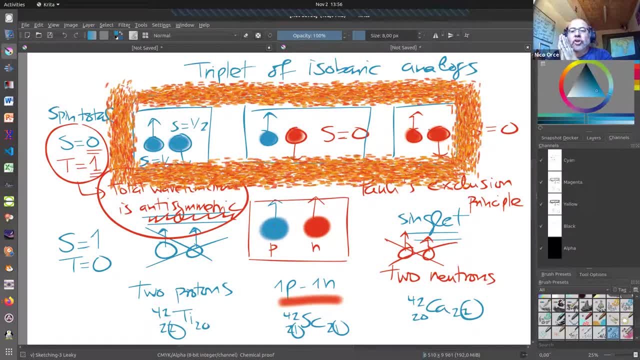 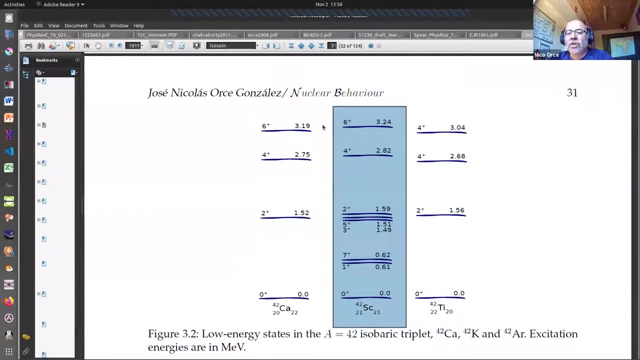 neutrons pointing up and down, Right. So it is actually quite beautiful And I want you to emphasize. think about that. when we look at how a nucleus gets excited, we can see that simple picture right here. Same number, same number. 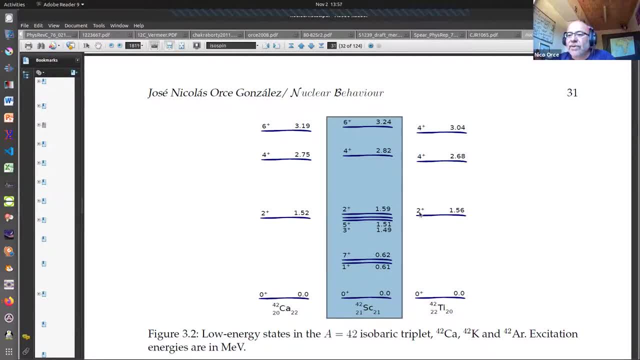 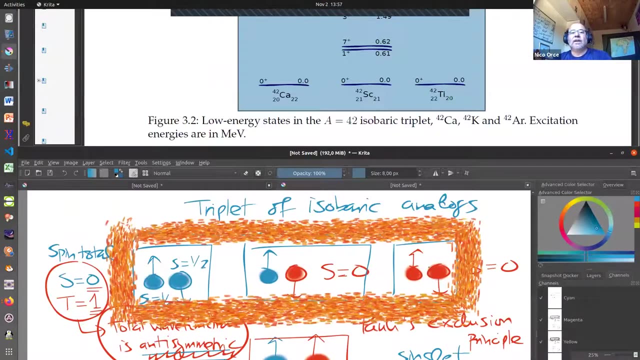 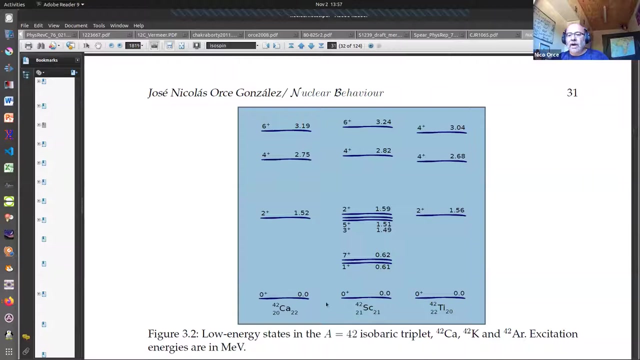 of protons in the nucleus of the nucleus. So this is the six four two zero. This is a pattern which is the beauty of isospin: All these levels have s equal zero. and these six four two zero, They are all t. 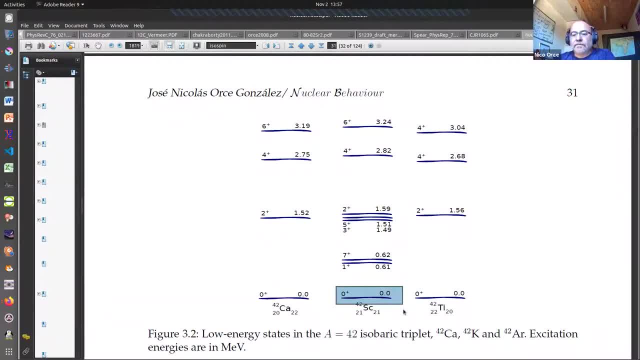 equal one states. Now for this particular guy, for the titanium 42, we have extra levels. We have these guys which are not here or here, right, They are only here. So what is the nucleus doing there? Nucleus? 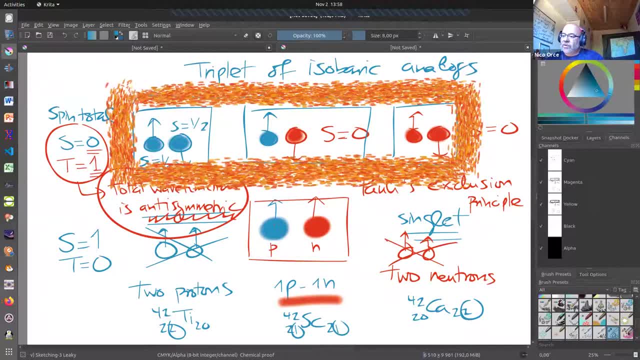 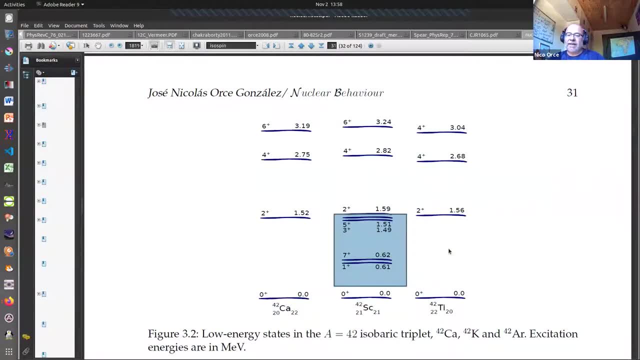 as you can see, here is doing what? How are the protons and neutrons being separated? So this is the nucleus and the neutrons are just between this one and this one, So this one does not have any neutrons, or 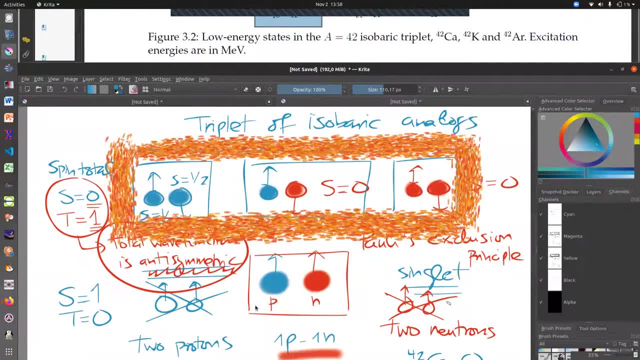 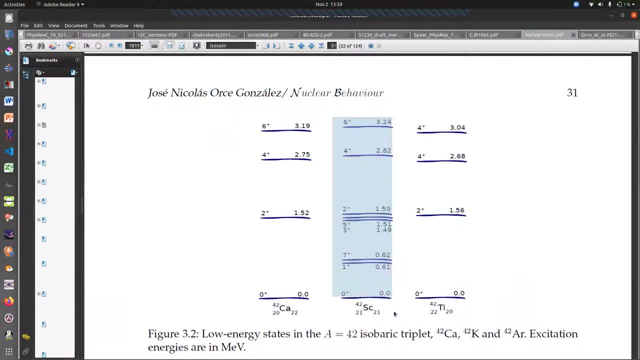 any neutrons. So the second one, for I think the one you got, This one, The second one, The second one, Second one, No, No, in the middle. Yeah, This one you have to be symmetric, This one. 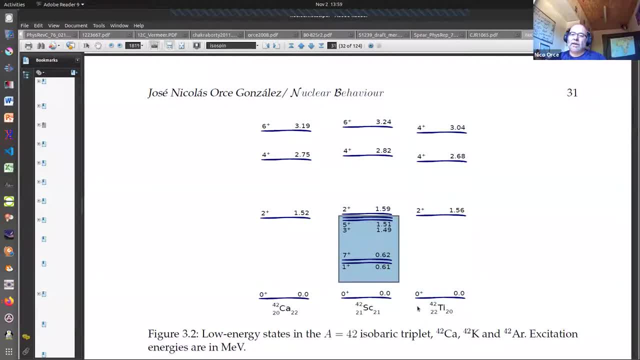 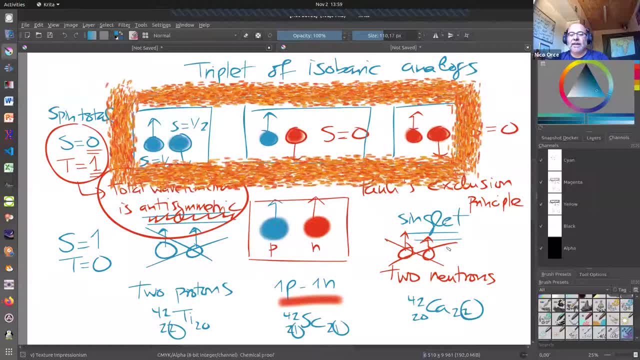 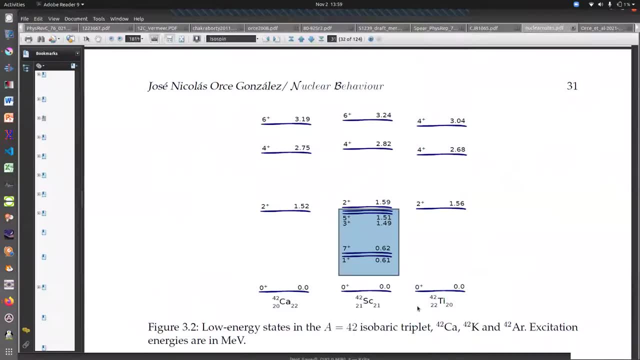 Uh-huh, So in this particular S, equal to one T, equal to zero, right, That's, that's absolutely correct. Uh, Ghaninshuthi, Is that Ghaninshuthi? Yes, So Ghaninshuthi, this is absolutely, absolutely correct, because these guys are not here, or? 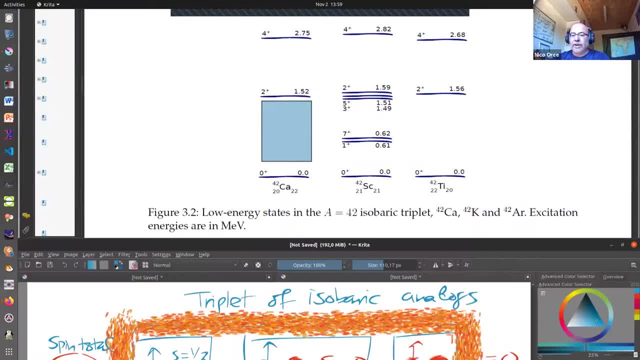 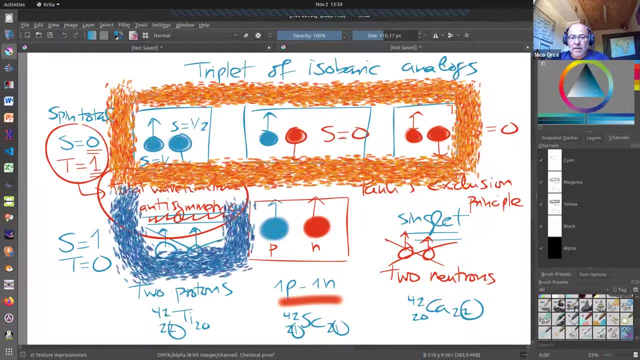 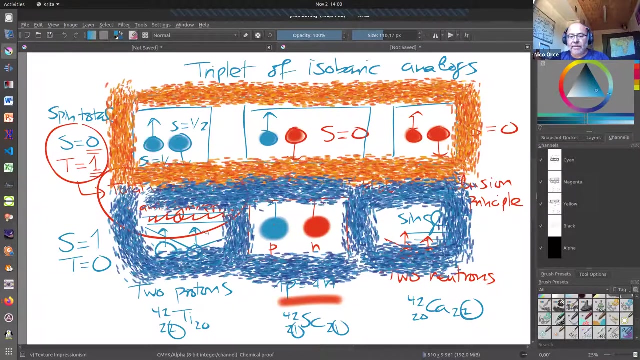 here? Right? I will look at the picture. This: These guys are the only possibilities which are not here, or here, right? These guys that we see for the scandium 42, pointing up proton and neutrons, they're not here and they're not here, right? 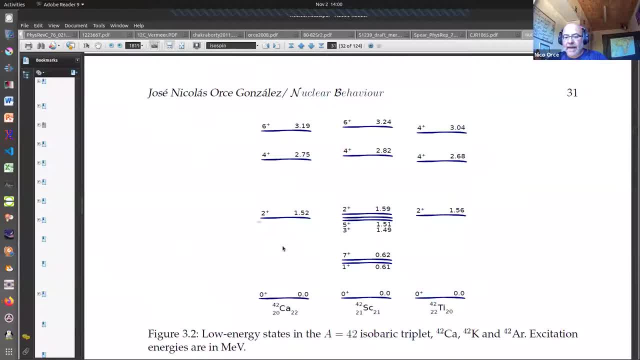 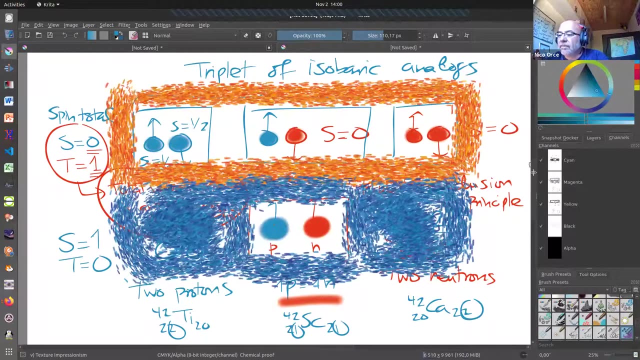 Which implies that we don't see them either here or here. Uh, Ghaninshuthi say, all of these guys are isospin S equal to one pointing up and um T equal to zero, right? So these guys that pointing up because they can do so, because they are not the same particle. 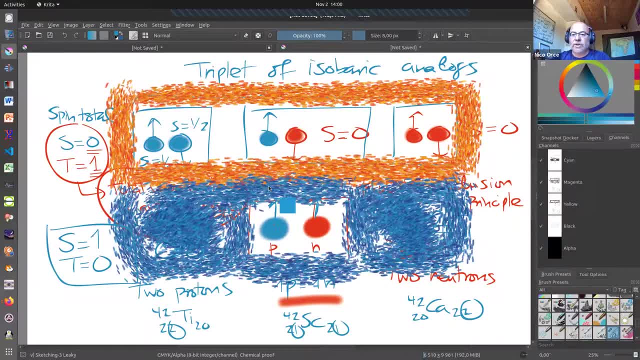 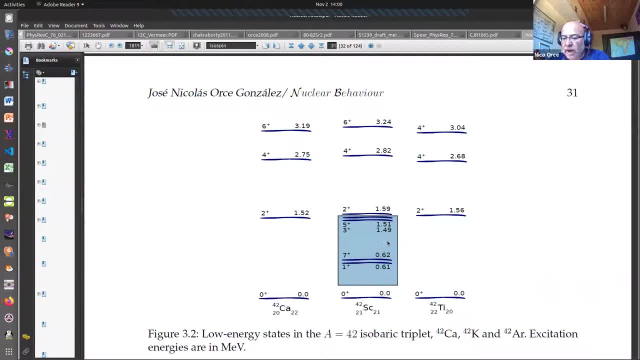 and these states Right, As you see here, they are all T equal to zero, S equal to one. These are the guys. all of them are T equal S equal to zero, T equal to one, S equal to zero, T equal to one right. 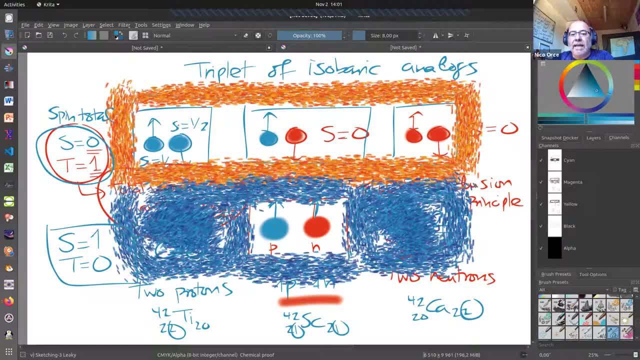 We are in this particular case And because the same, we have the same possibilities for the two protons, the proton and neutron, and the two neutrons, to say exactly the same, these guys actually, uh, beautifully represented in titanium 42.. 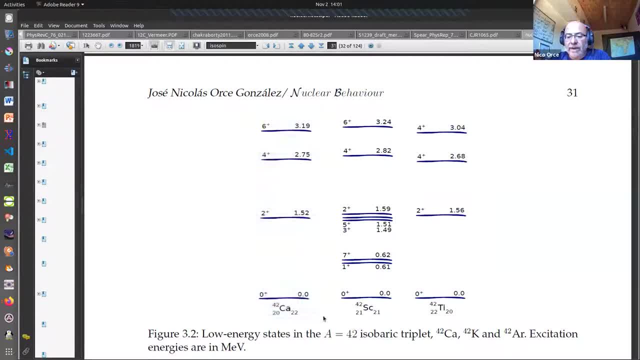 Again, this is a six plus here we have in calcium 42, and also we have the six, four and two in scandium 42, plus the zero plus Right, Whereas these guys is the only guy who has these guys, this, uh, one plus seven plus. 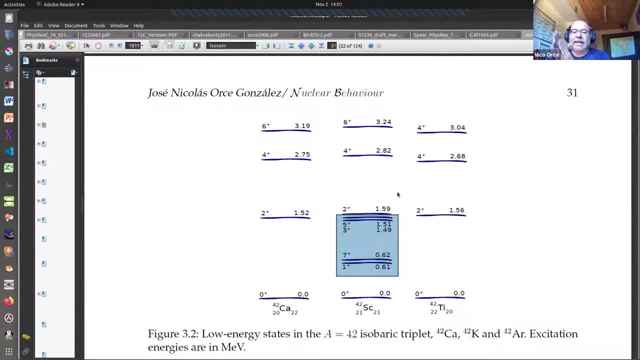 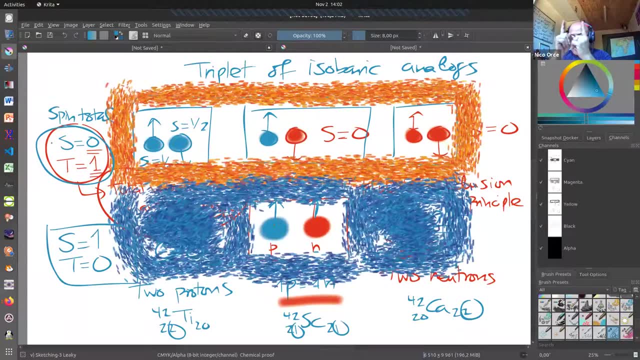 three plus five, plus excitations. and these excitations, they are characterized by having proton and neutrons, one proton and one neutron, pointing up to total isospin. one and T must be equal to zero there, you know, to fulfill the properties of uh- anti-symmetric wave. 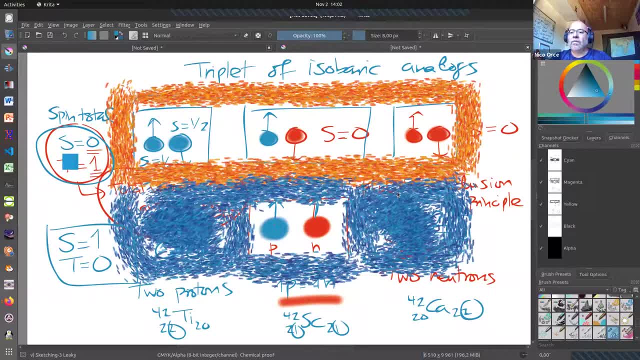 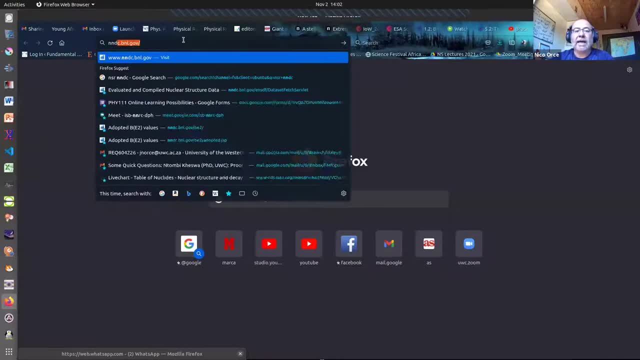 function Okay. So now, now is a good time to go to the NNDC, to go to the NNDC and say, okay, uh, let's investigate the situation a little bit farther and let's go to another triplet of isobaric. 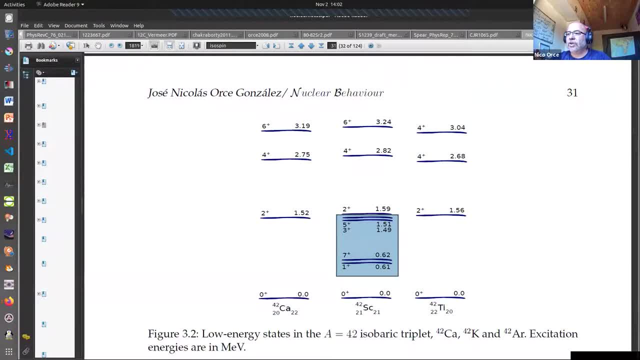 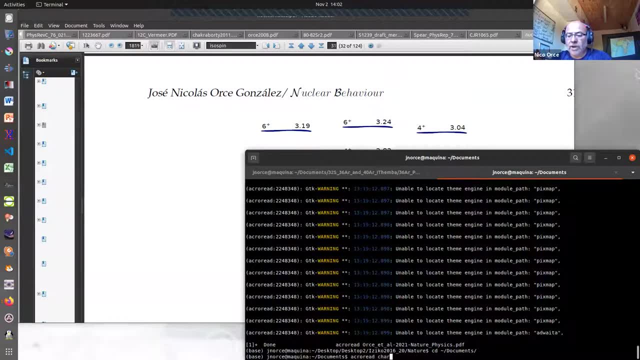 analogs. We can take, uh, the charts of nuclei. uh, right here, uh, I could have read um sharp. Uh we can say, okay, let's do, Uh, let's investigate this chart here. 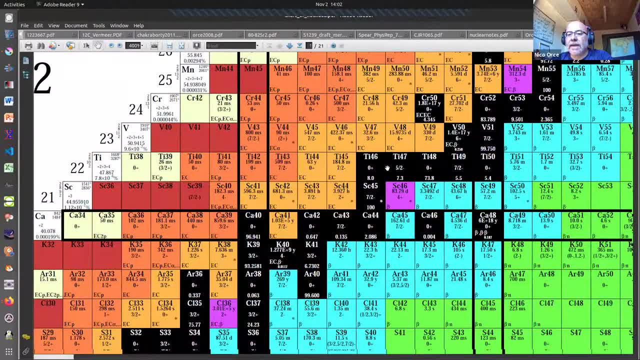 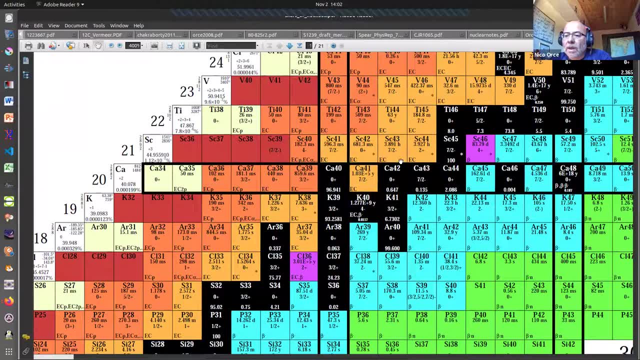 Uh, we were on the calcium 42, scandium 42, titanium 42.. You see these guys here, but we can do the same thing. if we do. uh, let me see here, For instance, Krypton 38, calcium 38 and argon 38, they will be again. 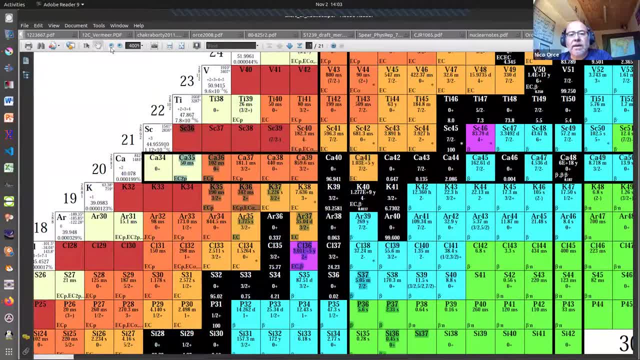 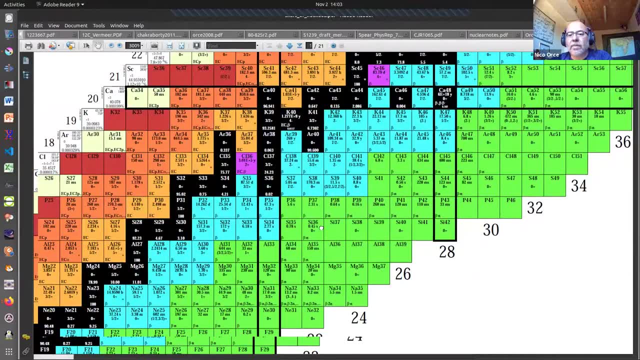 Let me see: Uh, let me go right here. Uh, let me see, I want to move it. Uh, I'm not holding it with this. Let me see, Here we go. So we have another situation where we can have: uh, let me see 19 and 19.. 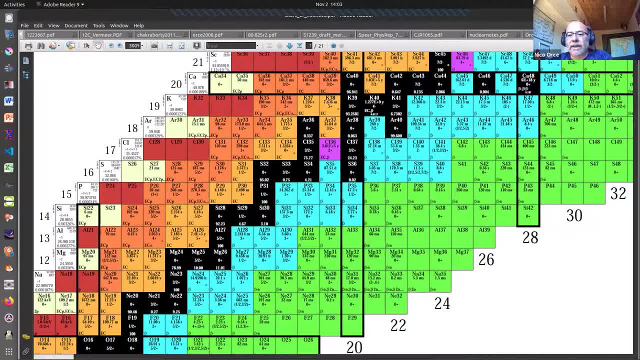 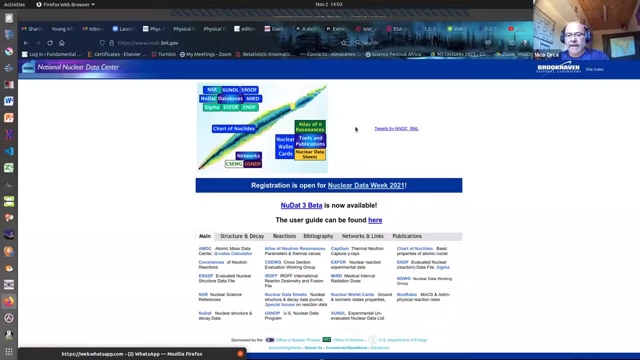 That's calcium, potassium 38. Then we have 20 and 18, and we have, uh, 18 and 20.. Okay, So we can have another possibility and we investigate. Now we investigate ourselves and say, okay, I want to explore this far. 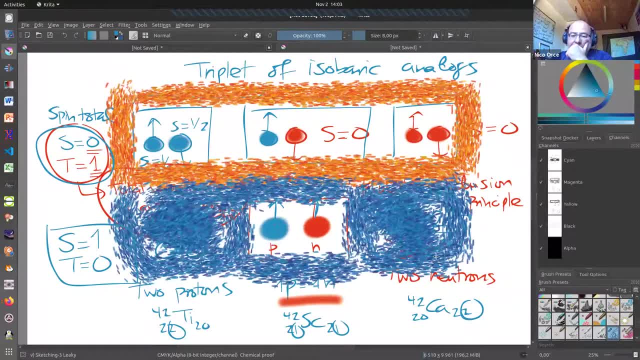 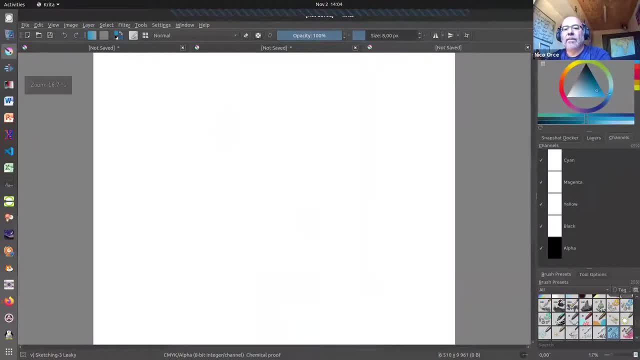 And I want to, uh, to look, this is an exercise for you to do for, for for next Friday. I want to look at these fellows: 38 potassium. Then we have, uh, we say we have 38 potassium. 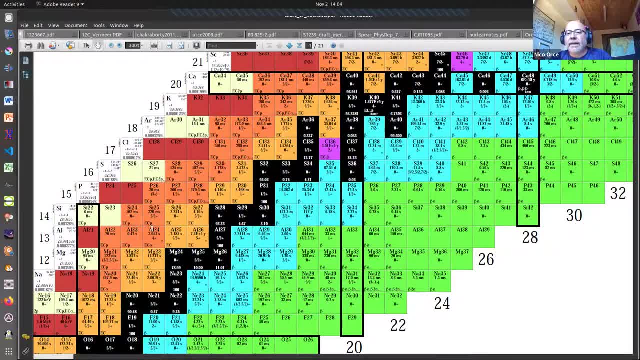 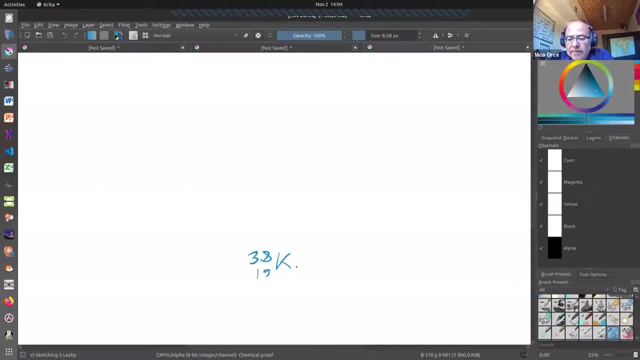 Then we have argon 38,, argon 38, and calcium 38. So this has uh, 19 and 19.. Then 38, calcium, which has 20 and 18.. And here we have argon 38,, which has 18 and 20.. 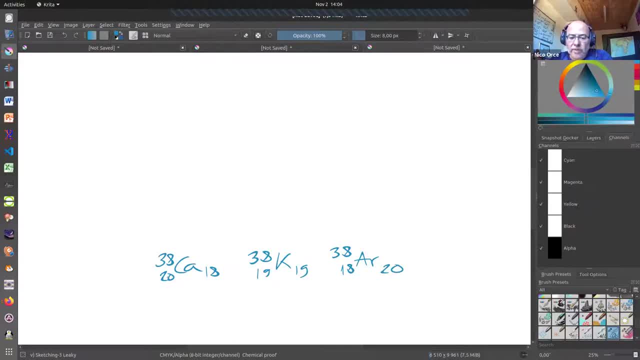 Again, Again. We are going to assume that the extra both of them has 18,, 18,, 18,, 18, 18 and we have extra. here We have extra, uh, two neutrons. right here We have extra two protons and here we have an extra one proton and one neutron. 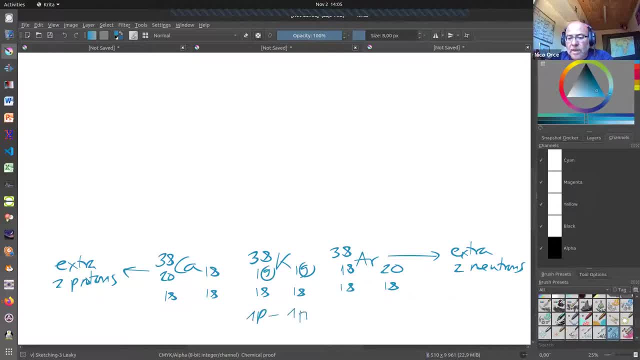 Okay, and one neutron, right, and we're going to apply the same thing and we're going to build the level scheme for these guys. we're going to build the level scheme and this is going to be our zero, but i don't want to say anything. we're going to go to the nndc. 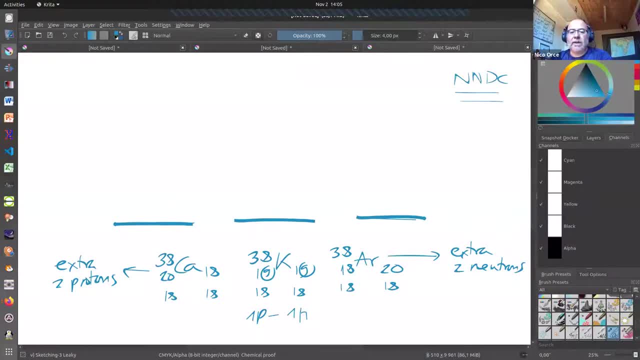 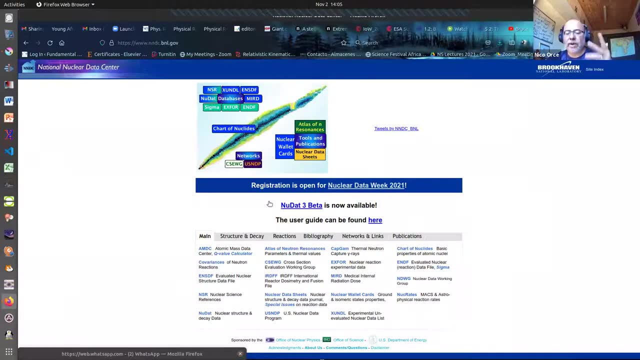 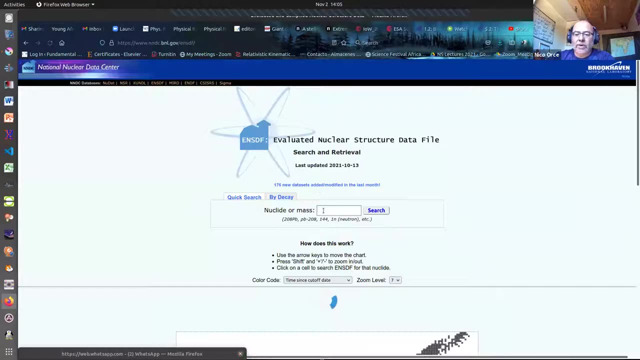 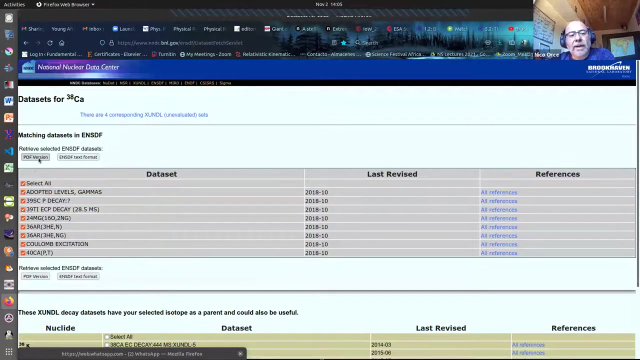 and we're going to go to calcium 38, and there we're going to go to the ensdf. ensdf: that's the evaluation of data, that's the data which has been evaluated already. and we go to calcium 38: search, search, select all and make a pdf version. and here we have 20, 38 calcium. 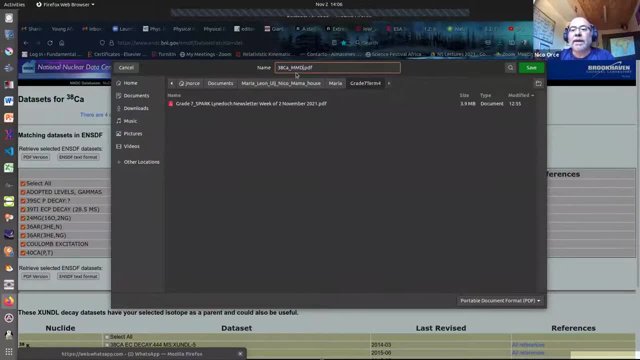 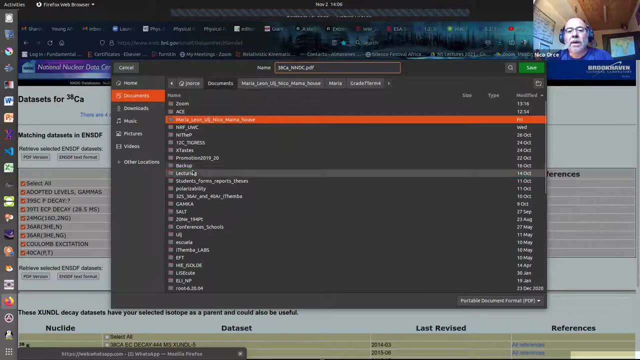 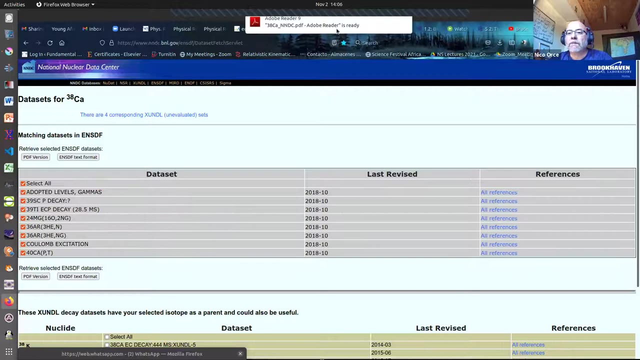 and dc and we put it in documents and we put it in documents and we put it in documents in lecturing nuclear structures, nuclear, in lecturing nuclear structures, nuclear, in lecturing nuclear structures, nuclear structure here, structure here, structure here. we open it up and let's look at what is happening right. 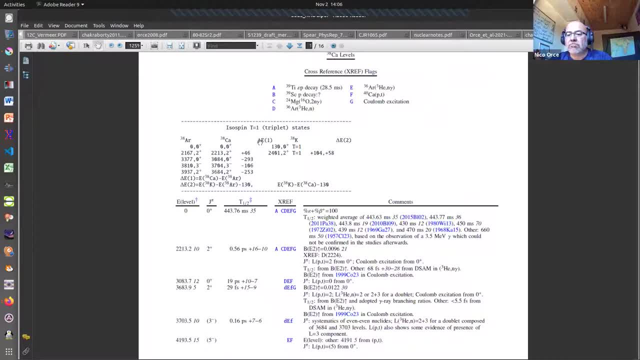 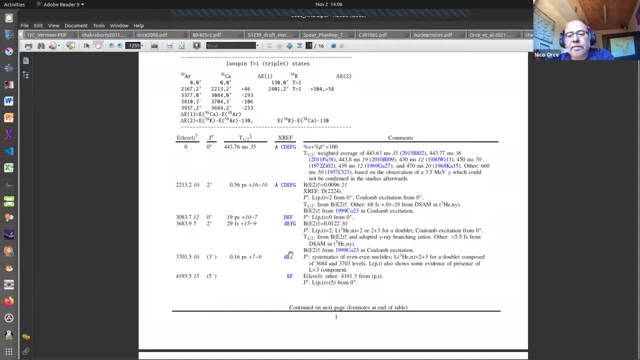 and let's look at what is happening right, and let's look at what is happening right here. okay, so we're going to write down. okay, so, we're going to write down. okay, so, we're going to write down, we're going to write down. uh, we're going to write down, uh. 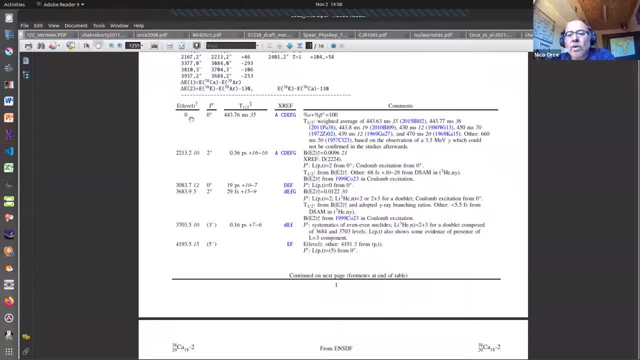 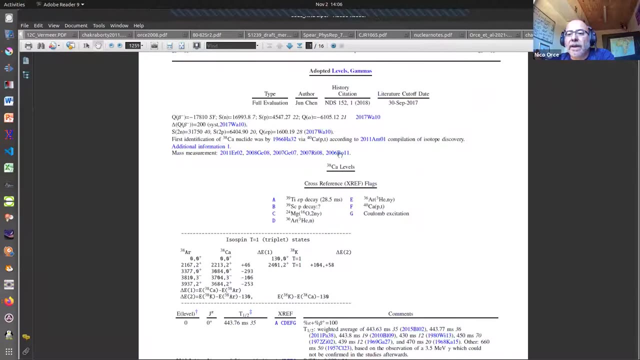 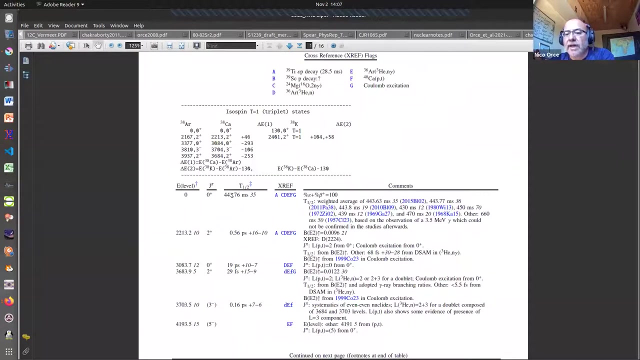 You know we have the zero, we have the two, and this doesn't say anything here about ISSP, But generally when you compile things you also write down the SSP quantum number on the state in particular. So this will be actually t equal one. 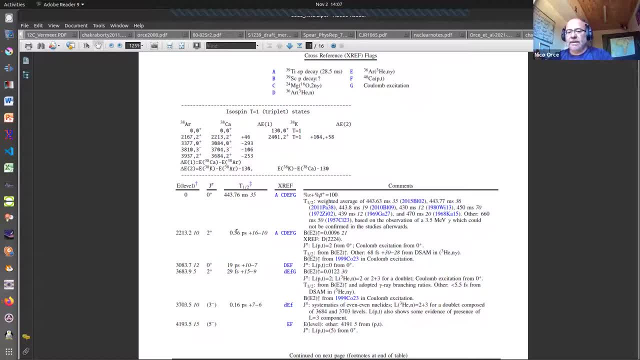 This will also be t equal one, But I'm going to show you just these first two. So this one, the first, this zero plus ground state right, And then the second, the two plus is at two, two, one, three. 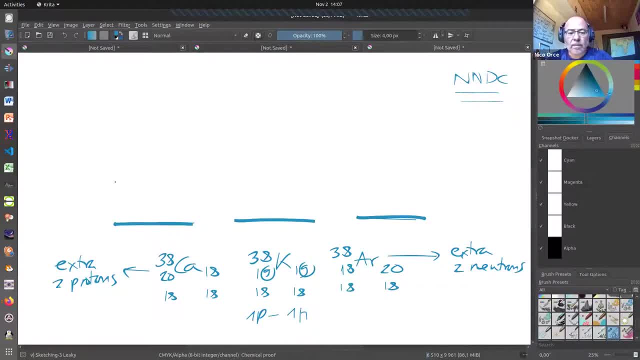 So let's write it down: Two, two, one, three, zero, zero plus. there's a two plus two. two, one, three, The same thing. there will be a two plus here and a two plus there. 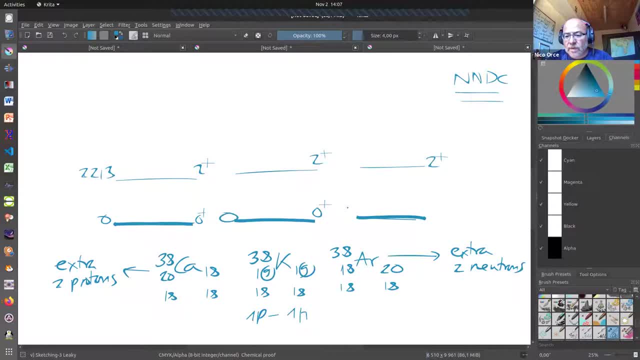 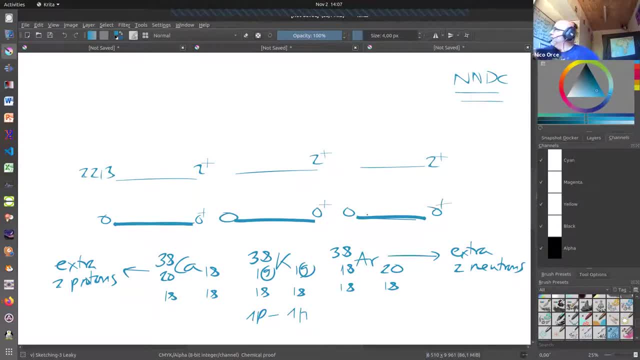 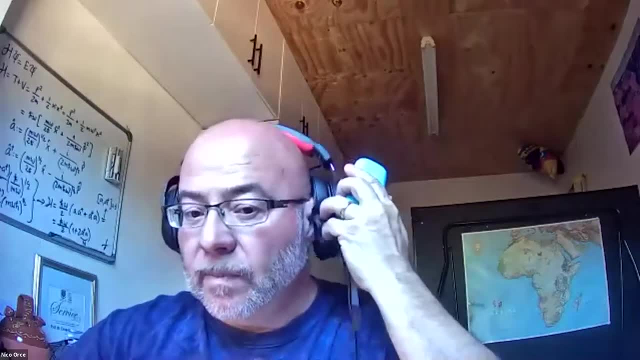 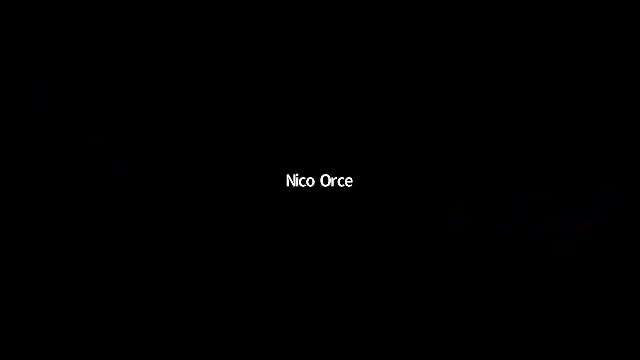 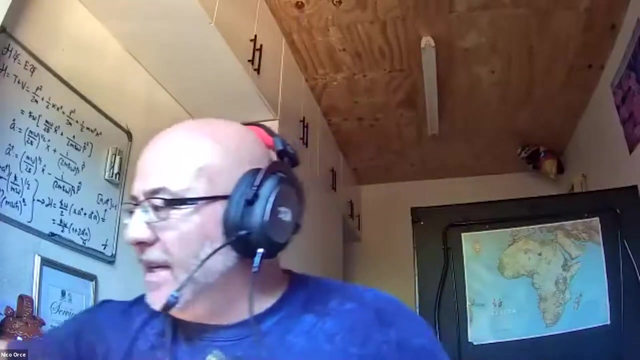 And then we have similar energies: zero plus, zero, zero plus. Excuse me, Let me see I have to pick up this one. you may continue, as prof was saying. hey, all right, sorry guys, i had to to take care of the kids as, uh, my wife is in a field trip. i have to be. 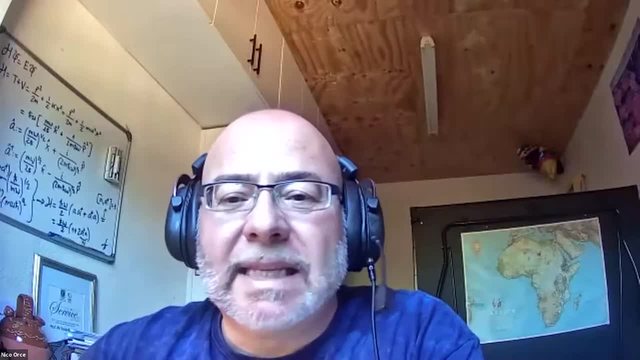 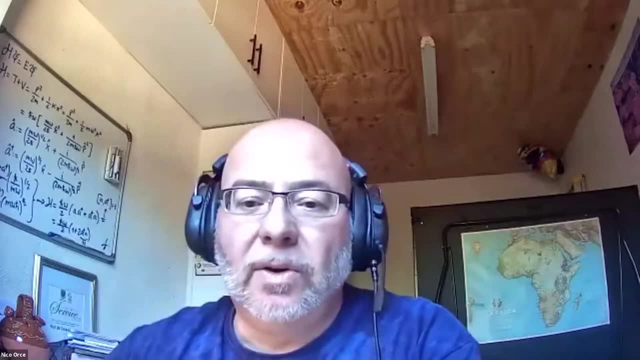 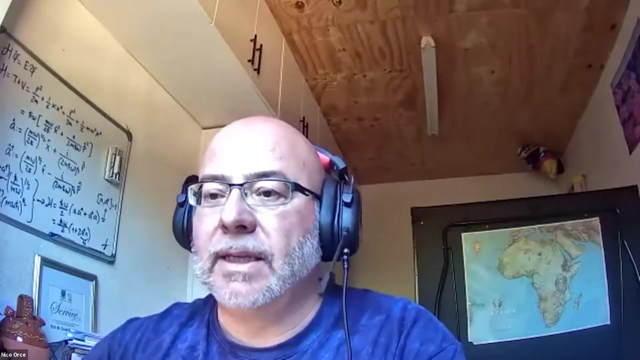 be ready for, for action. something happens. so i was telling you that we have a zero, two plus two plus, two plus and all these guys. you can confirm that on the nndc. so you're going to check. can you please again share the screen, right? uh, let me see that. 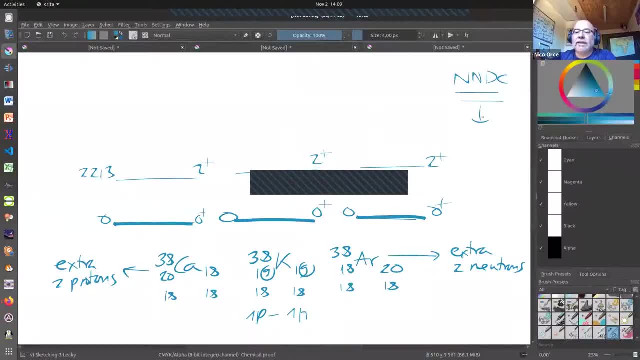 so i am sharing now, so i'm telling you that these guys, these guys will have: uh, this will be t equal one. uh, let me see, let's move this up here- this will also be t equal one. these will be t equal one because they are the same: t equal one, t equal one, t equal one. so we are assigning, assigning. 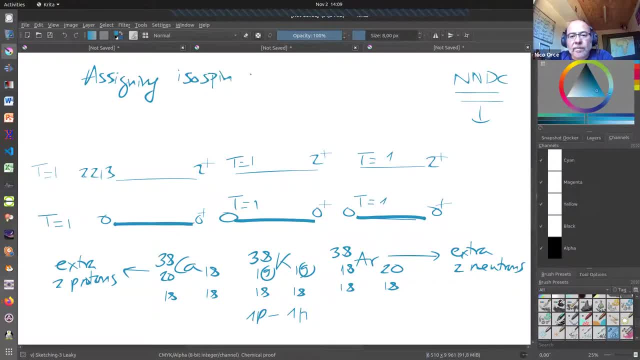 as a spin. quantum numbers, quantum numbers to all two states. so excitation, right. so excited, excited, excited levels and we will have anything which is similar, is the same, about the same energy. the energy will may change a little bit here and there, but every level which is the same would be t equal one. 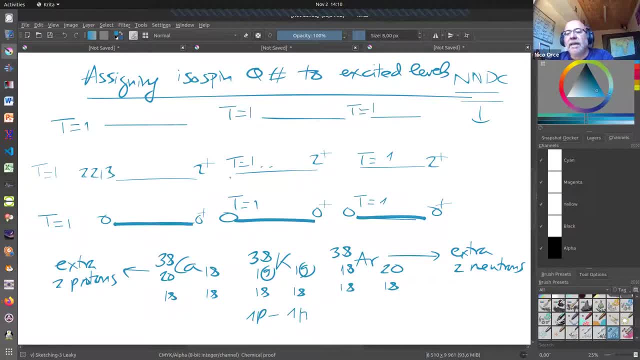 t equal one, t equal one. but there will be levels- and this is what i want you to investigate here, in particular in the, in the, in the potassium 38, which will be different and they will. they won't be here right here, they won't be- and those levels they will be obviously t equal zero and in the t equals zero. we know that. 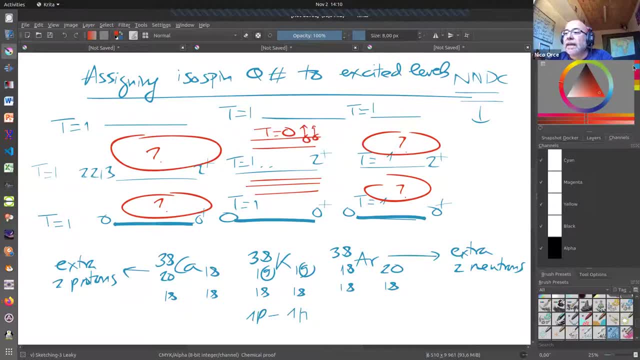 the spins, the will be pointing up in the t equal one. we know that the spins will be pointing up, are pointing up and down. So you see, without looking at the nucleus, we know by measuring the properties and looking at the similar levels, you know that at this triplet of isobaric analogs, 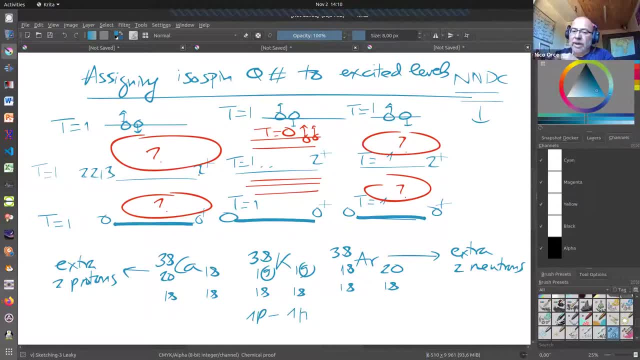 that we have described before, we can assign S-Sping quantum numbers to those levels which are equal to each other. You know, by measuring the spin and parity, two plus the zero plus, there will be a four plus here, four plus here, which will be the same, you know. 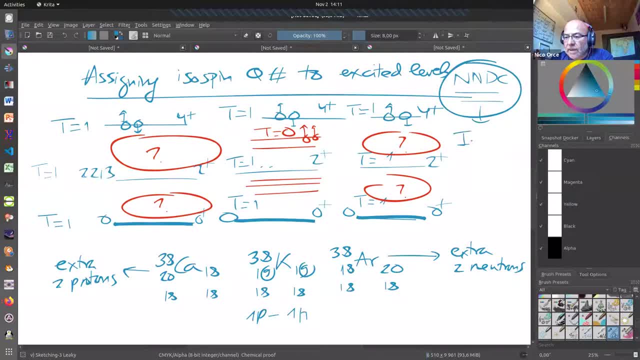 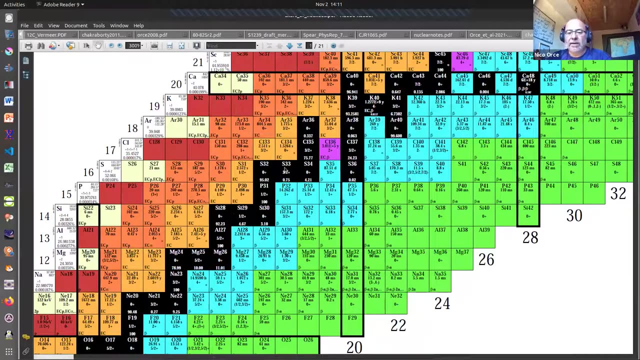 I want you to go to the NNDC and investigate, Investigate, and each one I want to investigate for different nuclei. You can go to the chart of nuclei here, the charts of nuclei, and say, okay, I'm going to investigate this. 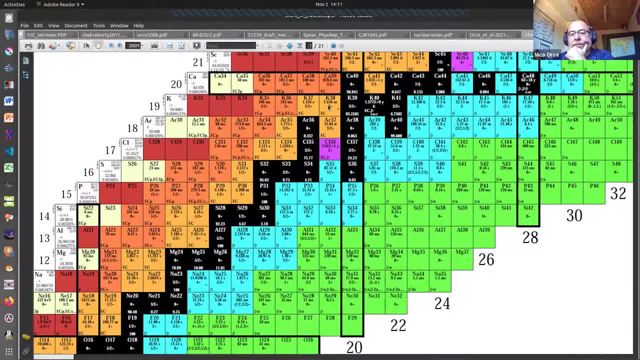 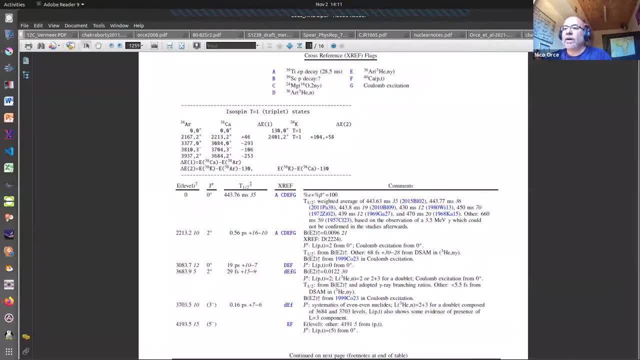 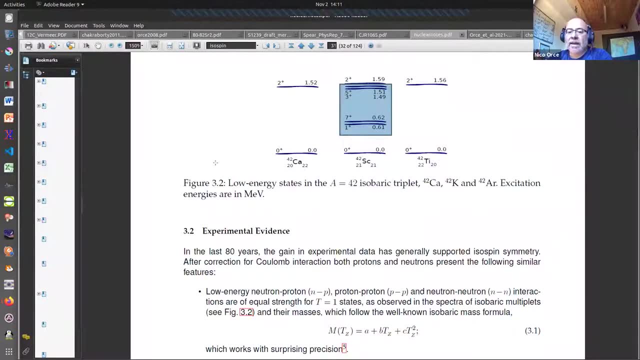 and someone else is going to investigate, for instance the. actually there's a paper, a paper here in the lecture notes. I wrote a very nice paper one time on S-Sping, S-Sping purity, on the charge: independence of these fellows. 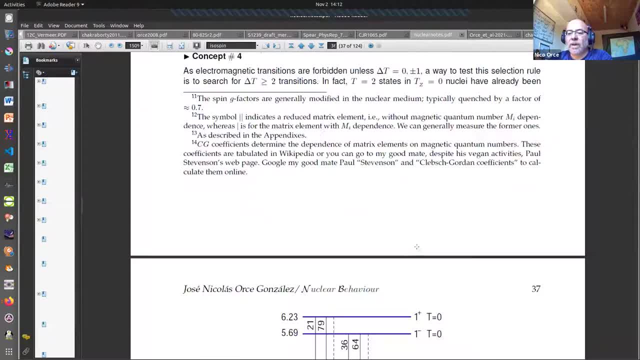 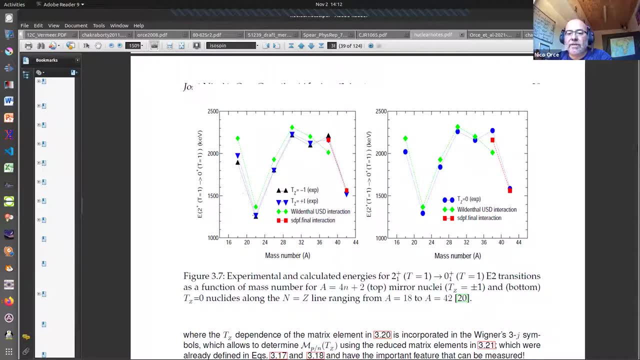 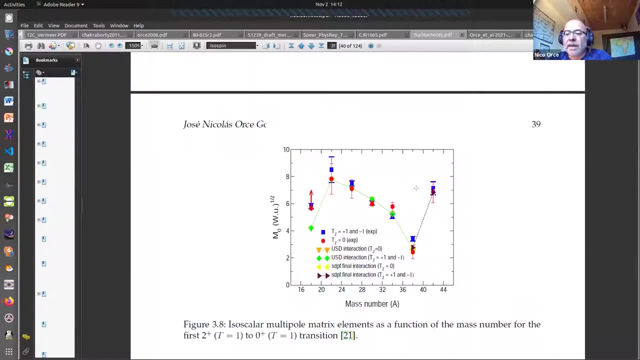 So at the end of this chapter I mentioned this paper And you have here the different triplets of esoteric analogs and different properties: electromagnetic properties, energies and electromagnetic properties down here, And I'm telling the 38, but also the 34 triplet. 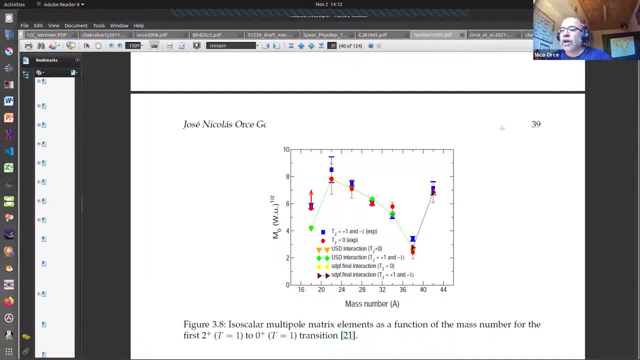 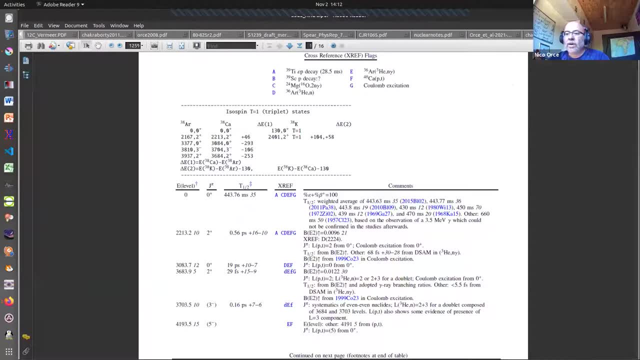 there's a 28 triplet. So if we go to the chart, someone can try the the 30, 34, so 30 would be silicon, 30, 10.. entonces, 30 operatores y 30, 20 de la уровeno de hexahébraize de hotspot y 10 de colorBoxe. 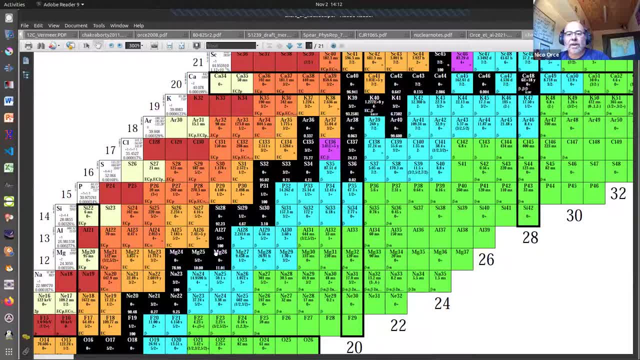 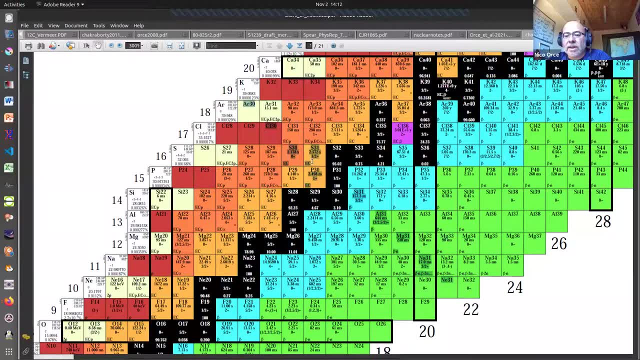 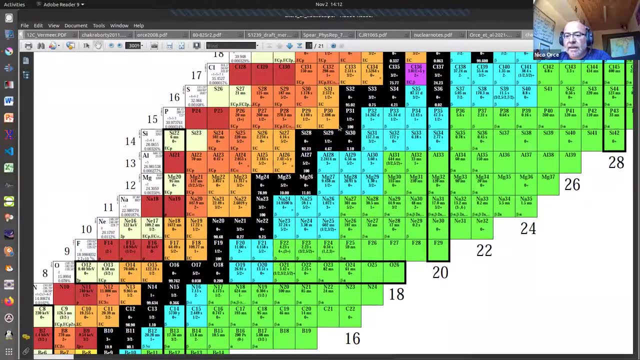 phosphorus 30. Basically, it's always the same. You need to find one which has, let me see, 30 is here, So that will be 15, phosphorus 30 and 15.. That will be the two possibilities, right? And then you have sulfur 30,, which is 16 and 14.. Let me see. 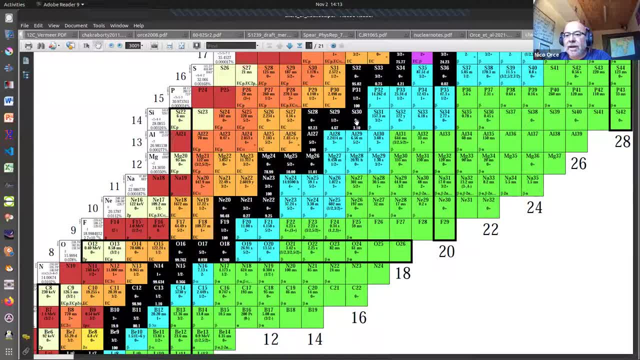 the 14 is here, right, And you will have another one. the third one will be silicon 30,, which has 14 and 16,, right? So the three of them. the three of them, the phosphorus 30, that will be 15 and 15, one proton, one neutron, all of them will have 14,. 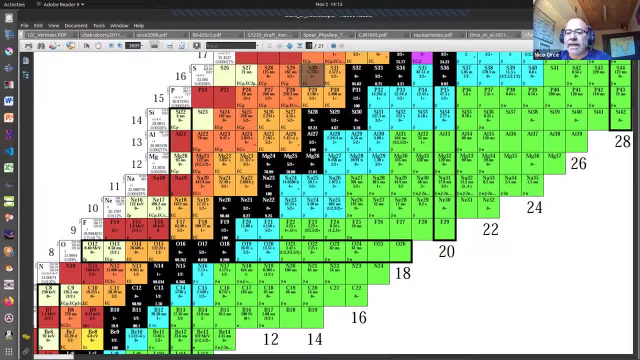 right, 14, and this will be 16 and 14.. So this will have two extra protons, And the third one will be this guy here, silicon 30,, which will have two extra neutrons. These are the neutron numbers here. So this is another triplet. So I want you to. 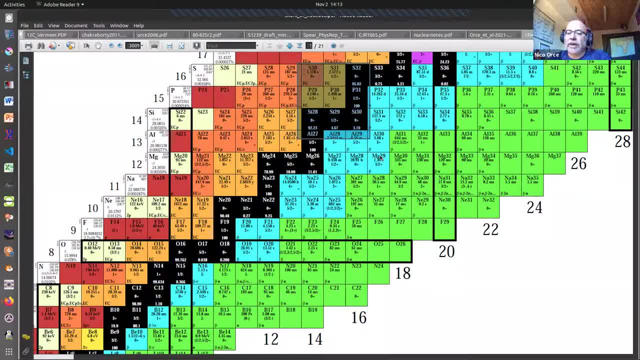 come with different triplets. I don't want you to come with the same triplet and everyone doing the same job. Another possibility is here: sodium 22,, 11,, 11.. Then you have magnesium 22,, which is 12,. 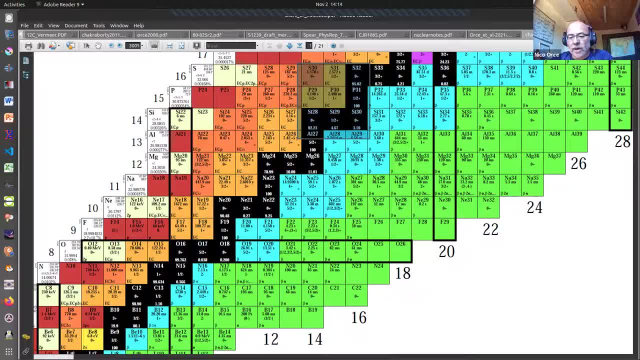 10.. And you have neon 22,, which is 10,, 12,, right? There's another possibility. Another possibility is here: 13,, 13.. And then you have 14,, 12, and 12,, 14.. This triplet here, right? So basically, you find yourself, your. 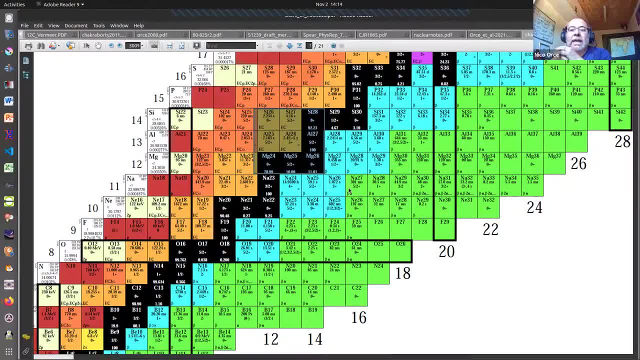 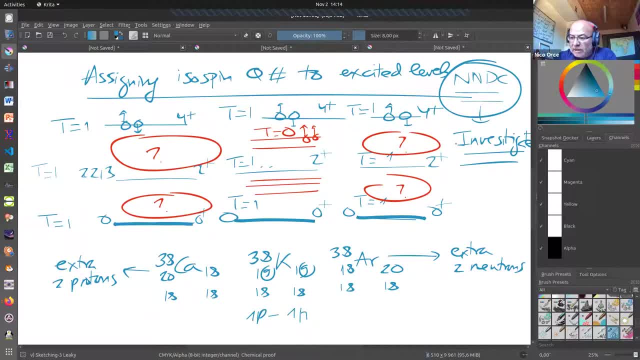 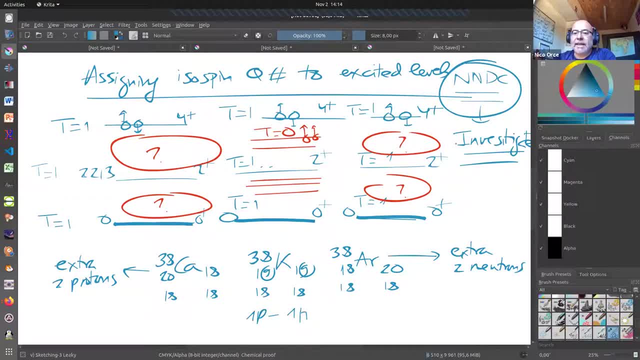 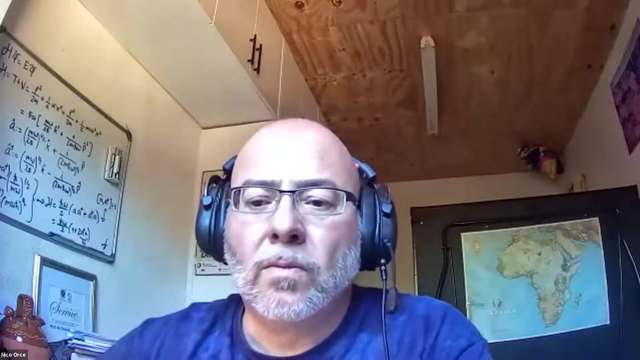 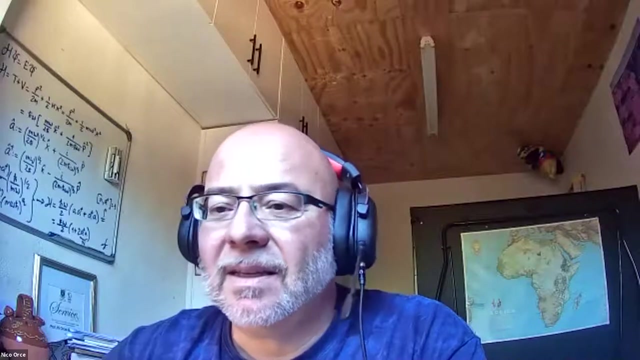 like this with you know exact energies here. you know whatever is the energy here- two, two, one, five, whatever it is energies here- and then assign them an ssping quantum number to each of the levels. is that clear, do i see? uh, no, prof, there is a problem here. from using this example, you give us for potassium, calcium and 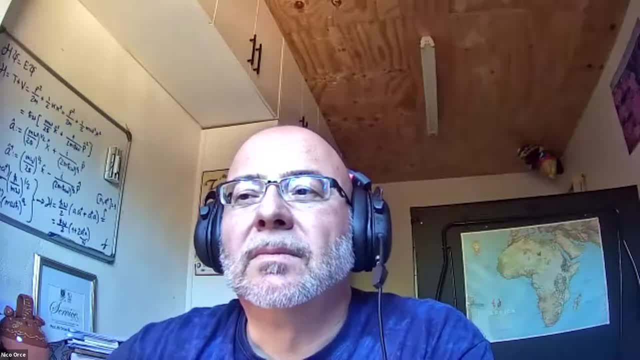 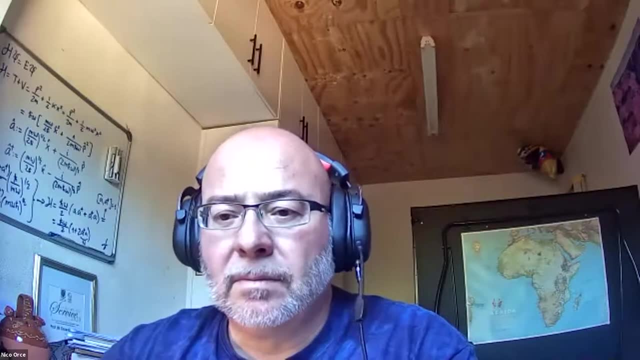 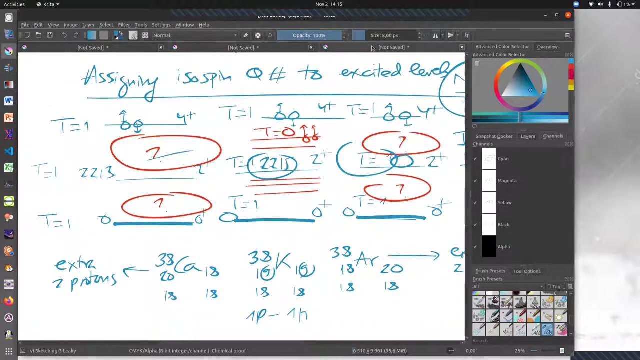 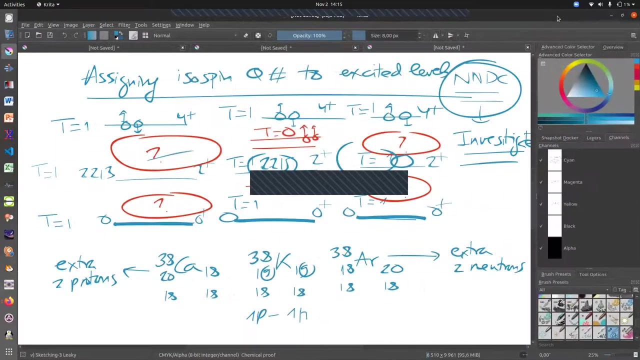 agro. uh, and if you go back to the sketch you will provide, you seem that, uh, potassium is only good. uh, yeah, the second one in the middle is only the one who t is supposed to be. uh, yeah, which one? which one all the others are supposed to have uh. 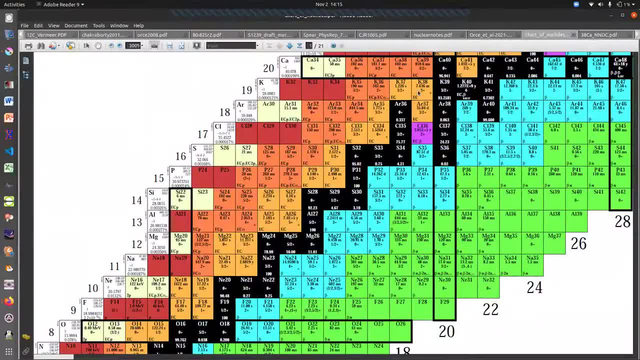 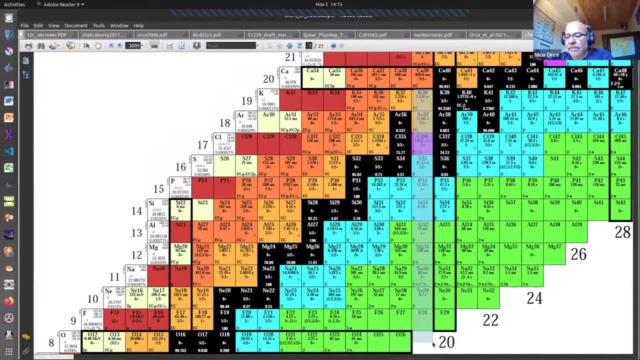 yeah, like which one, which one, 38, but that's okay. okay, but that's a 38 has 19 here and 19 here, right? yeah, so is this one has 20 here and 18 here. so all of them, all of them, they are 38. you see 38, 38 and 38, right. 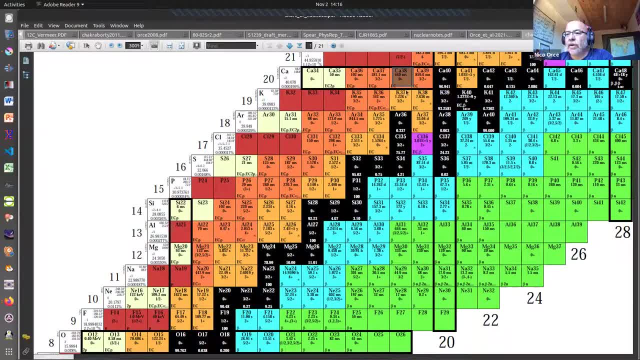 but, and all of them has uh, 20, 18. so all they has 18, 18, 18, 18, 18, 18. so every, each one has a difference of. extra two protons here, one proton. one neutron here. extra two neutrons here: here, one proton. one neutron here. extra two neutrons here, one proton here. extra two neutrons here, one proton. 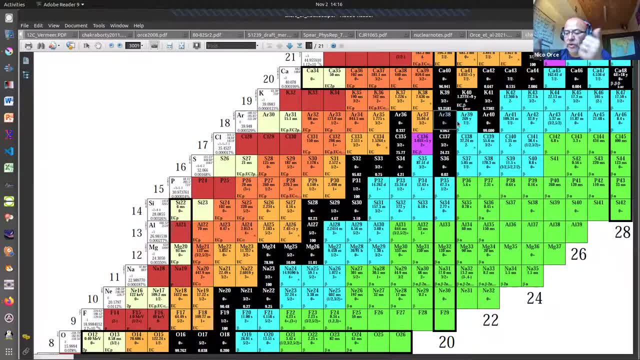 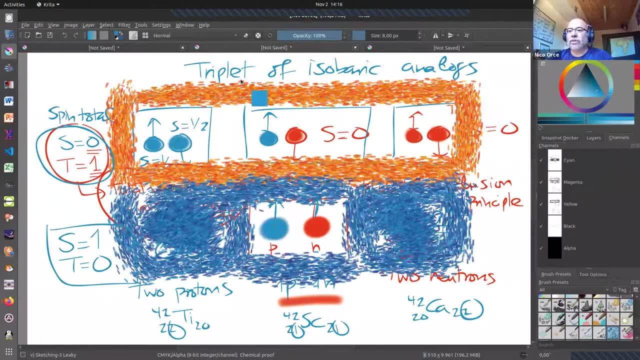 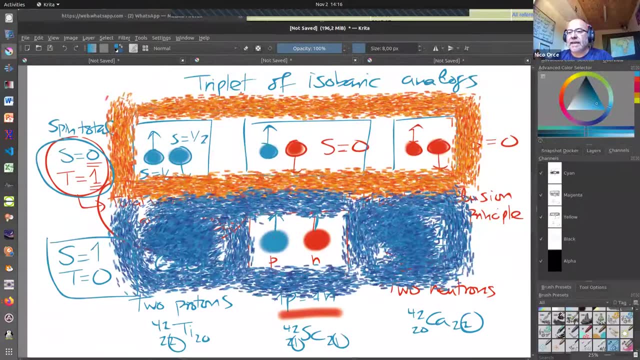 see, they are all exactly the same, but you have either two protons, two neutrons. can i go to the nndc? yeah, you can go to the nndc and check it out. you go to the nndc. this is the. this is what you're going to do. actually, that's the exercise. 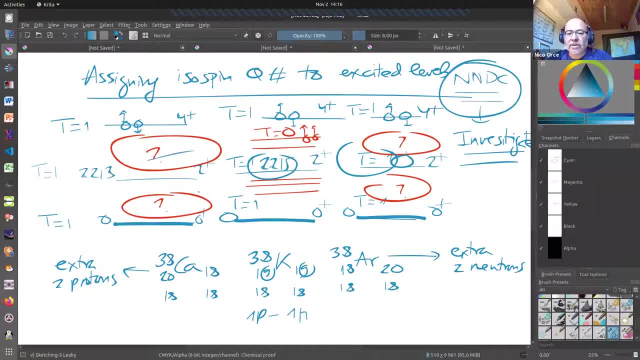 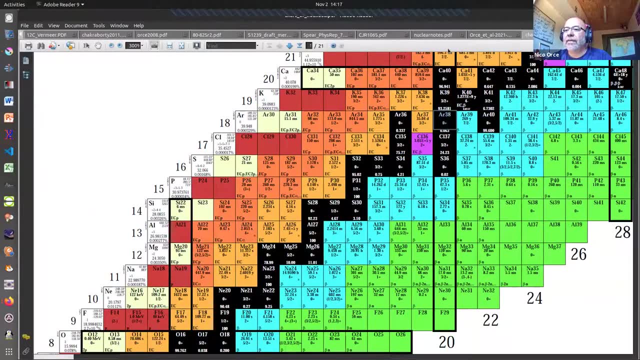 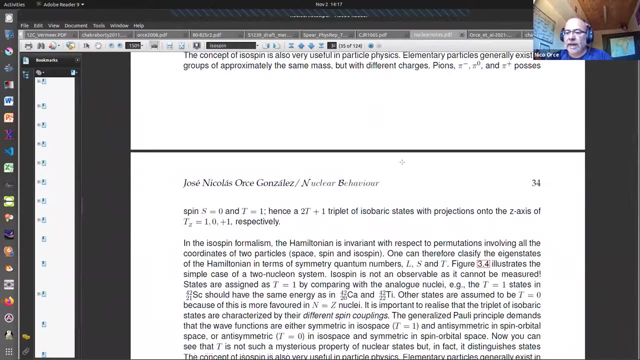 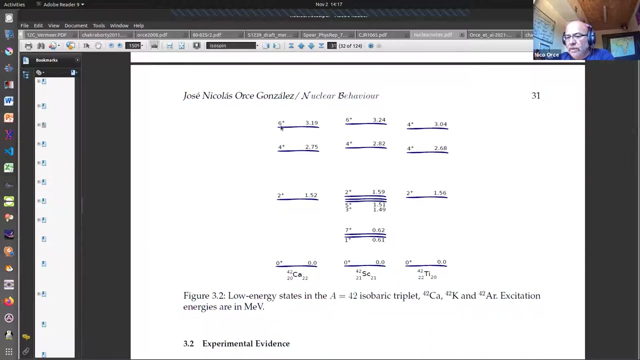 you go to the nndc and investigate yourself. show me this picture here for a different, a different, a different, uh, a different triplet. i show you this triplet. so i want you to go to the nndc and take your time and investigate and tell me assign. these are all we say: t t equal. one s equals zero t equal. 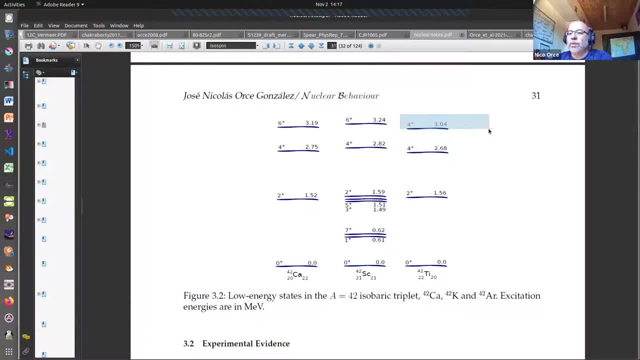 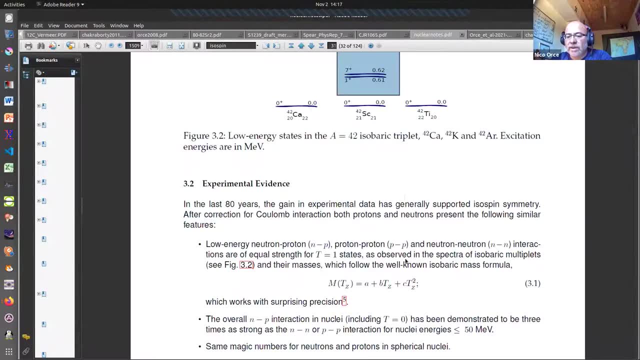 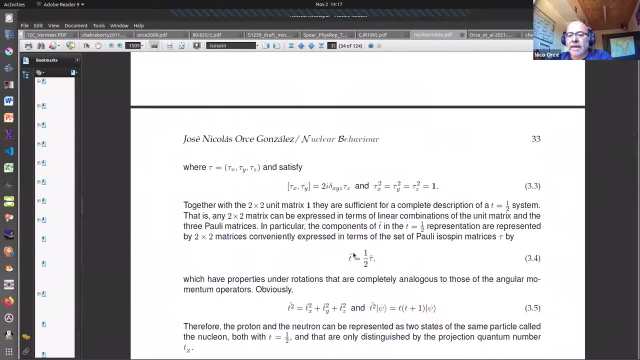 one. t equal one, t equal one. i want you to assign as a spin, quantum numbers to all these levels. right, and all these guys will be: t equals zero. so this is in particular. there's an assignment also here, in the right hand side here, but i'm just telling you the assignment itself. 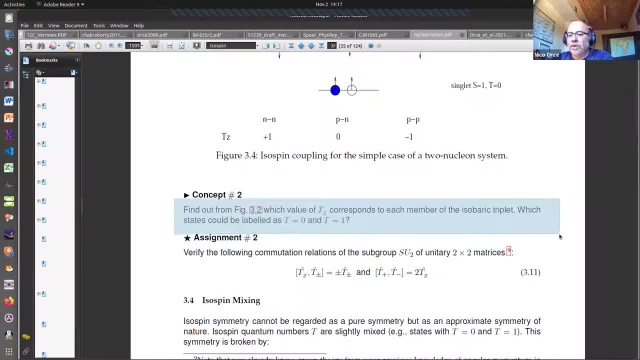 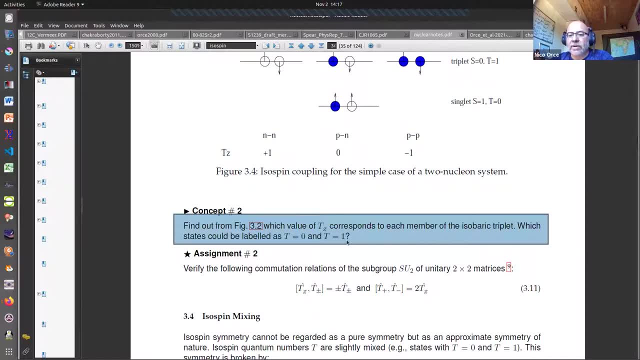 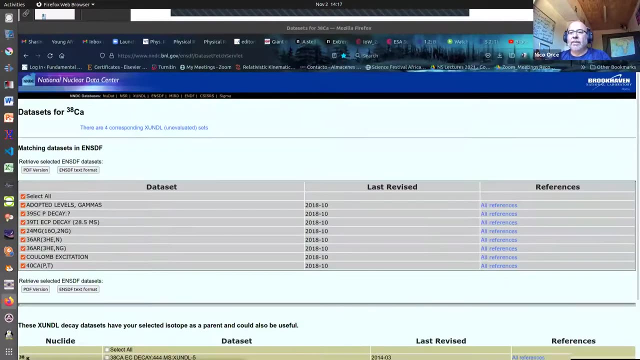 uh-huh. find out from figure 3.2 which value of t cell corresponds to each member of the soviets triplet and which could be uh labeled as t equals zero and t equal one. we haven't introduced this set so far, but this set is simply m minus z divided by two, so this uh nuclei can all just. 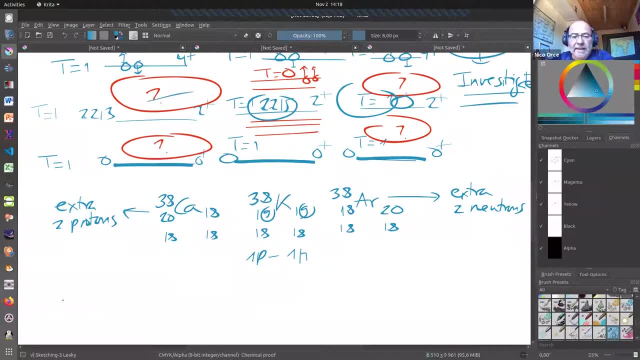 also be labeled as by a tset, quantum number, which is the projection, and this is given by m minus z divided by two, and this tset, this will be minus one. this will be zero because m and z is the same and this will be plus one because n is 20. so 20 minus 18 will be. 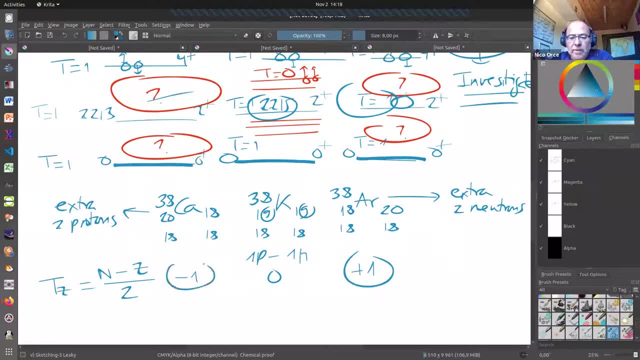 two. two divided by two is equal to one right. this will be minus one and this will be equal to zero. so there's a tset quantum number. so when you say tset is equal to minus one, you refer to this particular nucleus with the extra two, two protons, and when you refer to t zero, you refer to. 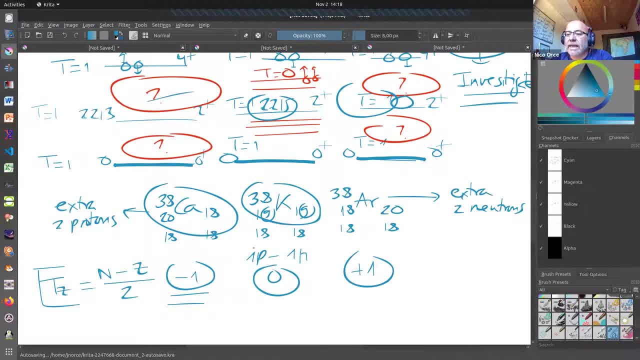 a nucleus, the nucleus with the same, the same number of proton and neutrons. and when you refer to the tset equal to plus one or tc equal to plus one, you refer to the one with extra two neutrons. right, it's just a part of nomenclature and this. 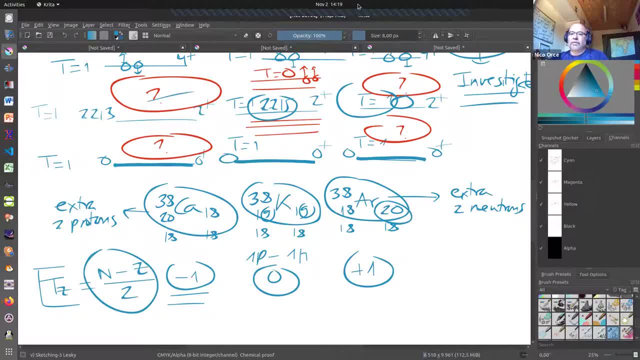 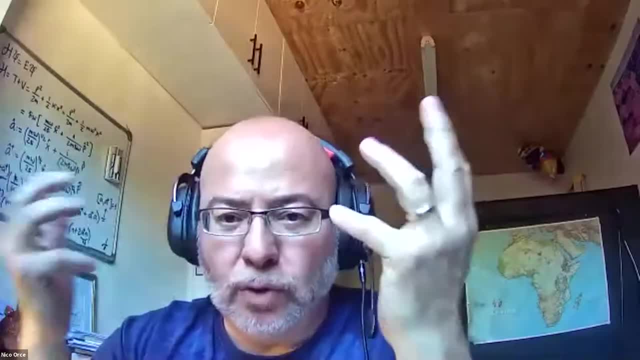 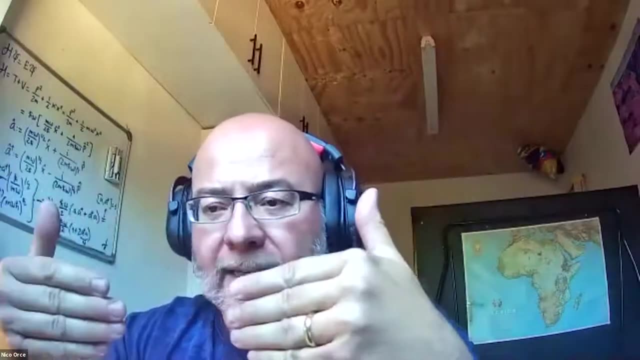 is the definition. there's a definition, okay, so now your job actually to for this to sink in is very clear. you're going to do the same thing. you're going to make your level scheme, you're going to go to the nndc and you're going to look at them and you're going to say, okay. 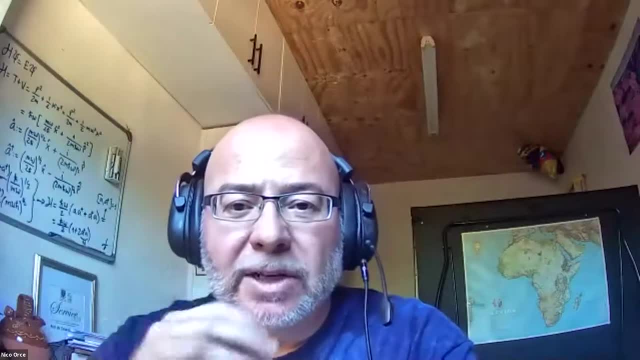 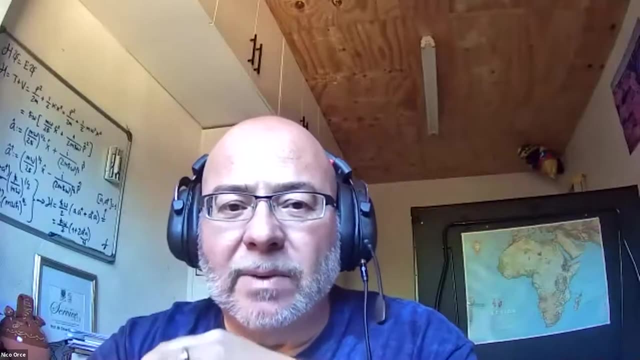 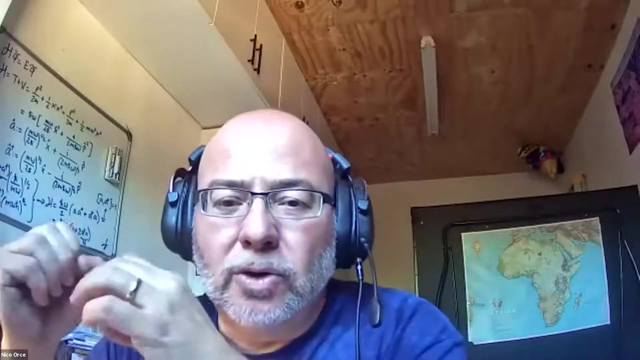 these ones are t equal one. this one at t equals zero. this tc is equal one minus one and zero because of the, or the m minus z, equal to equal divided by two. uh, i want to draw the two uh protons, so the two neutrons, so the two of the proton and neutron, how they are pointing up and down. so 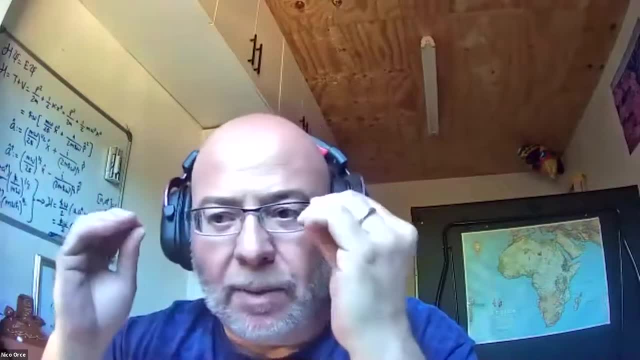 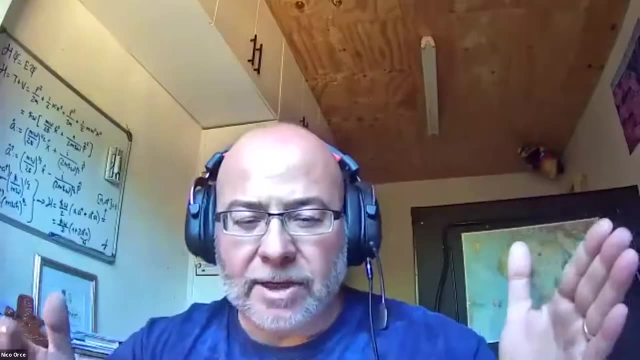 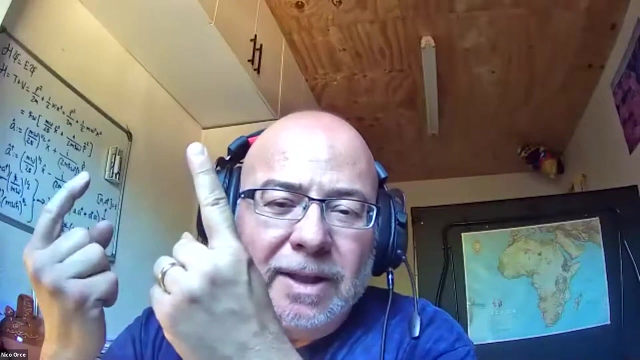 this is the thing, everything i want you to draw in your level scheme. i want you to get the point that you know, by measuring the angular momentum, measuring the energies of this level, the parity, we know how the proton neutrons are pointing. you know the spin quantum number is pointing up or down. 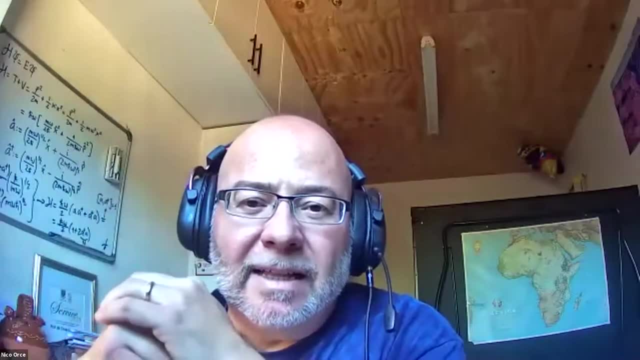 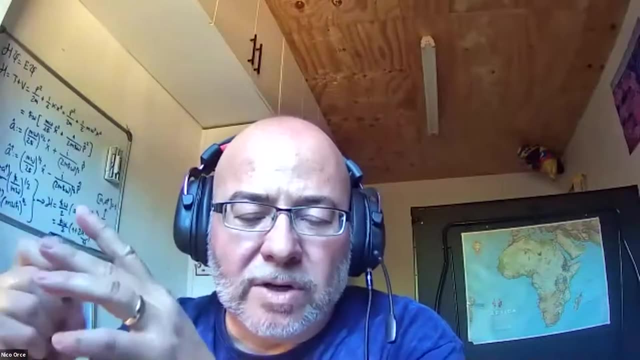 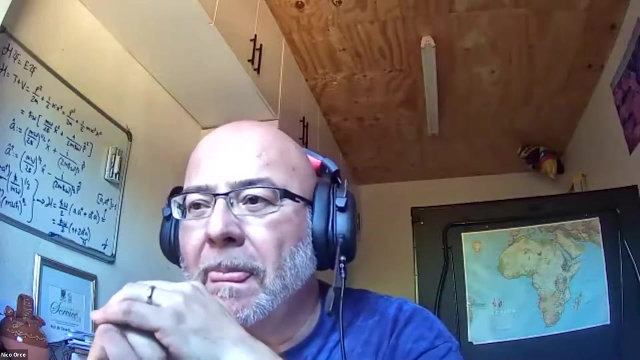 just by seeing, uh, the the the result of isospin symmetry. the charge independence of the nuclear force works very beautifully for something which does not have a spin quantum number. it doesn't exist. all right, this is for today. i want you to explore. now go to the ndc. 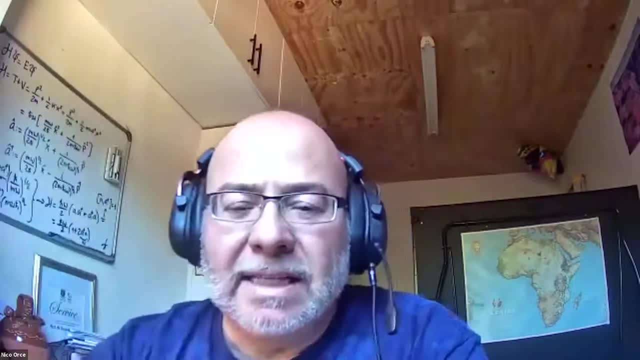 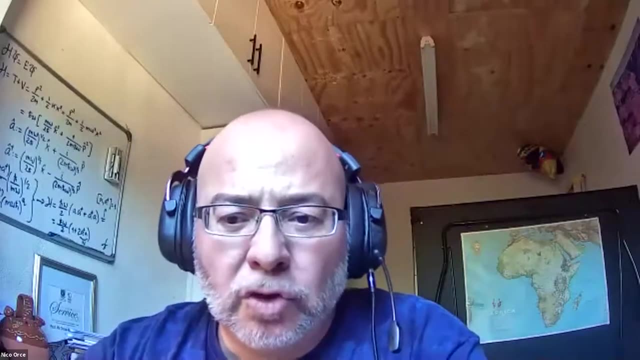 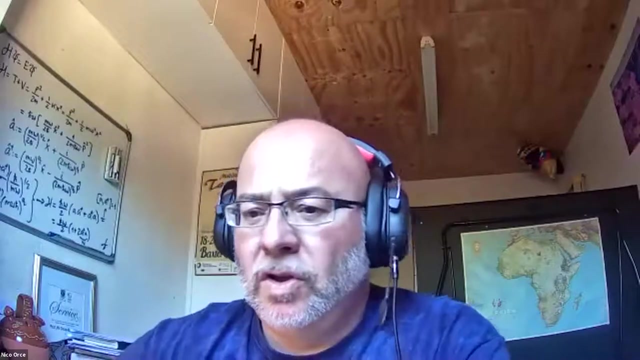 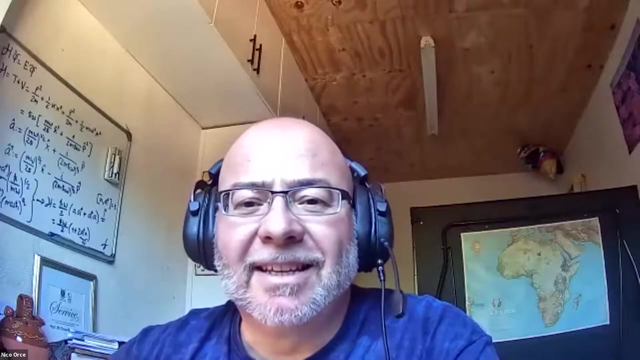 and write that level of steam, write the energies and see which ones are the same, which ones are different, and then assign yourself a spin quantum number to those levels. all right, any questions? manfred, you are very quiet. buku vuka vuka and danny jafta. any questions before we go? 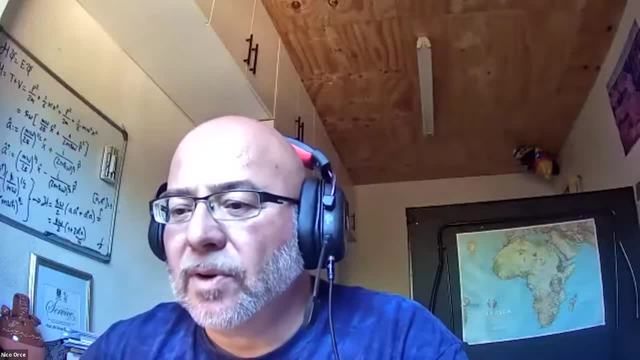 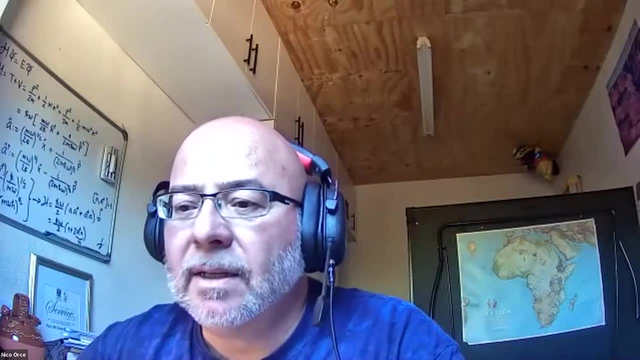 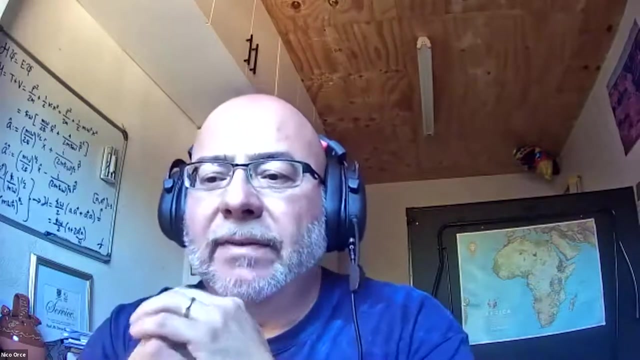 let me see what is in the chat. no questions from me, prof. uh, prof, sorry. what is the equal one? okay, now you know what is the equal one, jafta? yeah, that's where i'm getting lost. leads, leads after. are you okay now with the t equal one? 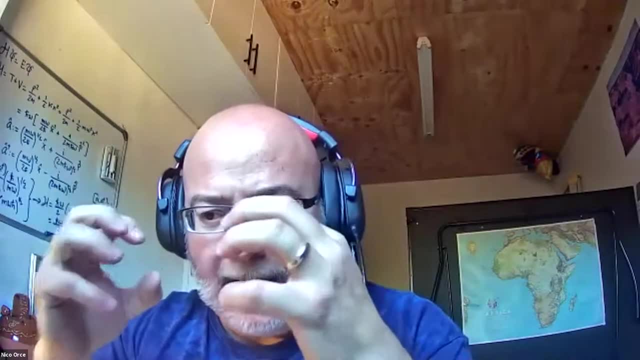 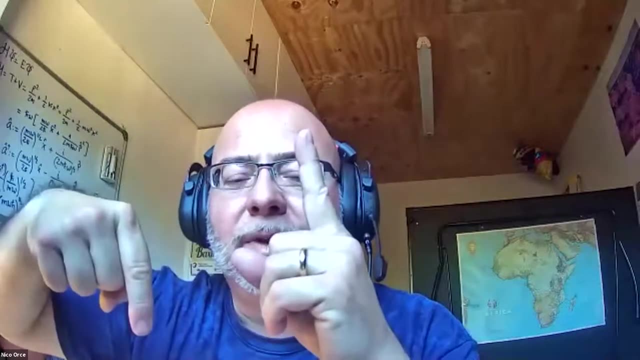 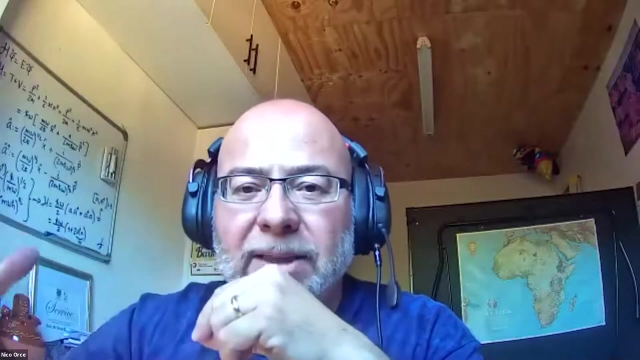 equal one means basically that s equal to zero s equal to zero means that the points, the spins, are pointing up and down. when the spins are pointing up and down, the total spin is zero. so to make an anti-symmetric wave function, which is how you describe fermions. 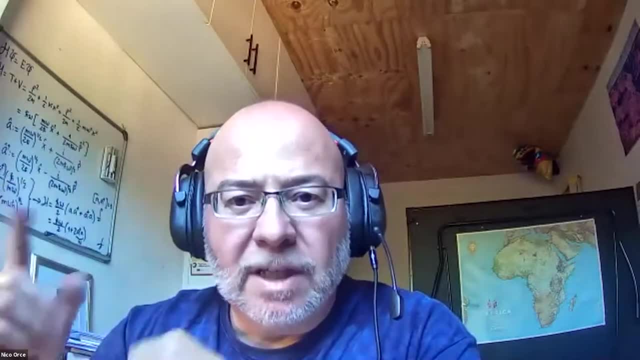 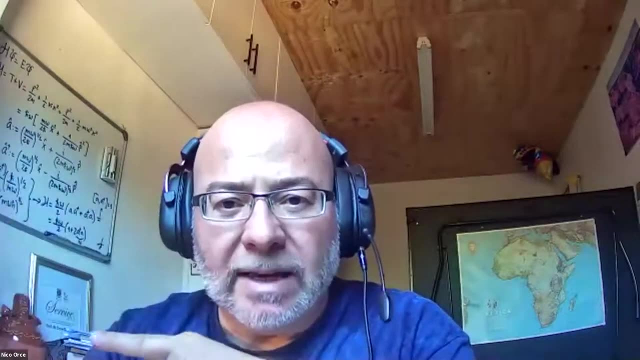 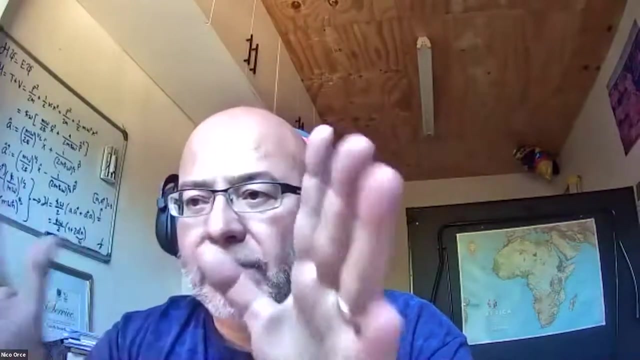 s equal to zero, t must be equal to one. the total wave function, the total uh you must have the product of the two, must be always an e or not number. if it's uneven, you have a symmetric wave function and you cannot describe fermions right. this is just basic quantum mechanics. 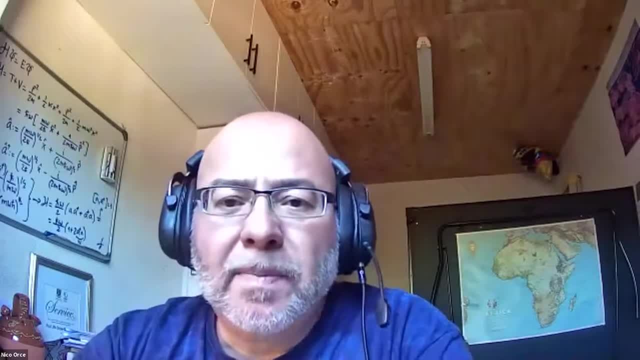 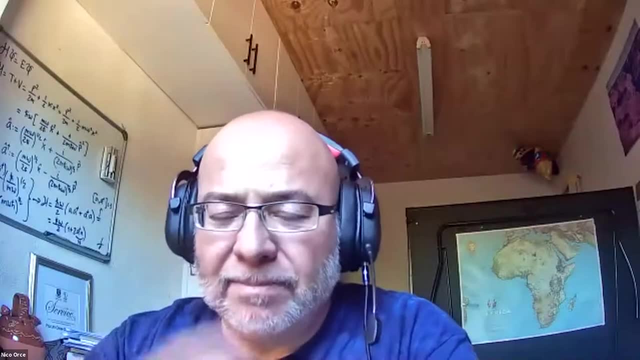 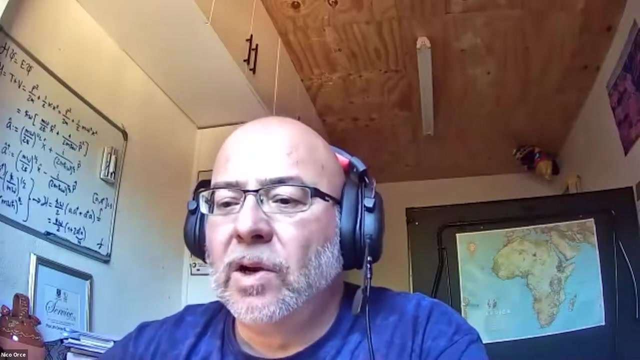 can you shoot it? tell me everything clear now. yeah, i think it's fine, sir. good, if, uh, if nothing, if something is comes unclear in the process, just send me an email. okay, all right, luasi, how are you doing? are you good? um, uh, one more thing is like, if you want to, 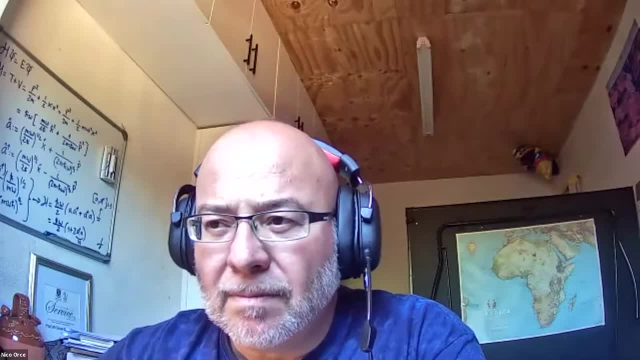 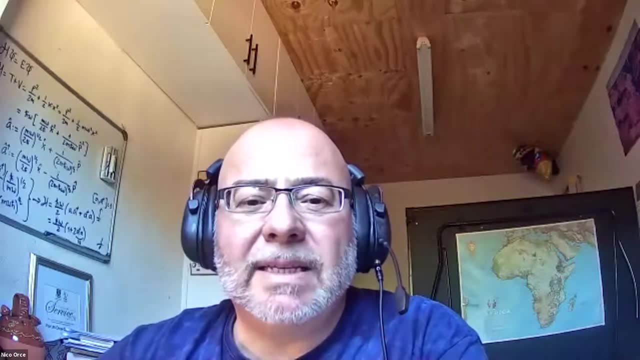 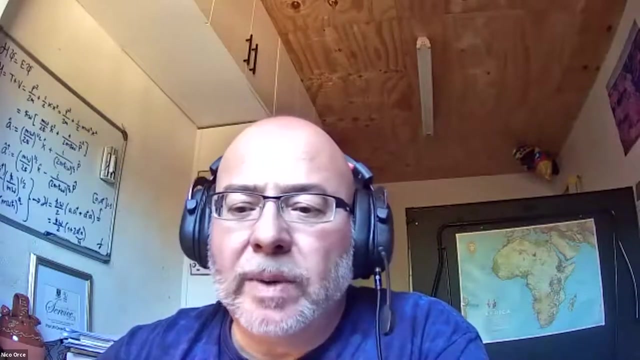 assign t. you use this formula: say: tz is equal to n minus z over two. i mean the number of protons. i i don't really do this, just, uh, a way to label each nucleus. there's a way to label this nucleus. it could be, you know, in. 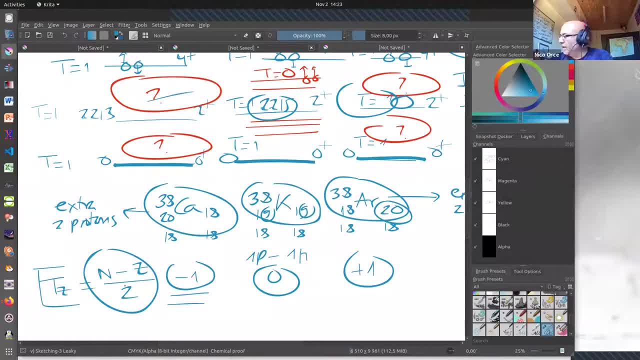 actually in particle physics they use the opposite formula. in particle physics they use t set equal z minus n divided by two. so this is just a nomenclature. i don't care about the whether tc is equal minus one, zero plus one, at this particular stage. i want to know: 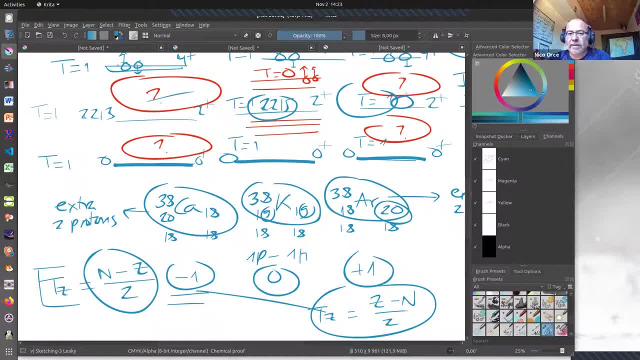 that when we look at the state this guy, we know that the two spins are pointing up and down, right, so i want you to label t, not this t set. this set is okay, you can also put it, but it's just a simple formula here. it's just: you know, 20, in this case neutrons, will be 18 minus 20 will be. 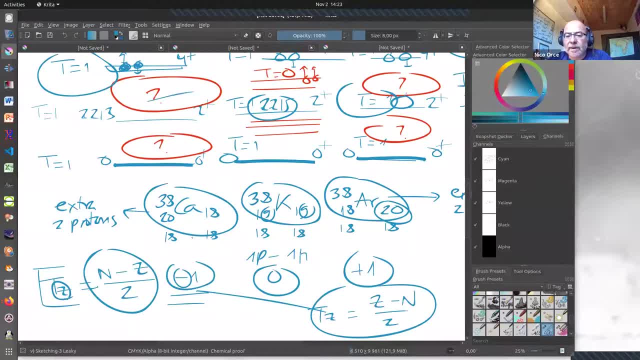 minus 2. divided by 2, this is minus 1. right, it's just a simple formula. but then really and really about is for you to label these guys: the t equal 1 s equals 0. t equal 1 s equals 0.. so you know that.